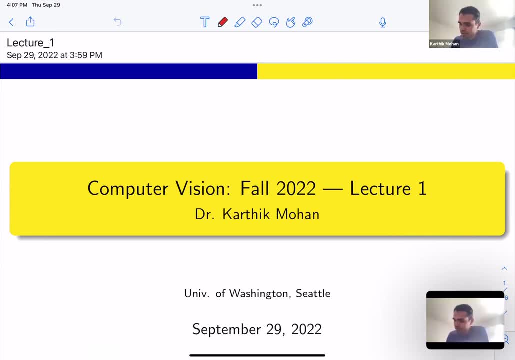 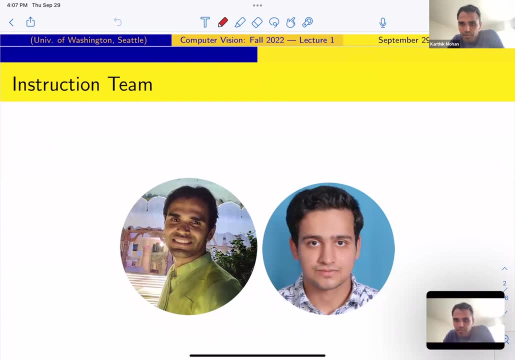 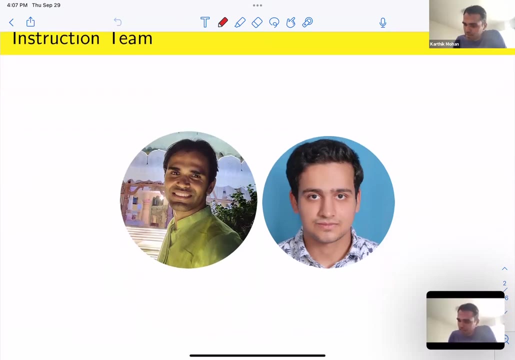 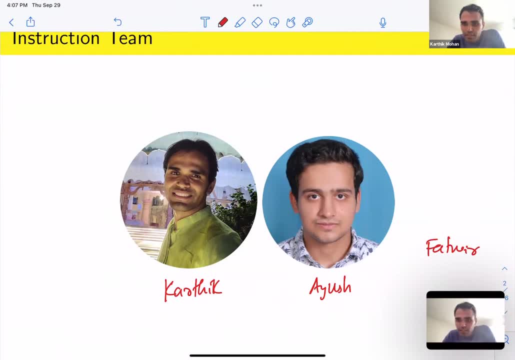 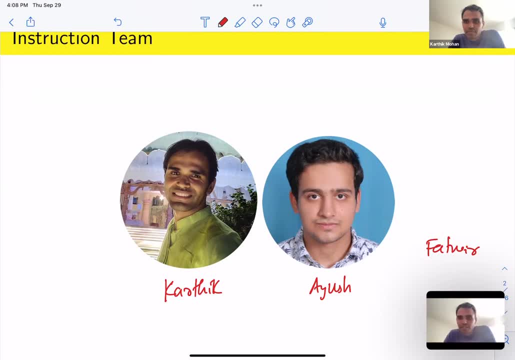 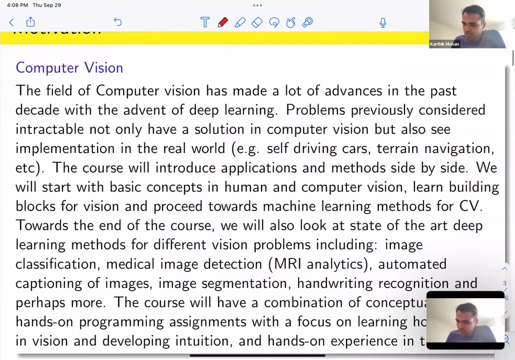 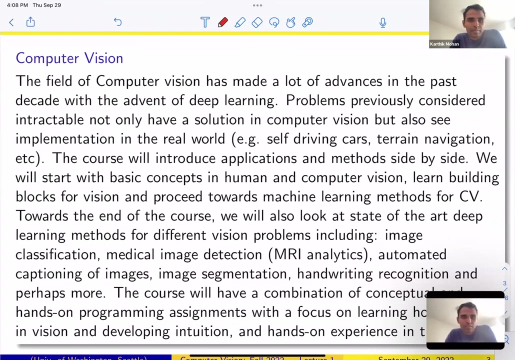 support with the grading. yeah, so we have a nice team going here for um, for uh, supporting you through the course. all right, so ta, and then greater right, okay, so uh. like we spoke about, uh, the motivation for computer vision is that, um, a lot of advances have been made in the past decade. 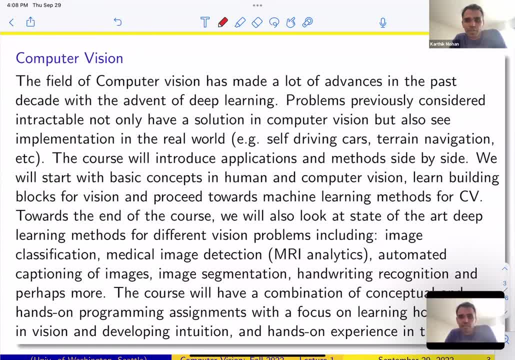 especially because of the advent of deep learning and computer vision, although has has been a old area where people have been looking at things for quite some time, understanding images better, understanding videos better, trying to solve problems in that space, doing object detection, image segmentation and things like that- but more recently, with the advent of deep learning, a lot. 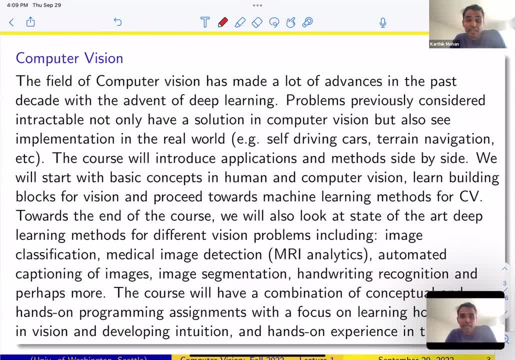 of things can be done more accurately and in real time because of, you know, computational power and advances in deep learning as well. so the combination of accuracy and real-time monitoring of images and videos enables things like self-driving cars or terrain navigation, or, if you have a drone going through an area, the drone is able to spot objects in real time. so all 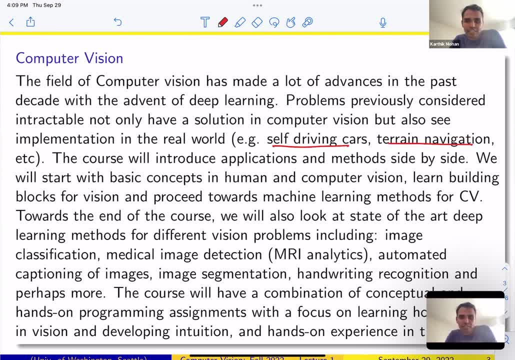 of that is a combination of advance in computing and also advance in computer vision, right, um, yeah, so we'll be looking at, uh, basic concepts in human and computer vision. uh, we'll understand some building blocks for vision and we'll also proceed towards machine learning methods for 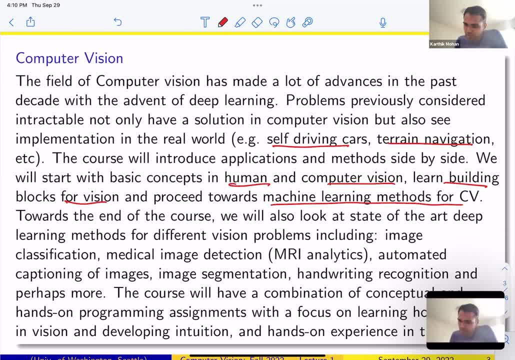 computer vision. right um, and hopefully by the end of the course we'll have looked at uh some state-of-the-art deep learning methods for different vision problems, um image classification, uh image detection, um automated captioning of images, uh image segmentation, uh handwriting recognition and maybe more. but again, 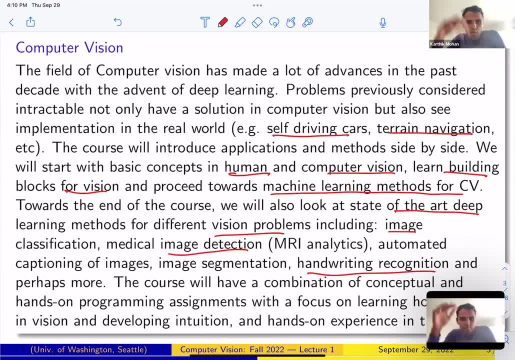 there is application of computer vision to these problem spaces, there is also really understanding how they work. so these are two different things. you can take a library and you can apply it to an application and say, oh, i applied it, but that may not mean you actually understood what what's. 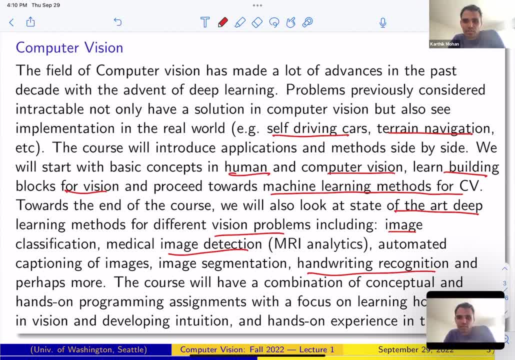 actually happening there, right? so this: in this course, we focus more on the understanding as well. without the understanding, if you, if you just apply a library somewhere and then you got some result and you're not able to explain why it's happening, then you'll not be able to, you know, make those. 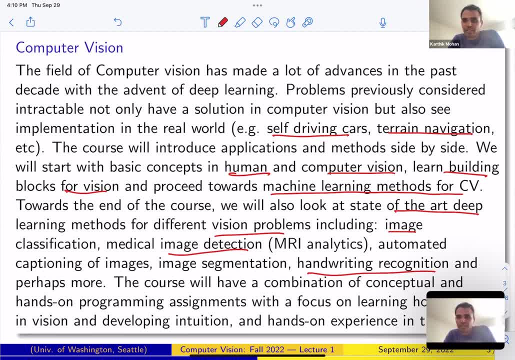 insights actionable. if you were to work at a company, for instance, you'll be asked to explain why this is happening or if you can change it, and you're like, i'm not sure. i just apply the library, so that's not going to work. so for that reason, we are actually going to also focus on some of 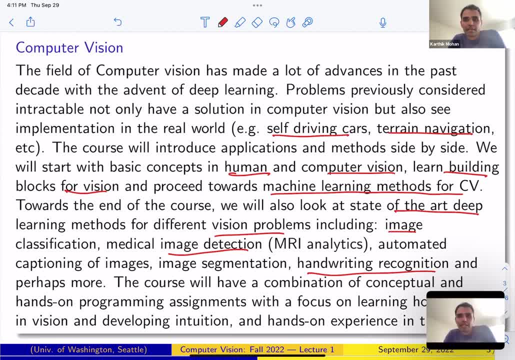 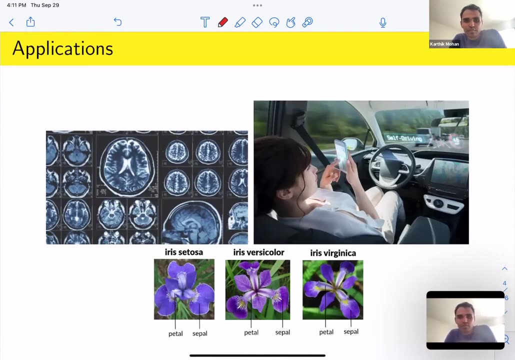 the fundamentals of computer vision and understand things better. yeah, does that sound good? so we will be having a balance between where you want to go, or i want to go here, versus where we can actually go, because we want to also get there with good intuition and good understanding. okay, um, all right, so let's let's look at some some of the cool stuff. 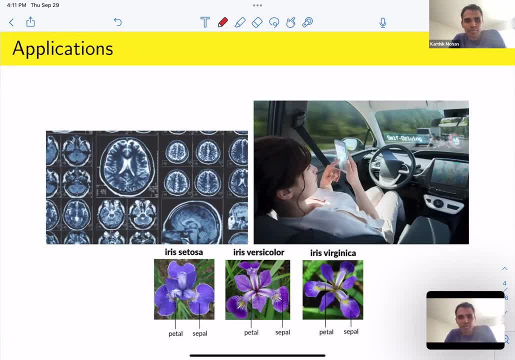 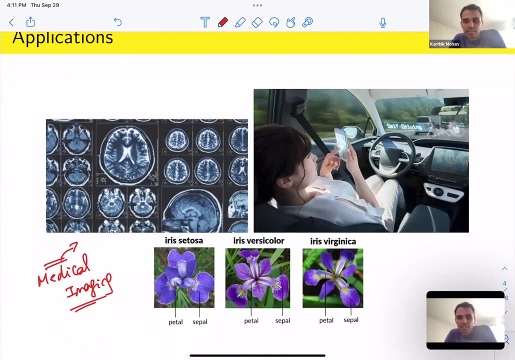 um. so there's a lot of applications of computer vision, as you know. so this is in the field of medical imaging. so i taught a course on ai and healthcare in spring quarter this year and we looked at some applications in um in healthcare. medical imaging is one instance. so here you see some mri images. 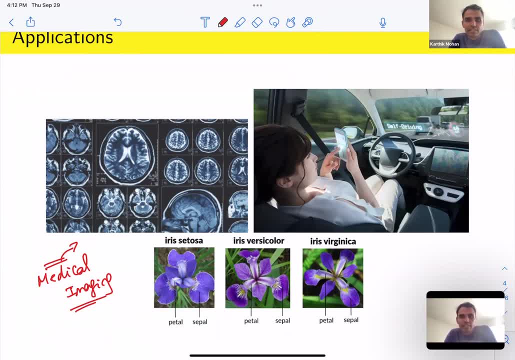 and then: are you able to detect a disease, or are you able to diagnose a disease or a defect based on these images automatically, or can you support a doctor in making a better decision? so there was a recent article i saw in the space where, uh, the article said that 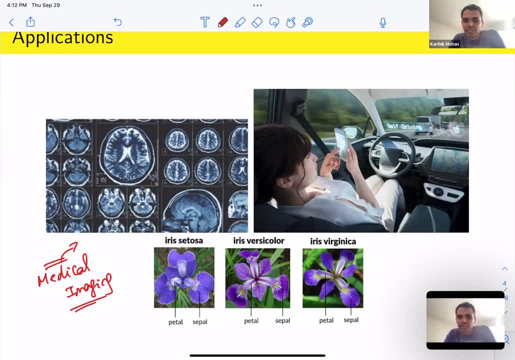 recent advances of you know medical imaging technologies. uh is helping doctors and, uh, you know imaging technology come together so they can do better if if they're standalone than if they understand alone. so, uh, the combination of you know socialatta and you know imaging technologies, i'm going to talk a little bit more about. you know the others, but also, of course, you know if you're already an embryo. it's the same thing. you know the newer embryos are different, right, and they're a different recipe and you can get or you know, and so they see the different applications and some of 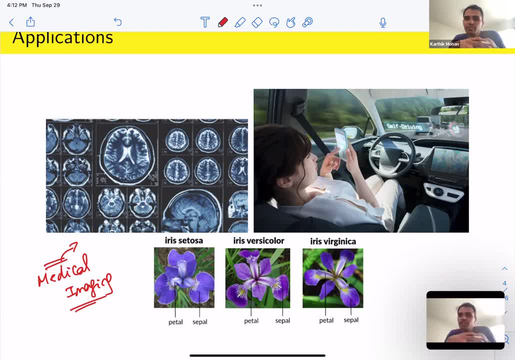 the other things, but i'm going to talk a little bit more about the history of the international, and a doctor looking at an automated system is better than just a doctor diagnosing the disease or the automated system diagnosing the disease. So there is a role for a combination of technology and 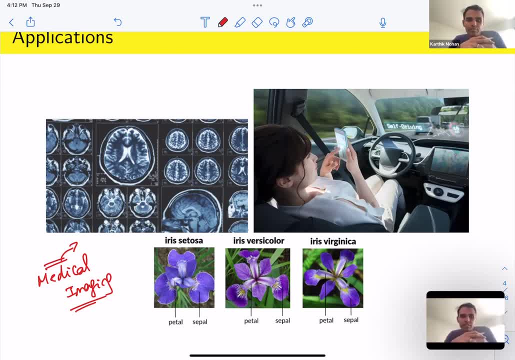 human in the loop, to work together to make better predictions in the case of healthcare, for instance. So that's medical imaging Also a very complex space because of the different levels of resolution, the zoom, the different technologies keep changing and there could be a lot of noise. 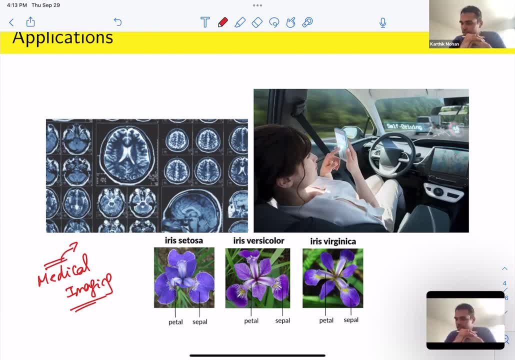 It's a pretty fascinating yet complex space. So that's one application: Self-driving cars- Anyone. Maybe just a show of hands if you've driven a Tesla, or you got a ride in Tesla, Okay, Or you've driven a smart car, let's say a smart car with autopilot feature. 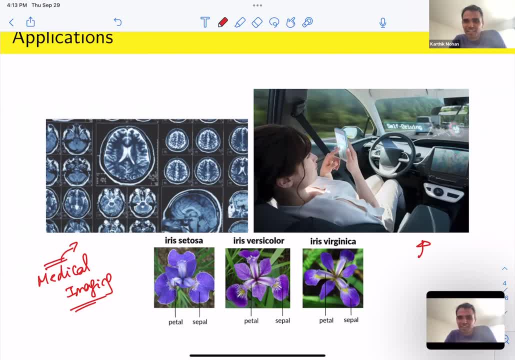 Okay, So self-driving cars, If you see, does anyone know how many cameras a Tesla has? Like eight, right, Yeah, Roughly around. I think there's. I think it's about eight. So I think there's about eight. 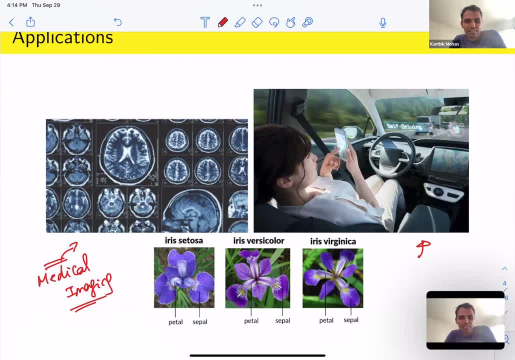 Okay, Okay, Okay. Two on the sides, one in the back and a couple in the front, So probably six, but I'm not. maybe eight, Yeah, But I was thinking six, but there's many. even six is a lot of cameras, right. So there's a lot of data coming in constantly. 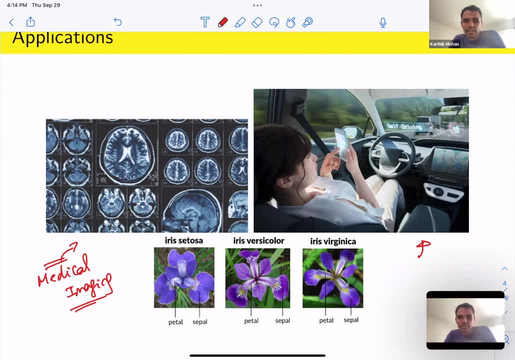 that's getting fed in through these cameras to understand what the surroundings look like for, let's say, Tesla or an automated self-driving car. And it's even. despite all of that data. you'll notice that if you've driven a Tesla, it still makes mistakes in low light conditions. 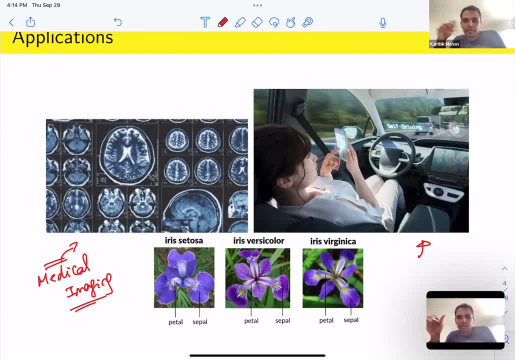 for instance, or you know, I was once driving on a highway- well, not a freeway, but maybe like a kind of 45 miles per hour speed limit road- And the white line was kind of blurred because there was some sand or something else, So it was not very clear and Tesla was not sticking to the lane. 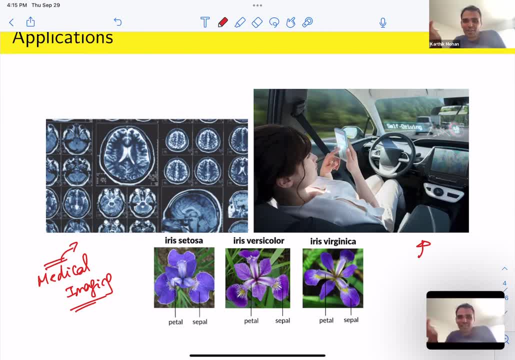 It was like kind of wandering off, when it would usually not do that So, but as a human I would not make that mistake. Yeah, So despite all the data that you can feed in real time and use the most you know best of the best computer vision technology, you can still make mistakes. 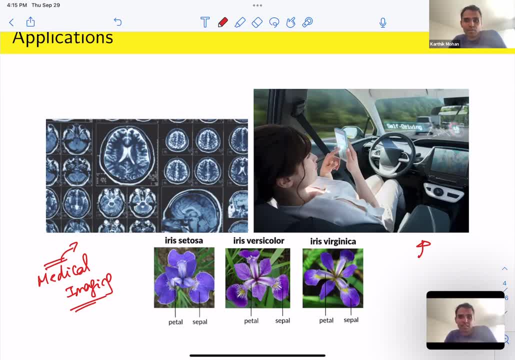 So that really helps you understand how amazing our human brain is. right, You know, we don't make such mistakes. We kind of are able to drive in many, many kinds of conditions. So self-driving cars is a very important application of computer vision. It obviously involves a lot, lot of tech. 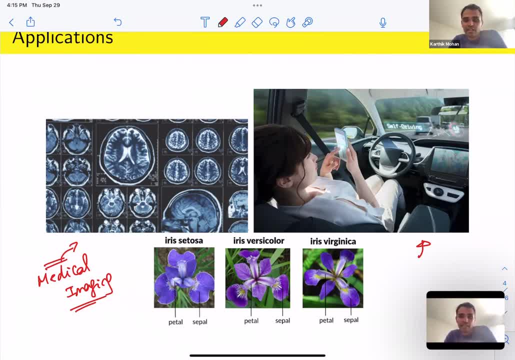 that's kind of put together to finally, you know, get there. It's a lot of moving pieces going on, but a key moving piece is computer vision. right, There's also batteries and other things, you know, that come in place, but so computer vision technology plays a key role there. 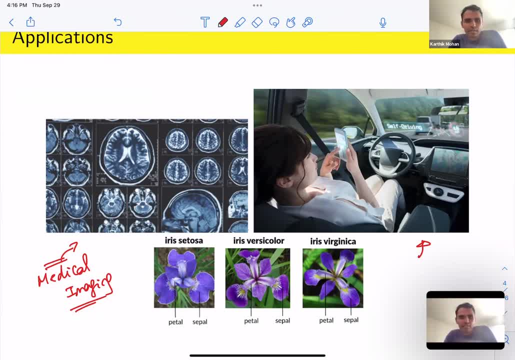 And we also have like standard image classification. So, given an image, can you classify it as a particular species of a flower. So we'll actually look at one of. well, this will be part of, probably, assignment two. So we'll kind of look at this data set where you have different subspecies of a given flower And 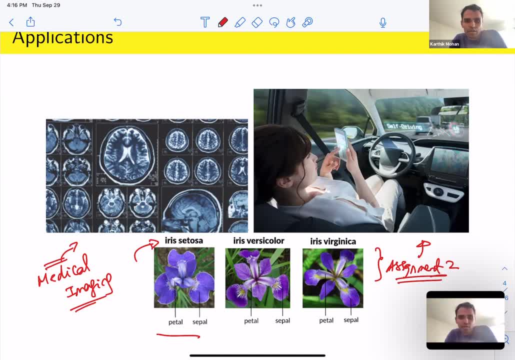 you can also look at the size of the set. what is the size of a flower? Can you classify it as like an iris? can you classify it as a particular species? Are you able to align yourself to that? or whether it's an ella or an isola, whether it's a common живот that is considered? 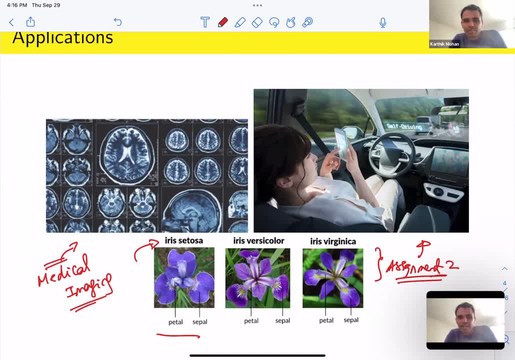 can you correctly classify it as, let's say, either setosa or iris versicolor, based on their characteristics? So this is a very classic application of computer vision, right, We'll also be looking at that, And I think there are apps these days as well, where you can just 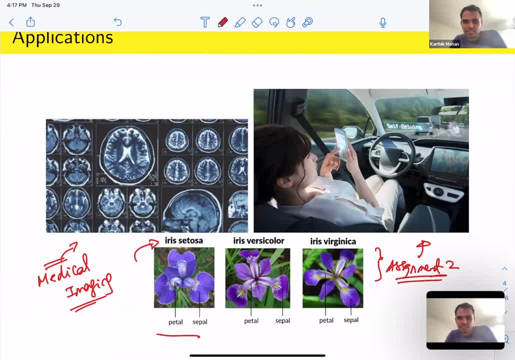 let's say there's an app for understanding a plant. You can just point your camera to a plant and it'll tell you what the plant is. Has anyone used such an app before? Yes, No, Yeah, So feel free to unmute and share. you know we'll keep it interactive. 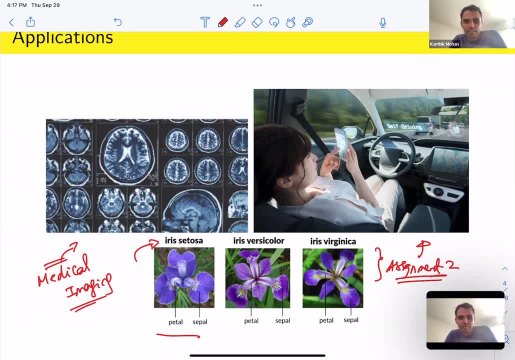 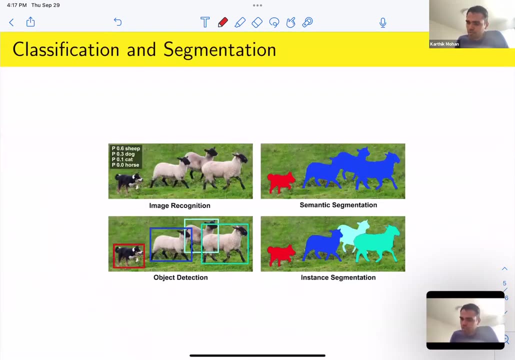 through the lecture. Um, so, if you have any thoughts, uh, just feel free to share and then we'll we'll keep discussing it. Um, so, yeah, that's another application: image classification, image understanding, Right, Um, going a little bit more into image understanding. 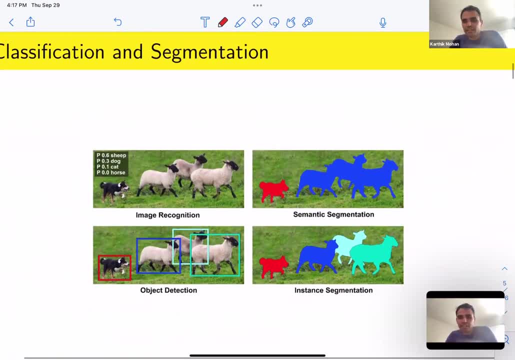 um, there's like different levels of understanding. that can happen with an image, right? You say, okay, do you understand an image? You're like, yeah, I understand the image. So then you say, what do you mean by understanding an image, Right, For instance? 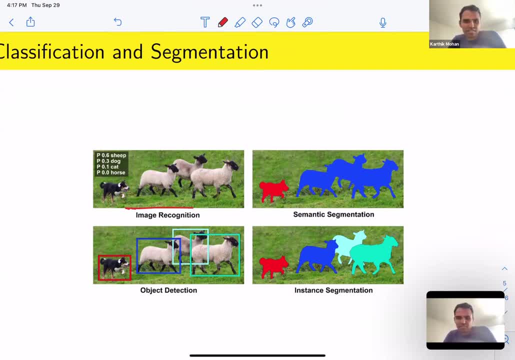 do you understand this image? You're like, yeah, I, I understand. there's a, there's some sheep and there is a dog. So what is so obvious to us? It's not so, not not so obvious to a machine. 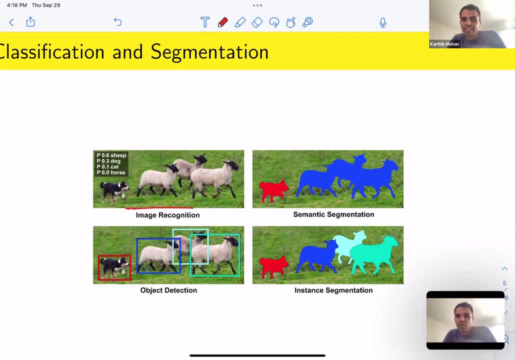 right, Like you can say there is some sheep, So you've already said there's more than one sheep, And you said there is a dog, So you said there's exactly one dog. So you you already know, just looking at the image, that there's like not just some, there's like three sheep and there's. 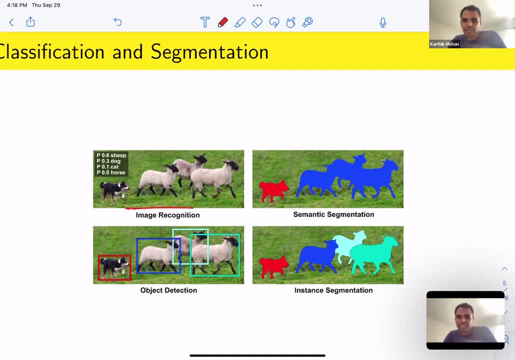 like one dog, So it's so obvious to you. but for a machine it might just say: I think there's a sheep in this image, or I think there's a dog, but may not be able to say how many. So that's. 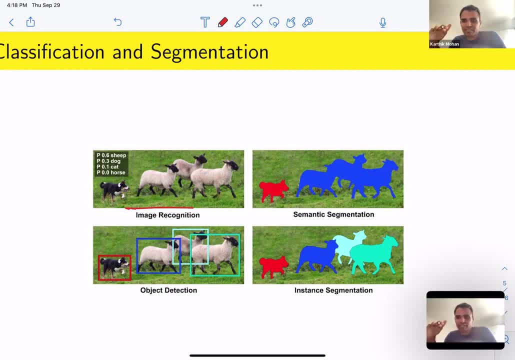 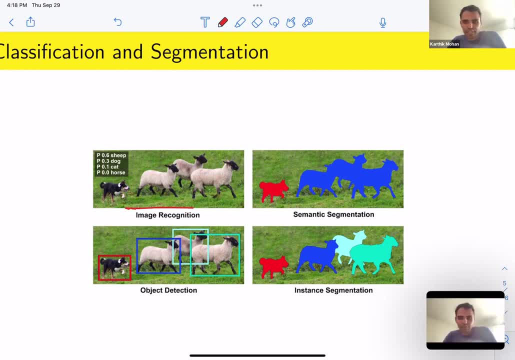 know You can also say multi class classification, multi-label classification, So you can put multiple labels to an image and say there's a dog, there's a sheep, but don't ask me how many. my algorithm thinks there's a sheep, but I don't know how many. Okay, So that's one level of 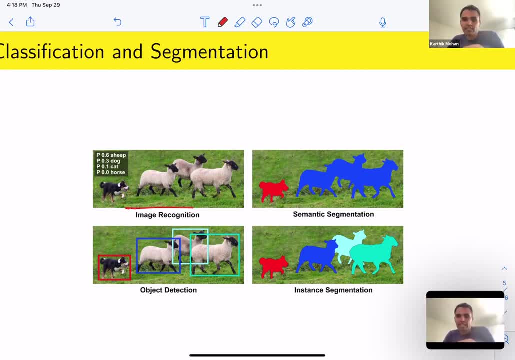 understanding, or even a even more basic level of understanding, is, I believe there is more of a sheep than a dog. So that's where this probably shows This is um multi class probability. If you think of it as a multi-class problem, you'd say I think there. 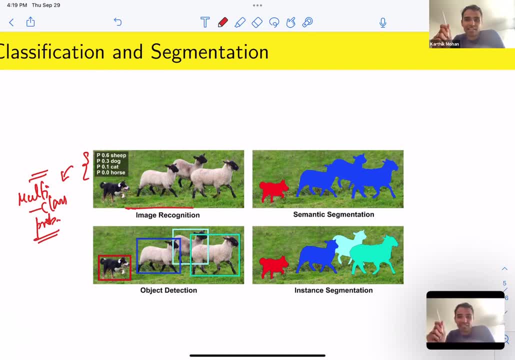 is multiple classes to pick from, but let me just pick one class, And the dominant class here, based on a probability, would be sheep, but multi-label would be like you know what? I think there's a sheep, but I think there's also a dog with a high probability. So that's a. that's a better modeling. 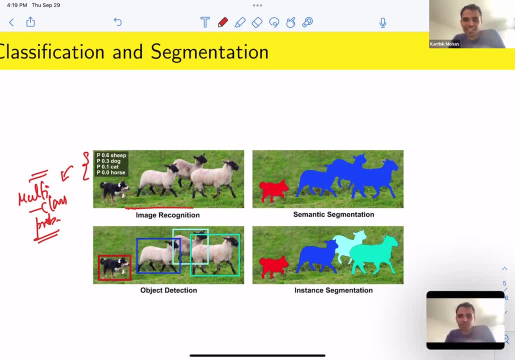 right, Because there's both a sheep and a dog. It's, it's true, Um, but that still doesn't tell you what else is going on in the image. Um, then comes object detection. You're able to actually put a bounding box around the objects in the image. So you say, oh, there is a dog, There's. 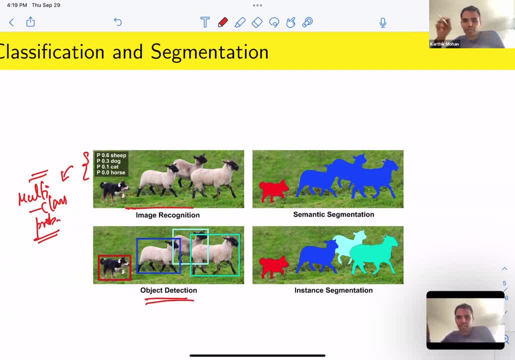 a sheep. Oh, there's another sheep And there's a third sheep, And you're able to pinpoint the rough location of these objects in the image. So the methods that do that fall under the category of object detection, right? Okay, So that's a better. 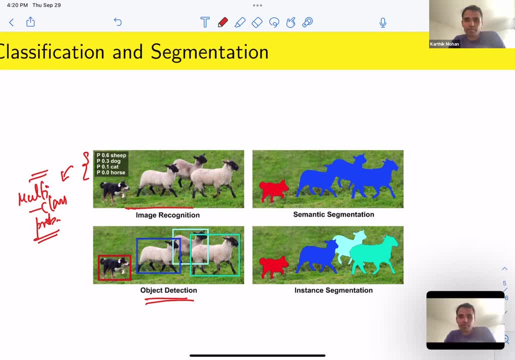 understanding of the image now, Um, I'm getting some messages here. Okay, So now, not only do I understand the image and I'm able to pinpoint the objects, I'm also able to pinpoint the location of the objects in the image. That's a higher or a better level of understanding, right? Uh then, 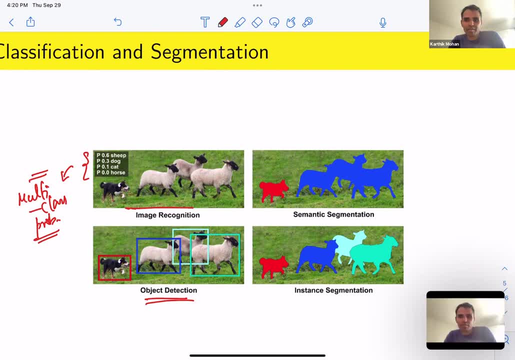 you say, you know what, can you just pull out the dog from the image, Just like pull it out, Like I just- I mean, even bounding box is probably not enough- Can you just pull it out. So that is segmentation, You kind of segment that part of that object from the image, kind of pull. 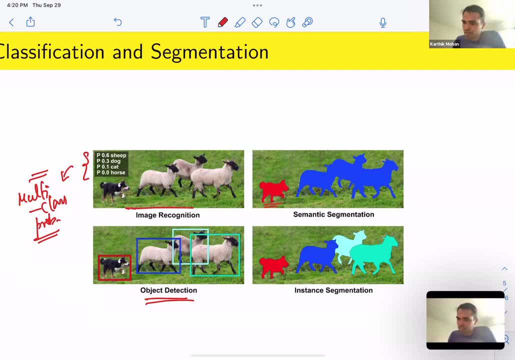 it out So you can see: okay, uh, the dog is clearly pulled out. Is the sheep pulled out here? Well, what's the plural? plural of sheep? uh, plural of sheep is sheep, right, So sheep is pulled out, but then it has multiple in them. So, uh, if you want to just pull out one sheep, 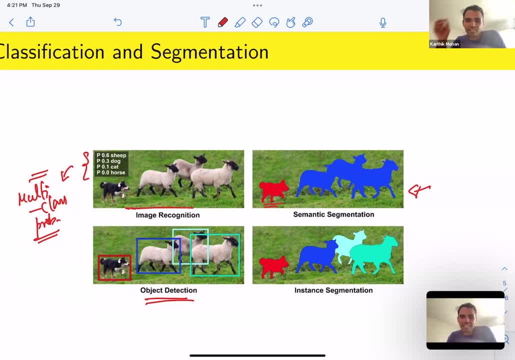 uh, that's not happening in semantic segmentation, So you need instant segmentation for it. So it's a refinement of segmentation where not only are you able to pull out a specific class of objects, you're able to pull out a particular instance of that particular class, Like if you've done: 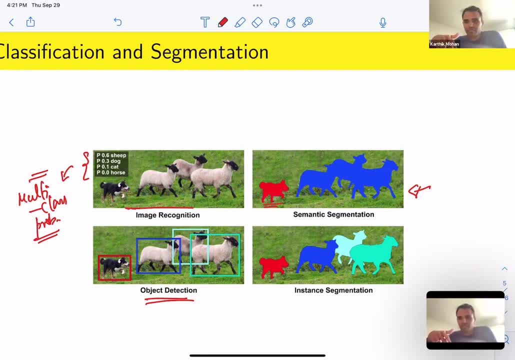 programming there is a class and then there's an instance of a class. right, There are two different things. Instance is an instantiation of a class, So the same thing here. uh, these three sheep belong to the sheep class. So if you say, pull out the class, 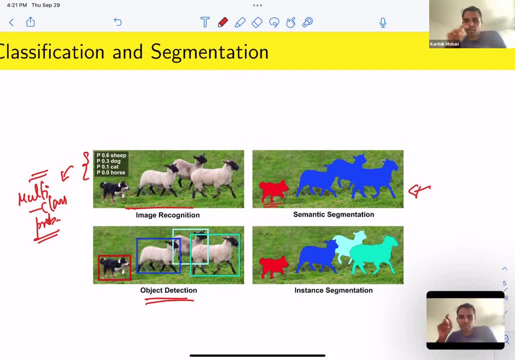 you'll just pull out the three sheep. But if you say, pull an instance of the sheep, you just pull out one of them. So that is instant segmentation, right? Um, so we'll look into uh segmentation as well in this class. So we're now just discussing the general uh right. 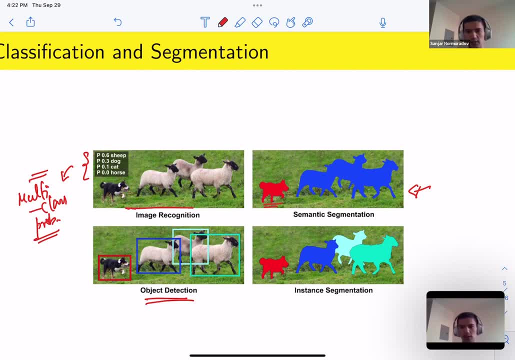 And we'll discuss more in details how we can realize instant segmentation from semantic. Yeah, yeah, yeah, We, we, we just, uh, we're just covering motivation today. Uh, each of these is like a separate lecture, or half a lecture at least, to go into how exactly we're going to do this. 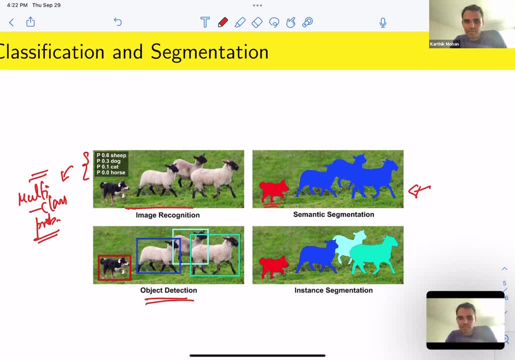 Yeah, Yeah, So we'll, we'll. we'll probably get to this and maybe week four or week five of this course. Uh, there's a lot of ground to cover, but I'm just motivating some applications that we'll be looking. 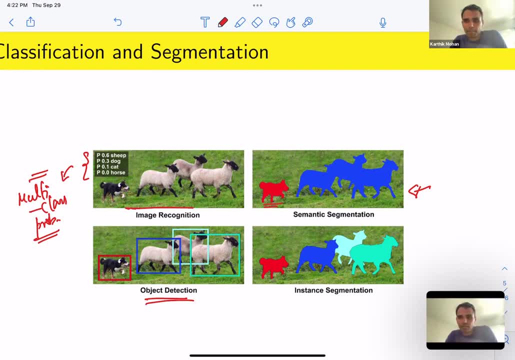 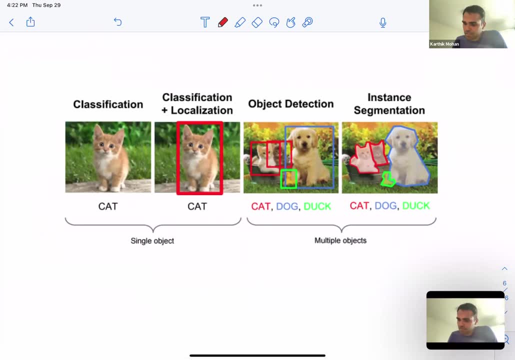 at uh in the coming weeks. Yeah, All right. Yeah, This is another example. So you know, you go from classifying a single object, let's say a cat, And then when you put a bounding box, you also call it localization. So it's not enough to classify, You want to localize it and say: 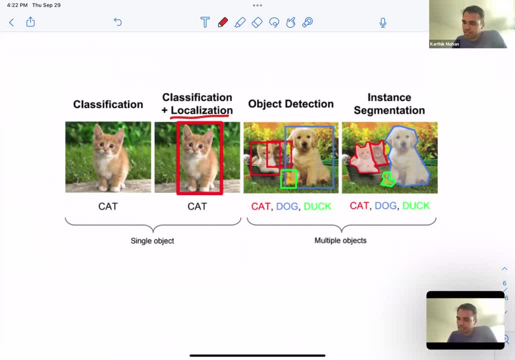 where exactly is it in the image? And then you have multiple objects, So it's not just a single object. So that's object detection, And then you're able to specifically pinpoint and segment these things. that is instance segmentation. So this is a more. 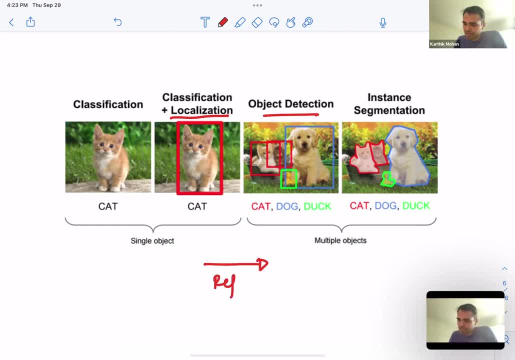 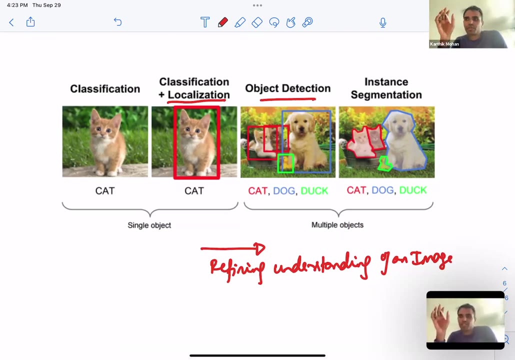 you know, as you go from left to right, you're refining your understanding um of an image. And then there's more, there's more and more. you can say So, when a human looks at an image, you can say so many. 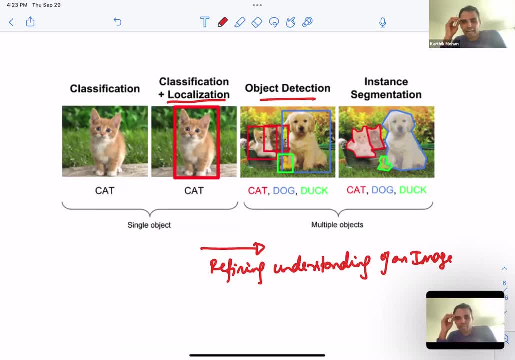 Things, uh, that a machine would find mind boggling. So we understand images so well. Um, you know vision is, you know the vision technology is getting there, but it's not. it's. it's not been easy. It's not been an easy ride to understand an image for a machine, Right. 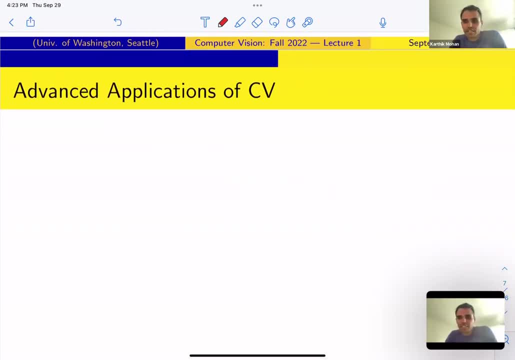 Uh. so let's look at some advanced applications of computer vision again as a motivation. we just to be very honest, we may or may not get to some of these advanced applications, because the background that's required to even implement any one of these advanced applications is like phenomenal. You need. 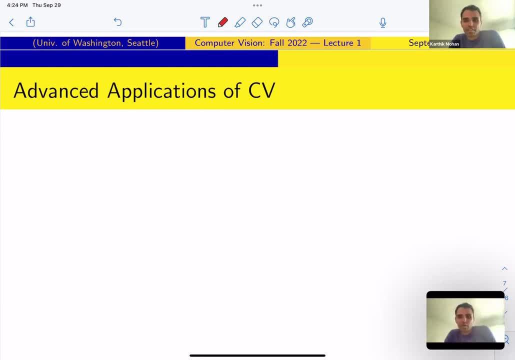 to have a deep understanding of deep learning, You need to know exactly what kind of architecture you're using. You need to be able to know how to train it and you know. you know, get a good algorithm going, good uh, evaluation metrics, And then, when you apply it, it seems to work. So you. 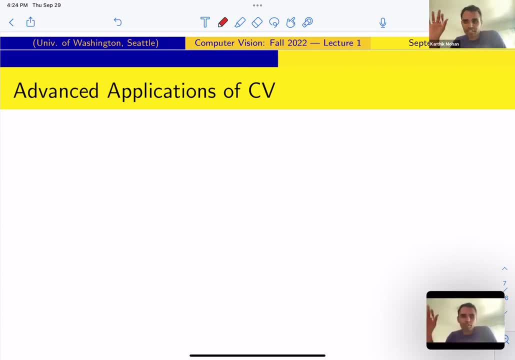 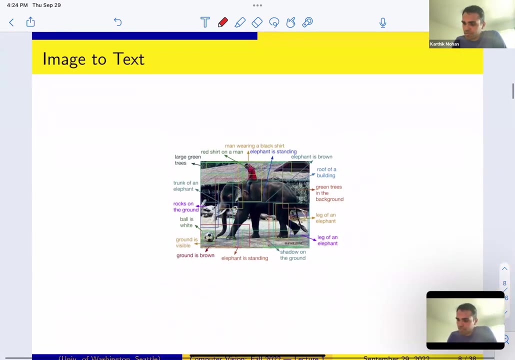 it could be a full project in itself. Each one of these applications could be a full project, Like you could spend like three, four weeks just like trying to get it right, But as a motivation it really is pretty exciting. So let's take a look at it. So, uh, you know we spoke about 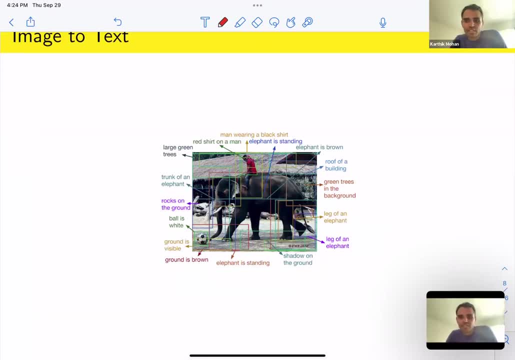 understanding images, right. So there's levels of understanding in images. So here's something more: not just pointing to what objects are present in the image, but point to it Like humans would do it. How would humans do it? We'd use language, right. 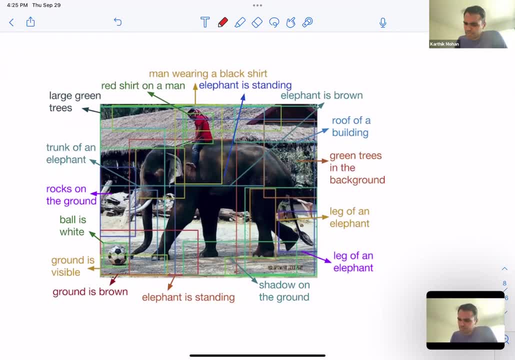 Let's say, okay, can you describe this image? You'd be like, um, I see an elephant, Okay, great. Then I see a man, Okay, I see a football. And then you can start having phrases like: okay, this is a Lego of an elephant. So you can, you can have a bounding box. You can just say: 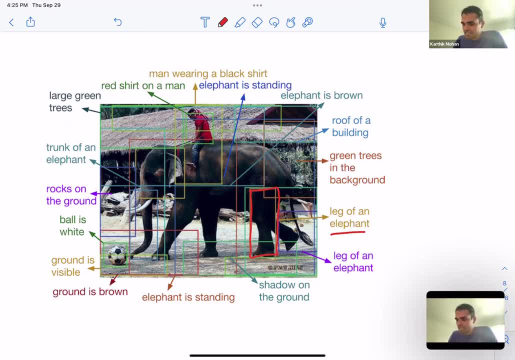 what is this? You'd say. oh, that's a Lego of an elephant. What is this? So it's almost like a kid looking at a scenery and saying: hey, mom, what's that? What's this, What's that? So even 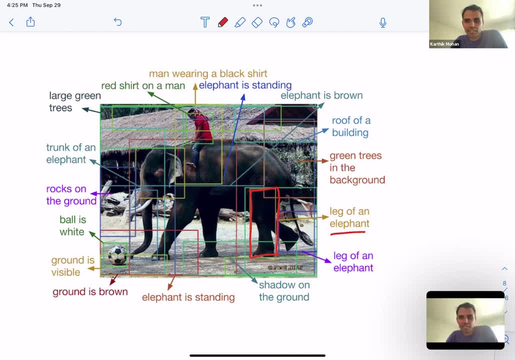 doing this accurately is amazing for a machine, right? Just pointing to different aspects of the image and understanding what's going on there through text. So you want to be able to use a sentence. So that's the next level of complexity or next level of understanding to just saying 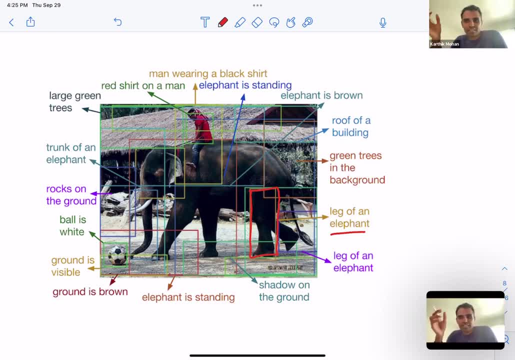 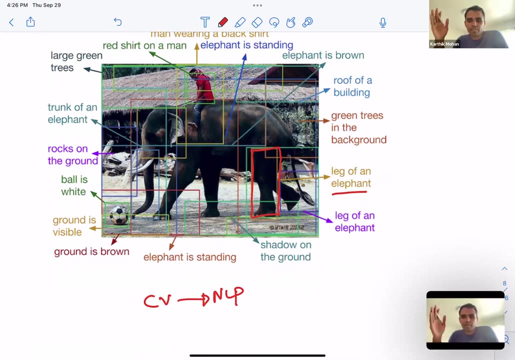 elephant just using a single word, because that's like a class. But when you are actually generating text, then we're getting into natural language processing right. So this is like CV to NLP. So until now maybe you were just in the domain of computer vision, But as soon as you 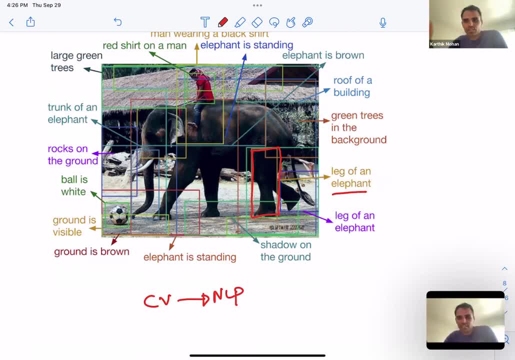 introduce more than one word that gets generated through a model that gets into natural language processing. So here maybe you are combining a computer vision model with a natural language processing model, So you're putting them together and then training them with some examples So you can actually generate these phrases or sentences. 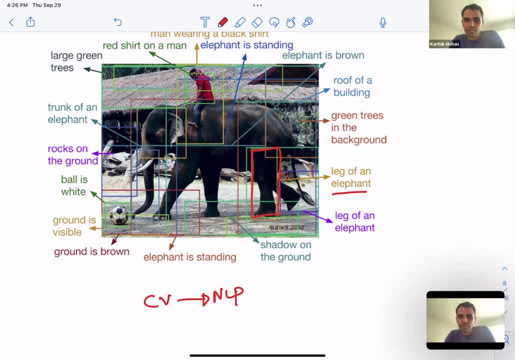 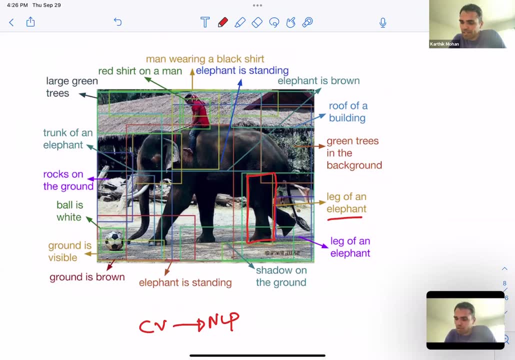 Right, So yeah, So you can see, this is okay. this is great. You can basically pinpoint to different parts of the image and you're able to say different things. That's great, But that's still not the same. So you can actually generate these phrases or sentences, So you can actually 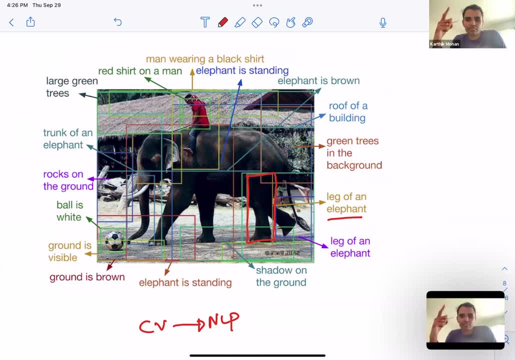 generate these phrases or sentences. So you can actually generate these phrases or sentences, So they're the same as captioning this image. If you had to just caption it using one sentence, what would you say? You'd say: oh, a man riding an elephant playing with a football. 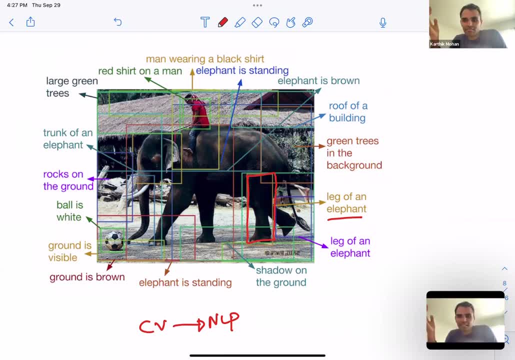 in a rural setting, right? Something like that. maybe isn't that complex. That seems simple, but it's actually very complex to be able to capture all the different things that are happening in the image and put it into a sentence, right? So that's great, Alright. So here let's try with the imagesek. a non-essential script saying in a specific way is somehow a sentence, and again, usingacional examplesso, he is the type of action that he takes when you like large format, aloud or other types of questions. Ok, So here. 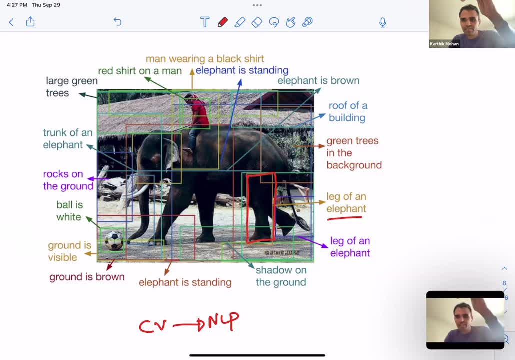 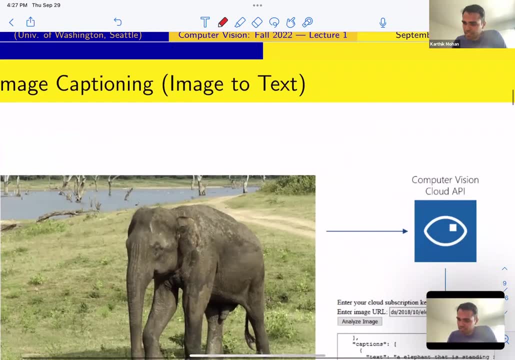 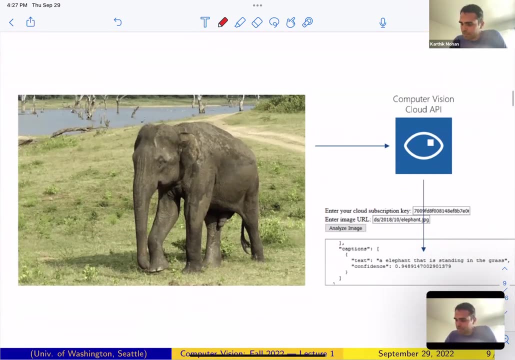 So that's called image captioning, a much more complex level of understanding of what's going on. So that's image to text. So here this is. I just found this example on the web where someone built a JavaScript product, JavaScript code, so that they can insert an image. 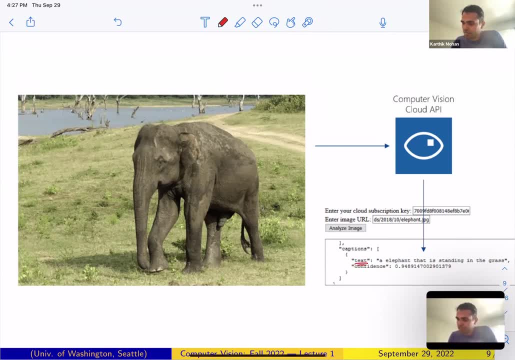 and it is able to generate text that's generated from Azure Cloud CV service. So the image goes to Azure and then Azure has a library that's able to caption an image and it generates it and then they put it here. So here the caption that was generated for this image. 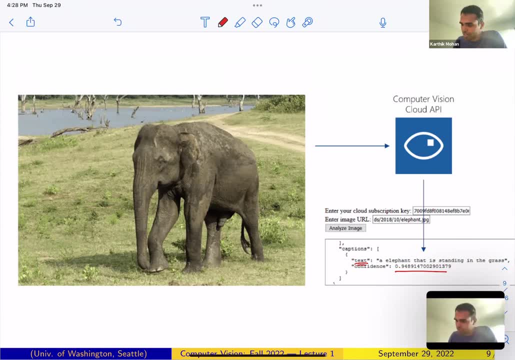 with this confidence or probability. like you can see, probability is not 0.95,. elephant that is standing in the grass. Okay, that's a very simple description, But this is image captioning, So you're able to give a caption to an image. 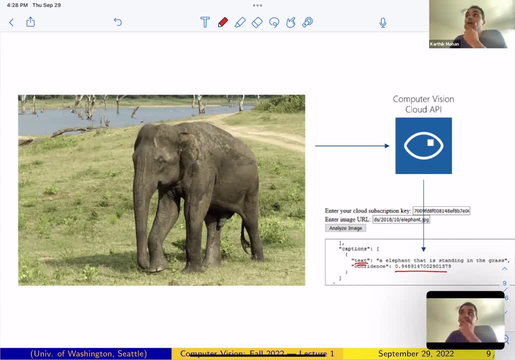 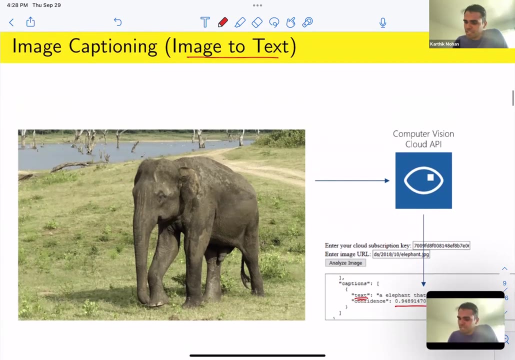 And I think there was a recent Kaggle contest on this as well with Google images, maybe like a couple of years back. It was pretty popular. It's available on Kaggle And there's a competition on that. So image captioning: image to text right. 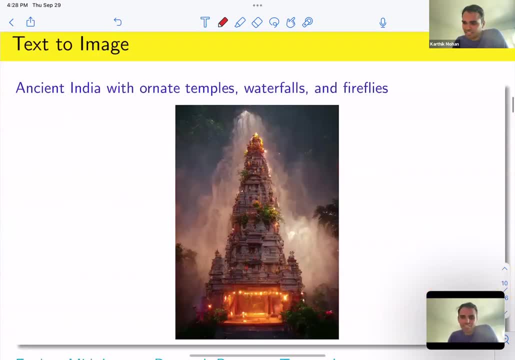 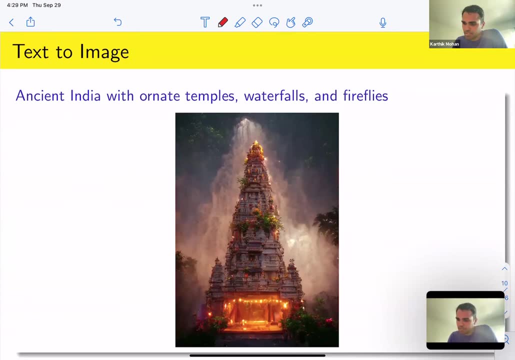 Here's something even more advanced and more recent. It's text to image, So this is a image of a temple. It's really, really amazing. Do you guys know where this is? Anyone know where this temple is located? Just take a guess. 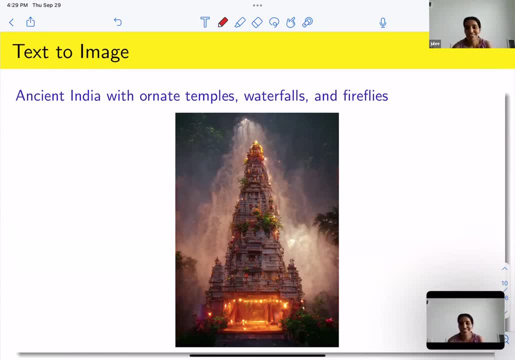 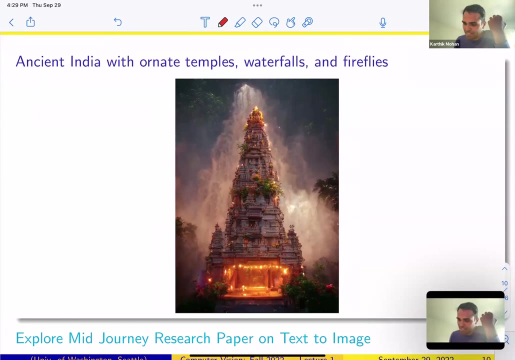 Somewhere in India. Somewhere in India? right? Yeah, Supposed to be, but this temple doesn't exist. It's generated by AI. It's completely generated by AI. There's no such temple, So this is generated to a web interface called MedJourney. 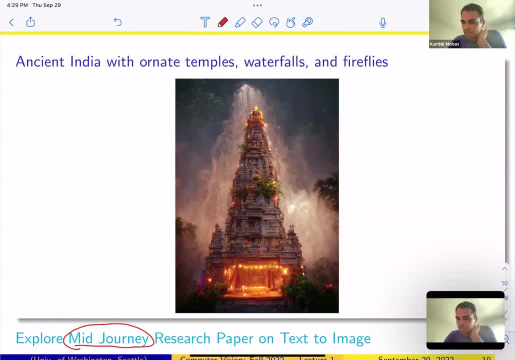 You can look it up. The link is provided in the PDF. So the person who generated this image through the AI, which uses computer vision, is basically typed something like ancient India with ornate temples, waterfalls and fireflies. So they gave some different keywords. 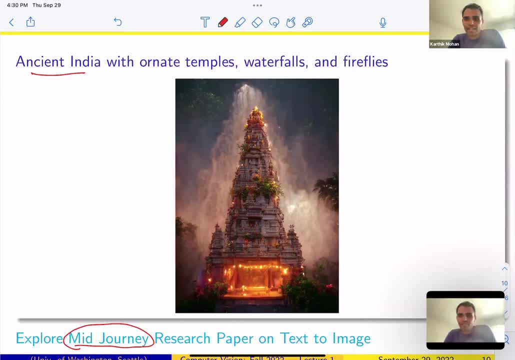 And that was the input, And there is a base set of images. You can see a very vast library of images that this AI depends on in generating photorealistic or artistic images that look really real. Of course, it looks like a fantasy, right. 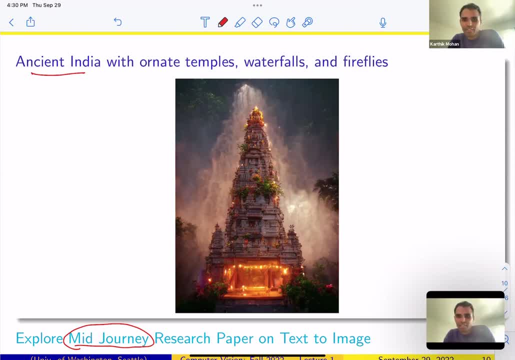 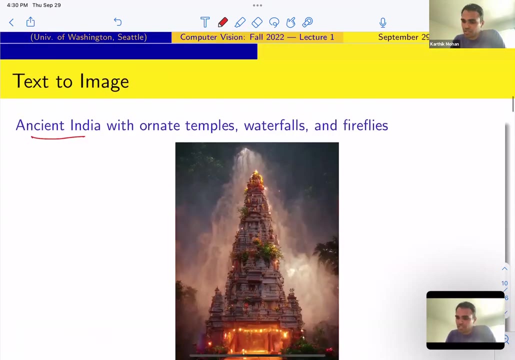 You can see there is some kind of a fantasy going on here, But it does also look real, right, But it's completely generated by an AI, So this is not real. So this is a very recent development, which is you reverse it. 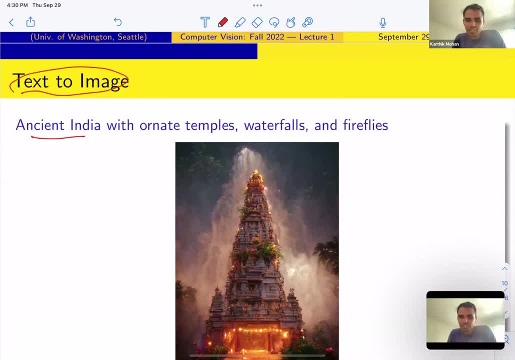 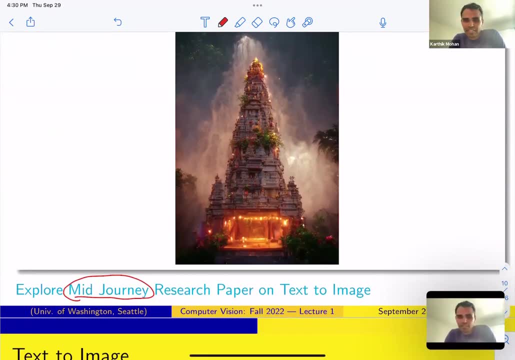 So, OK, image to text is complex enough, But text to image, that's crazy, right, But it's happening And I think we'll have this as part of assignment one. OK, So this is just go generate an image of your choice. 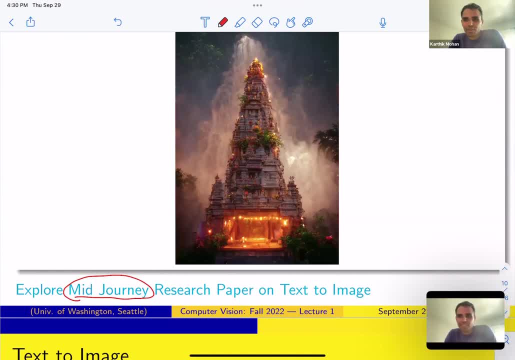 using your favorite text And maybe we'll post it in your assignment, but also on Discord, where, hopefully, is everyone Discord. Yeah, You must have got an email with invitation for Discord, So do join Discord. All our communication going forward will be in Discord. 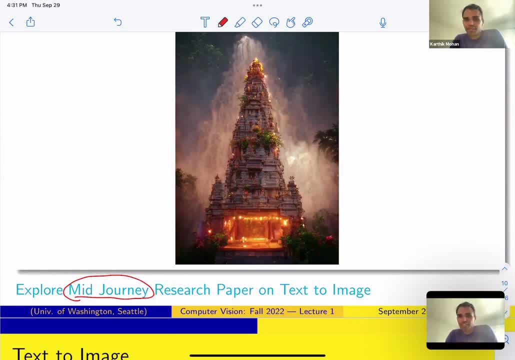 So, yeah, part of your assignment one will be to just generate an image of your choice. It could be anything crazy, but post it on Discord And hopefully you get excited about it. This is another example. Again, it's not real. 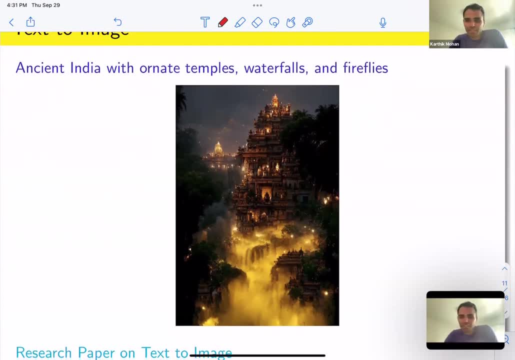 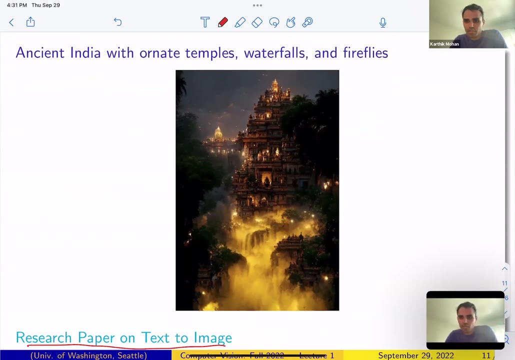 There is no such image. Maybe it could be real. It'll be great if it was real, But this is again generated by an AI, So really fascinating. There's also a research paper that I've linked here You can take a look on how they do these text-to-image models. 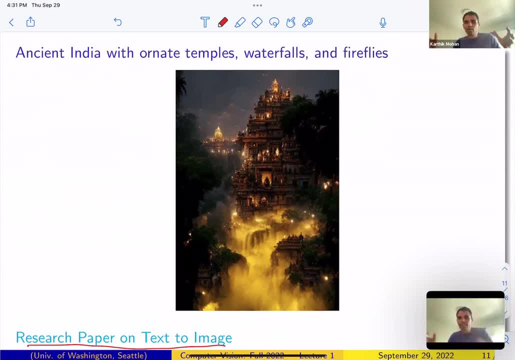 Pretty complicated, But again it's a lot of building blocks. You start with the alphabet A, B, C, D, And then you say let's create words, And then you take words, you create sentences, And then you take sentences, create paragraphs. 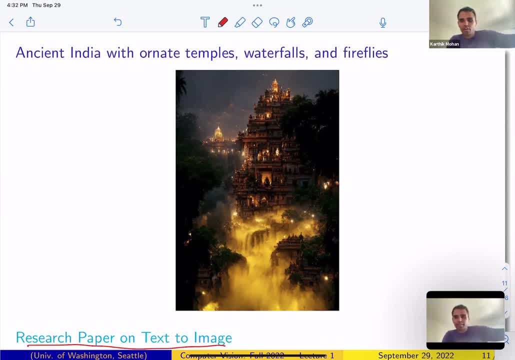 And then you take paragraphs, create a document. So if you say, how did you create a document, You had to go all the way to the alphabet. So the same thing here: How do you generate an image from text? Well, there's a lot of building blocks. 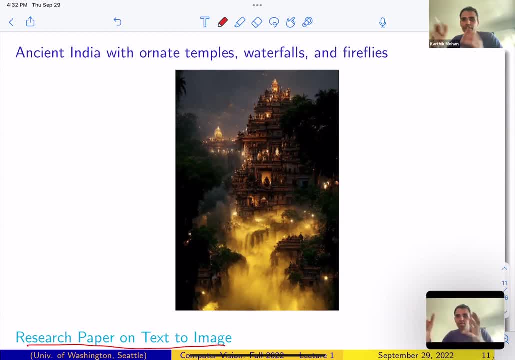 But those building blocks are present. It just has to be put together in the right way And you're able to get here. I think I'm getting some messages here once again. Let's see if my Discord is open, OK, I'll close it. 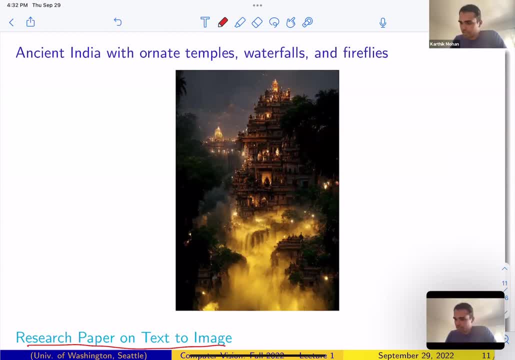 OK, All right. So yeah, Feel free to generate your favorite kind of image using mid-journey, And that'll be part of your first assignment. just as a way to understand the capabilities of computer vision, You can just take a look at it for yourself. 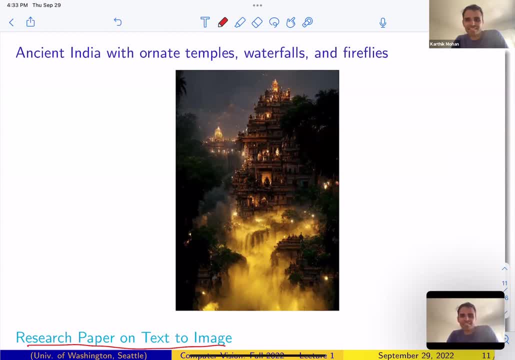 Whether we'll get to really understanding how it is done in this course we'll see, because we have to cover a lot of material before that. But it could be something that you can aspire to understand at some point And we'll see how it's exactly done. 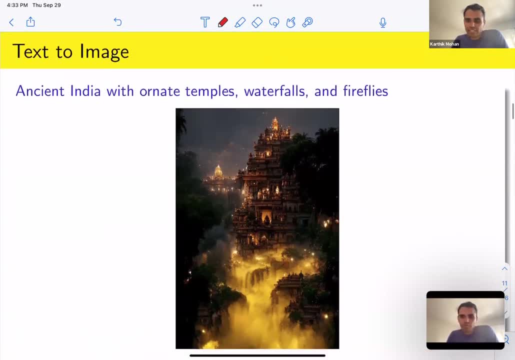 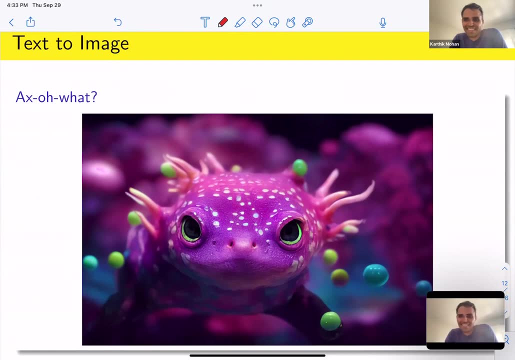 Yeah, Building on top of this. OK, There's one more. OK, Anyone know what this is? Salamander, No, Salamander, Yeah. Who said that? Sanjay, Yeah, me, Yeah. So this is actually based on a salamander. 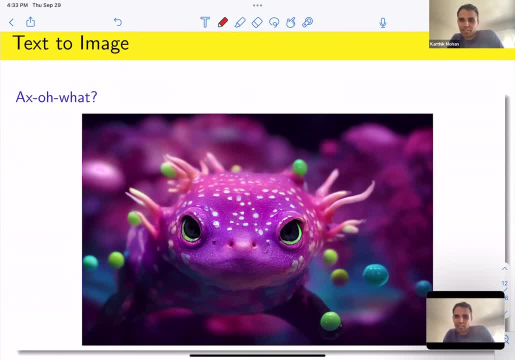 although it's not real. again, This kind of a type, OK, This type of shape and everything is not real, But it's based on a salamander that's actually real. So let's look at what the real one is. 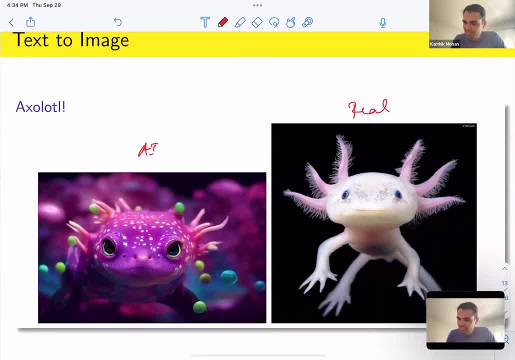 This is a real one. This is AI, So the right one is actually real, But the left one is based off that and it's not real. So you might see something like this in, like a Pixar movie or a Disney movie or something right. 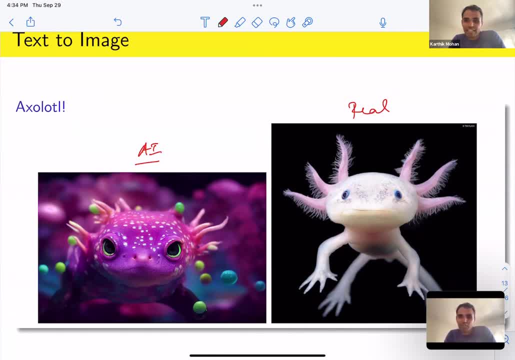 The one on the left, But the one on the right is real. It's a type of salamander that refused to grow up. So it has all these amphibian kind of goes through different stages. It kind of refused to grow up. 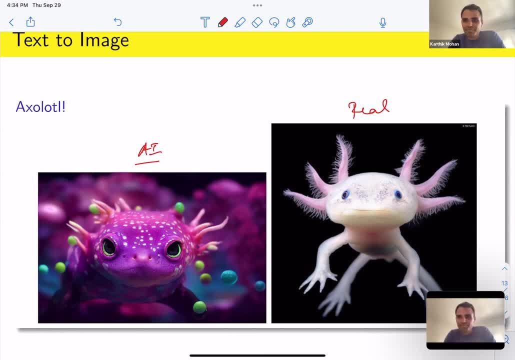 So it still has all these other things sticking out, So it's called axolotl. So this salamander is called axolotl. So someone actually generated this in Midjourney based on axolotl images and kind of added. 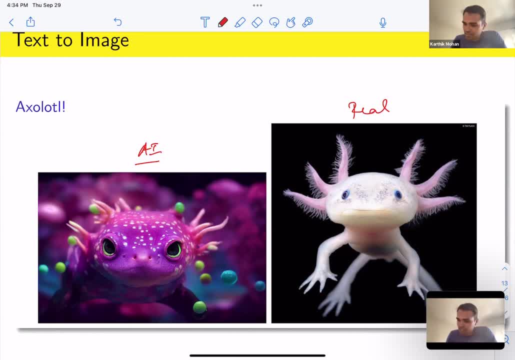 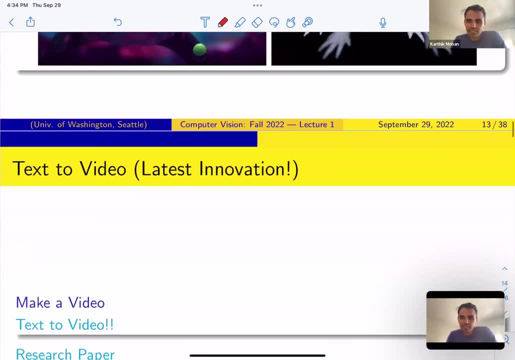 some different kinds of color and everything. So what do you see here? So text-to-image: OK. next level, which is very, very recent. I think I just saw posting on this a couple of days back. Text-to-video: take a text piece of sentence: 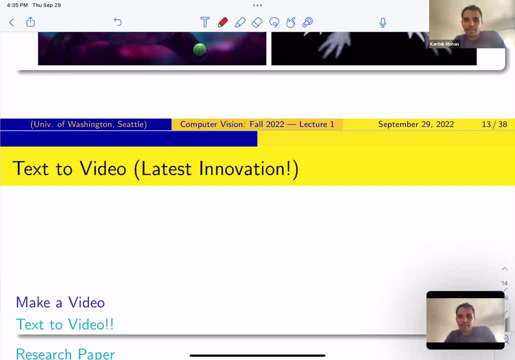 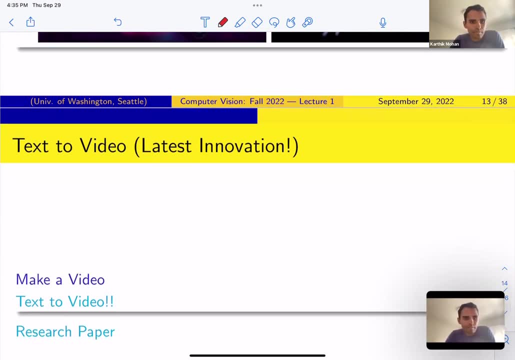 and then generate a whole video, Or maybe generate a TikTok-style video. right, Let's see if we can. I'm just going to. yeah, maybe it'll be worth playing some of this. Pause the video here, OK, great. 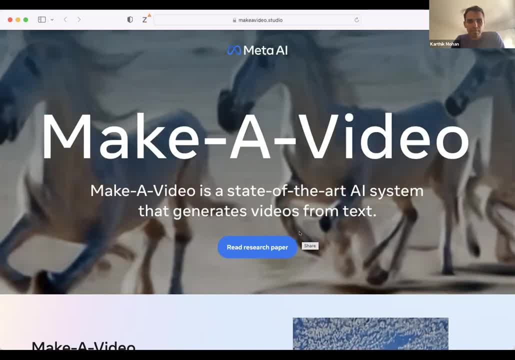 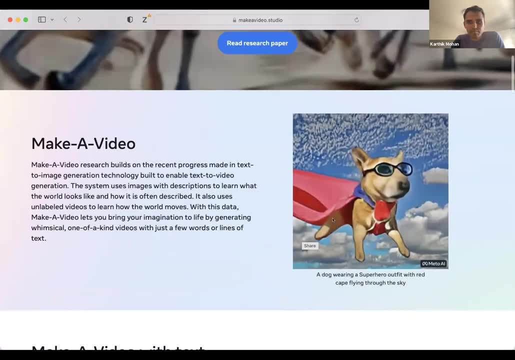 All right. so this is called Make a Video. It's a state-of-the-art AI system that generates videos from text. So there's a paper on this. You can take a look at it here. Of course, it's not super realistic. 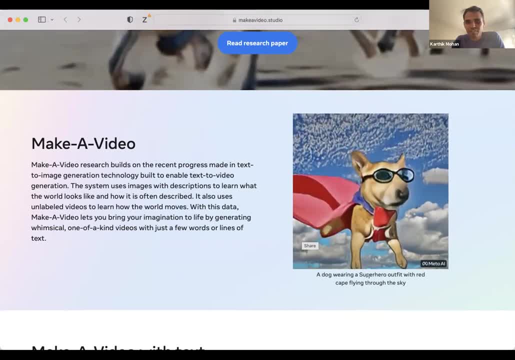 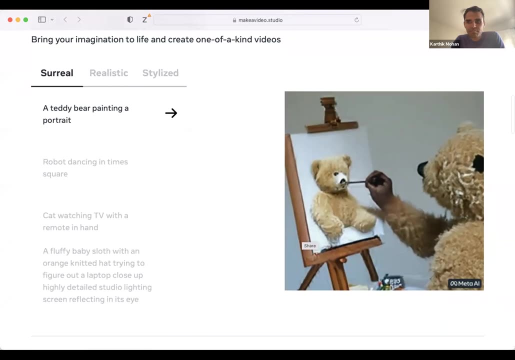 But this is a video, For example, a dog wearing a superhero outfit, with red cape, flying through the sky. So you type this text and then you get a video that looks like this, completely generated without any other inputs. Here's another example. 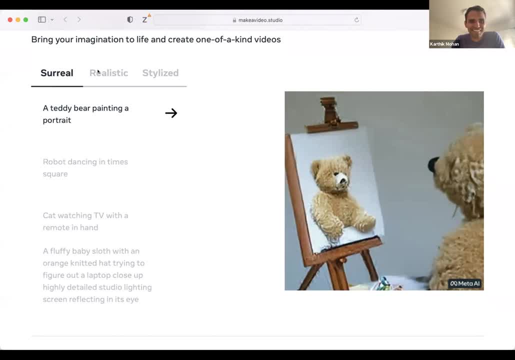 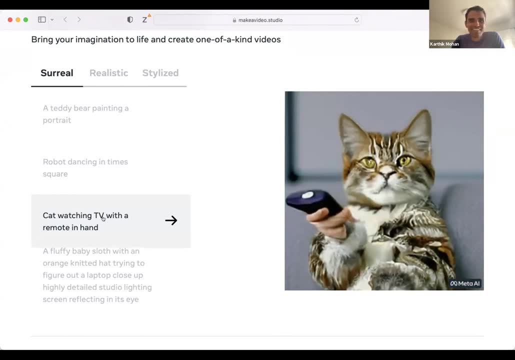 A teddy bear painting a portrait- This is other examples- A cat watching TV with a remote in hand. So things that you could probably never see in real life but you could imagine happening is something that you can generate through this, But obviously there's some low resolution going on here. 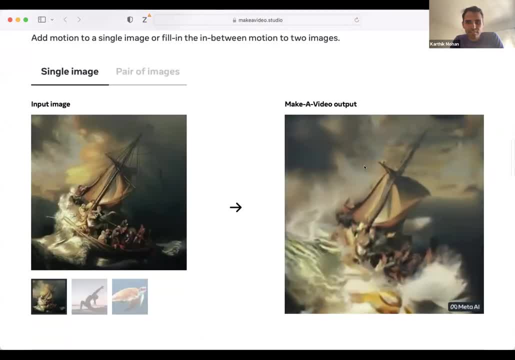 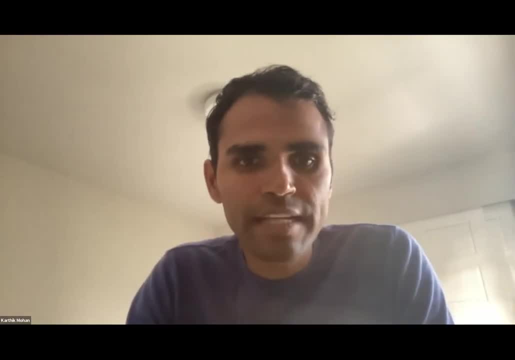 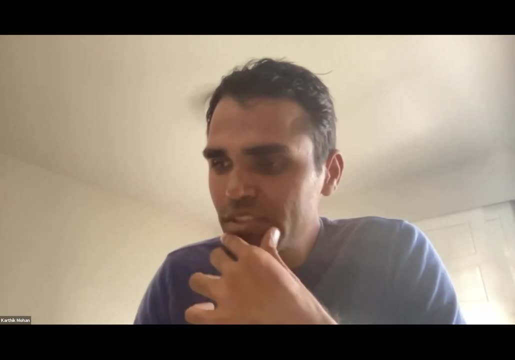 some warping of stuff, But it's like a start, So feel free to explore this as well. Put a link in the slides- The slides, by the way, I've shared on email. OK, But once the website is in a good place. 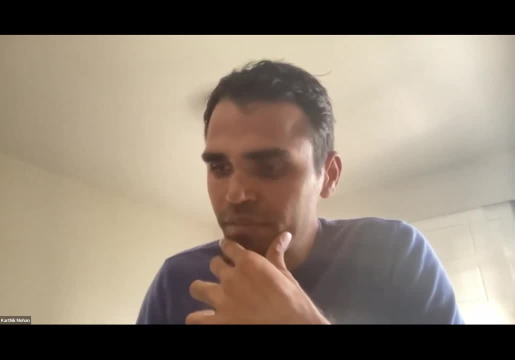 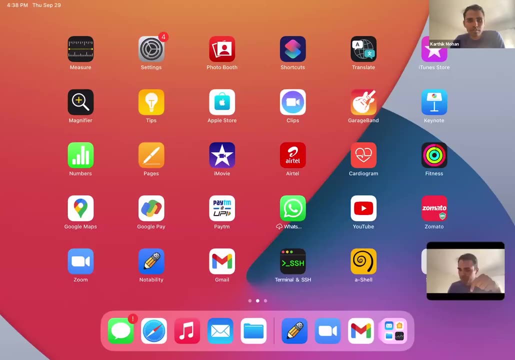 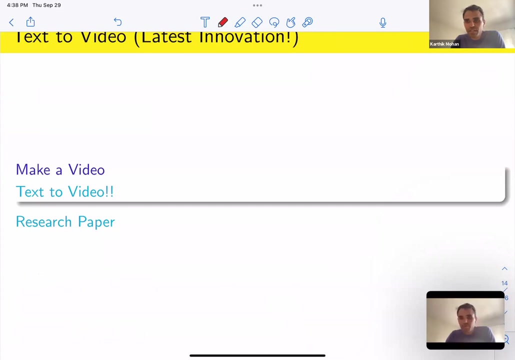 we'll also put it on the website So you can access the slides for the lecture before the lecture starts. OK, All right, So that's Text2Video And there's a research paper on it. Feel free to take a look at it. 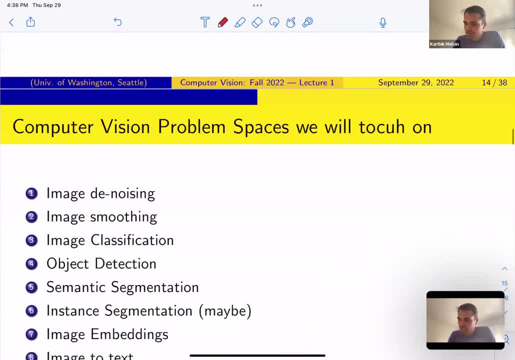 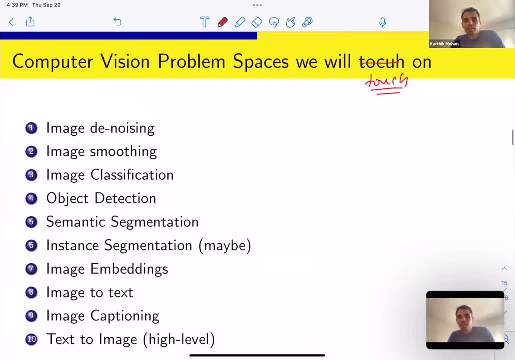 And if you have any questions, feel free to put them in the chat box And we'll get to them in just a few minutes. But, yeah, all right. so some computer vision spaces we'll actually get to touch on in this lecture. 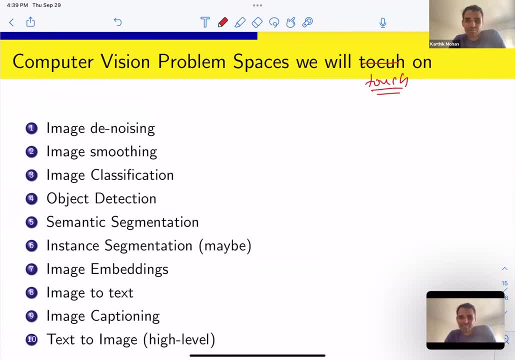 So that was motivation, right. So we may not be covering Text2Video, We may not get to Text2Image as well, just because of the complexity of the models. So when I mean get to, it means actually implementing the model. 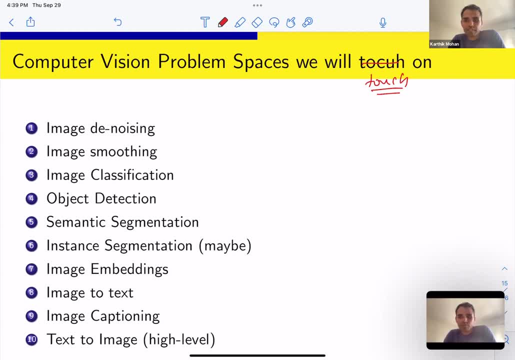 and understanding it, But feel free to explore it on your own, Like. these are all available, Papers are all available, You can just take a look. But what we will actually look at is some building blocks like the alphabets and words and sentences. 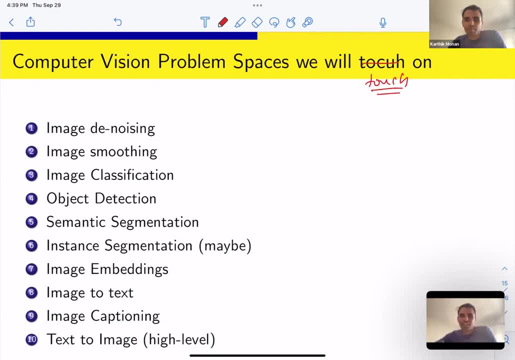 We'll get to, maybe sentences. We may not get to a paragraph in this course, But we'll have the building blocks in place in the course. So some of the things is things that you might know from the past: image denoising, image smoothing. 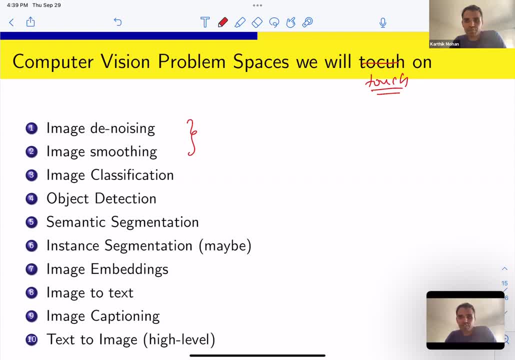 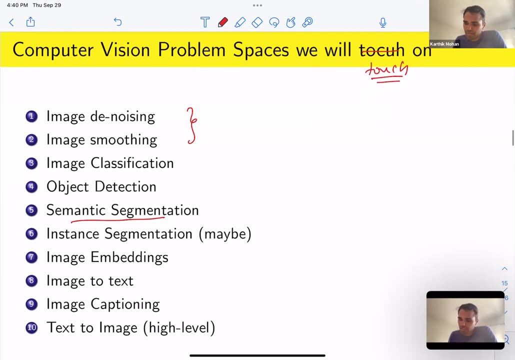 basic things, convolutions, OK. So image solutions: refresher of what you might have looked at before. Image classification might be new to some people based on your background in machine learning, Object detection, semantic segmentation, maybe instance segmentation, Image embeddings- this is a big one. 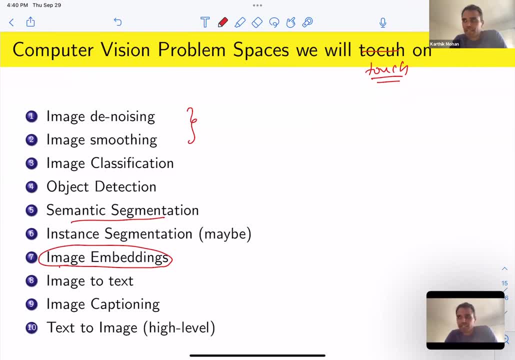 So there's fairly complicated models coming out these days which can do universal encoding of images or image encodings or embeddings- OK. So there's a lot of things that are useful in many, many situations. You can do different kinds of tasks once you have these embeddings. 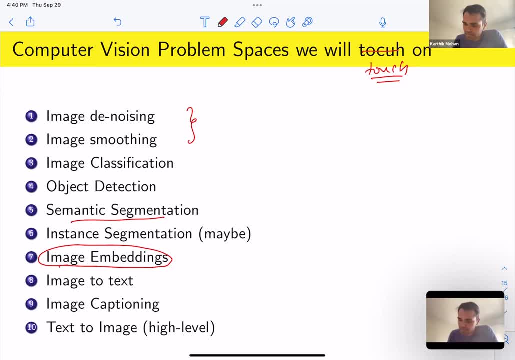 So what are embeddings and how are they useful? So we'll look at that in this lecture And then I think image-to-text is something we'll get to. So image-to-text and image captioning we'll get to. So we'll look at a model that actually you can take an image. 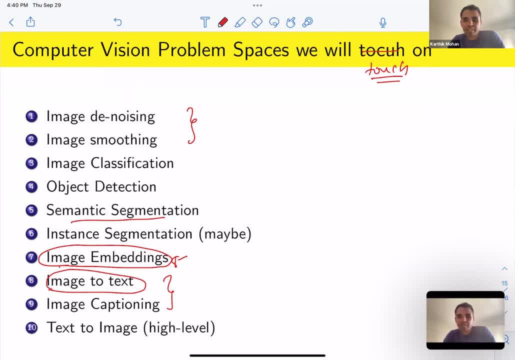 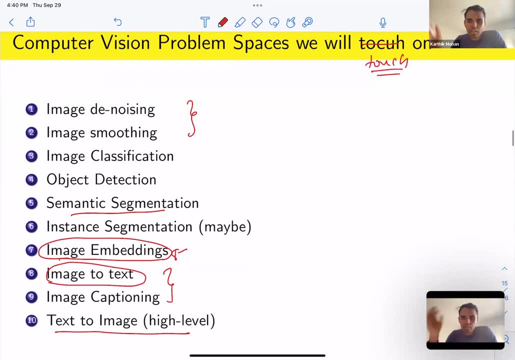 and then say: give me a caption for it, Tell me, describe the image to me. But text-to-image we'll cover at a high level. We'll look at the model architecture at a high level, But we may not have time to actually implement it. 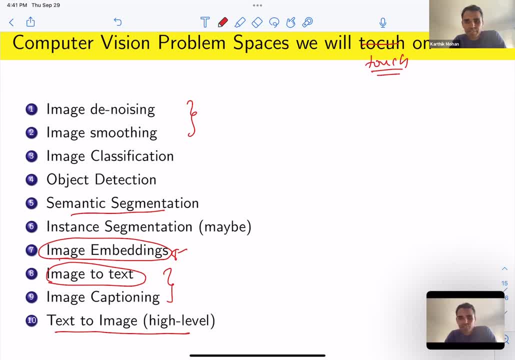 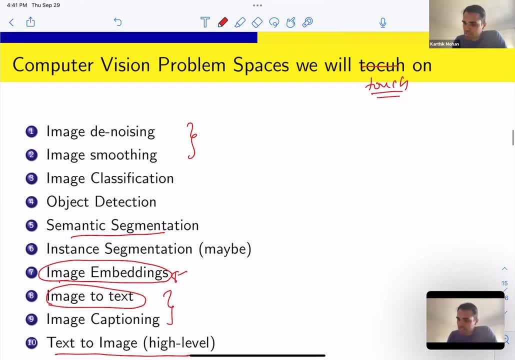 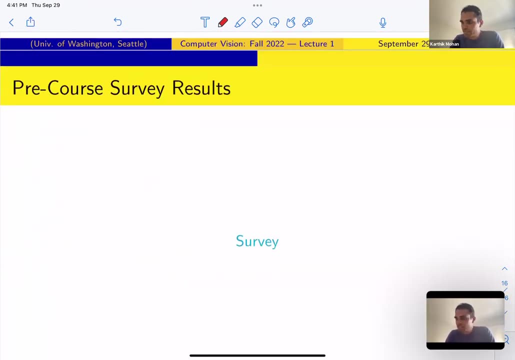 in the short duration of this course, Text-to-video. feel free to play around with that demo and read the paper on your own. Yeah, Does that sound good? Yes, OK, We also have the survey. Let me again Go through the results of the survey and see what's come up. 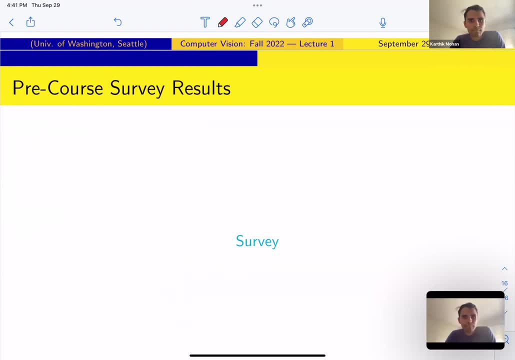 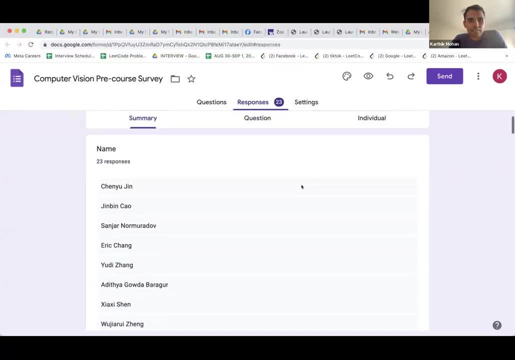 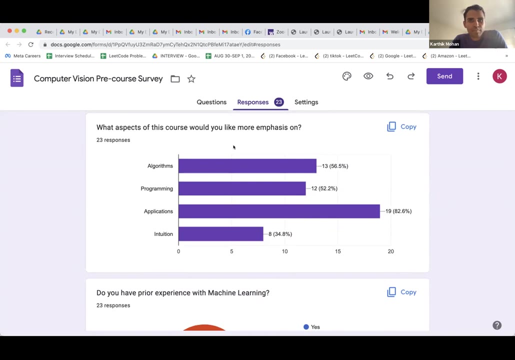 I'm going to pause the video again recording, OK. So here's a summary of the survey results. We have like 23 responses. OK, What aspects of this course would you like? more emphasis on A lot of people for applications. 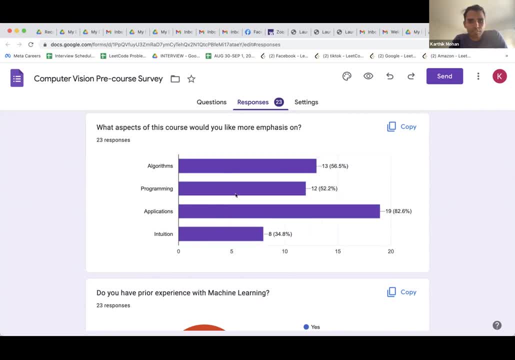 Algorithms, Programming And intuition. So all of these are interlinked. right, If you just did programming, great, But you may not have the intuition. If you just focus on intuition but you didn't do programming, then you might not get the implementation level. 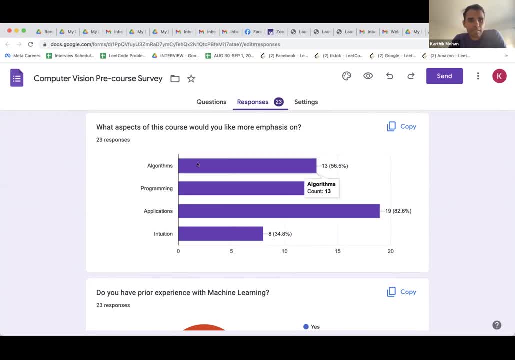 understanding of how you actually do it. Algorithms again: if you did programming and you had the intuition but you didn't understand the algorithms, then you may not be able to tweak things or explain things In an interview or to yourself also. what's happening. 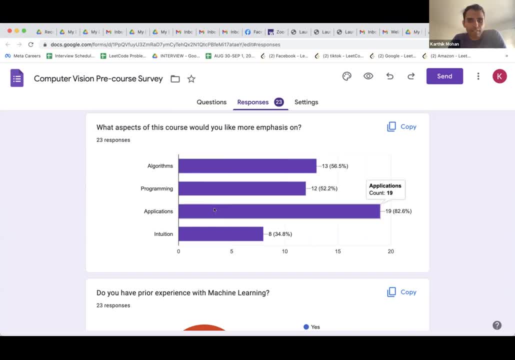 So understanding of algorithms is also important. But, yeah, we will be focusing a lot on applications, like we looked at: Keep the application in mind and then work on the models or algorithms that are needed, the programming pieces that are needed to go through those applications. right, 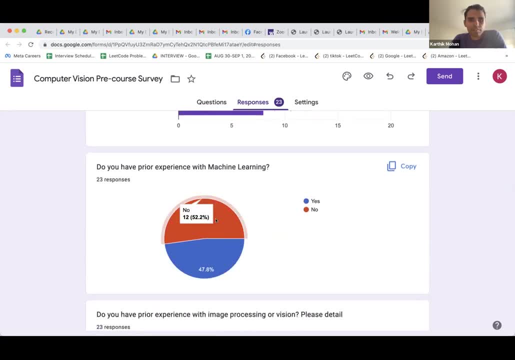 Do you have prior experience in machine learning? So 50% is no, 40% is yes Or 45% is yes. This is okay. To be honest, I was thinking that people will have a background in machine learning, because computer vision is an advanced course. 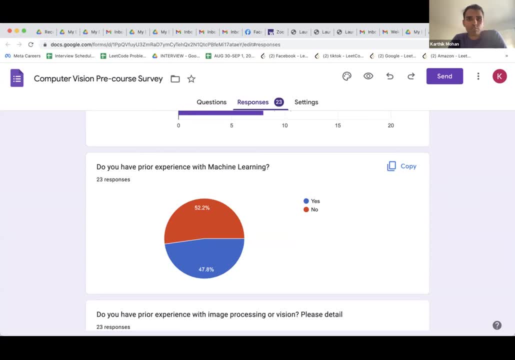 But I also understand that this is probably the first course that many people are taking in this program, right? Is that true? for people, Probably the first course you're taking first quarter. Yeah, So, given that is true and I think it was offered last year, 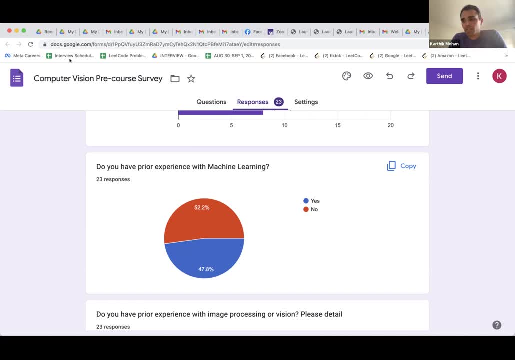 as well as the first in the autumn quarter. we will cover the necessary background in machine learning. However, if you think you're lagging behind somewhere, I'll point you to some resources so that you can catch up on machine learning as well as much as is needed. 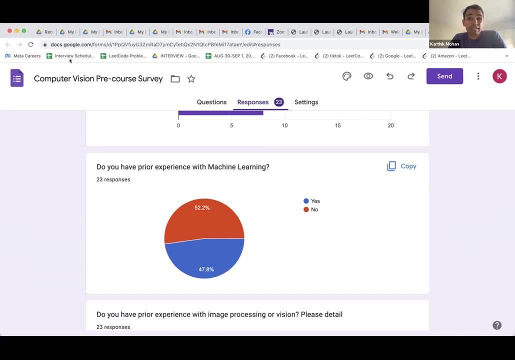 But we'll cover enough machine learning for computer vision And we might go through it quickly, given all the things that we want to go through in this course. Yeah, So a combination of some things we'll cover in the lecture plus your own, you know, reading on your own. 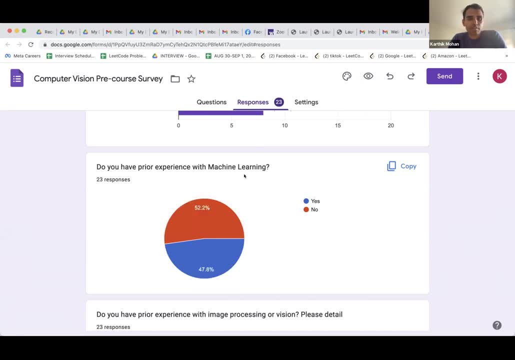 will help you get through the machine learning piece for this course, But also, I think, next quarter, I'm teaching a course, advanced introduction to machine learning, So you're welcome to take that course as well, to go in depth into many applications in machine learning beyond vision as well. 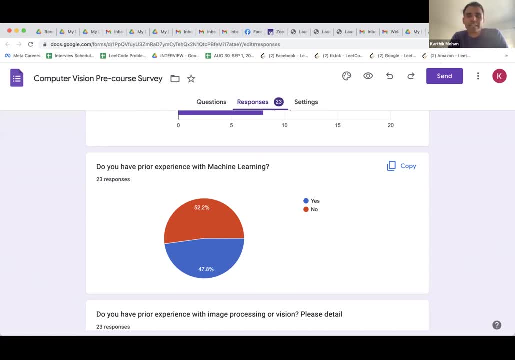 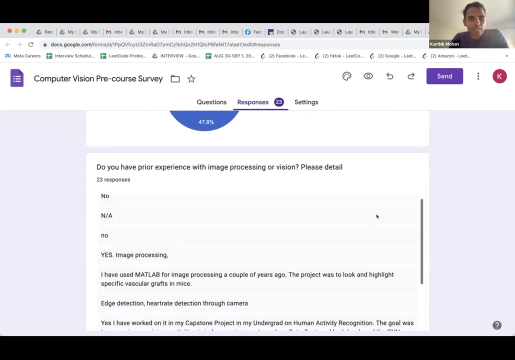 So it's widely applicable. Also, many methods, many algorithms get covered in that course, a really broad spectrum of things. So if you want to solidify your understanding of machine learning, I would point you to that course. Great, So that's that. 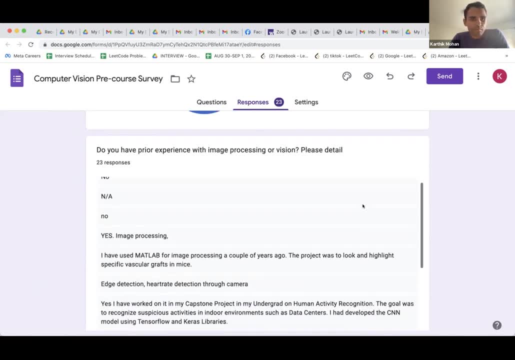 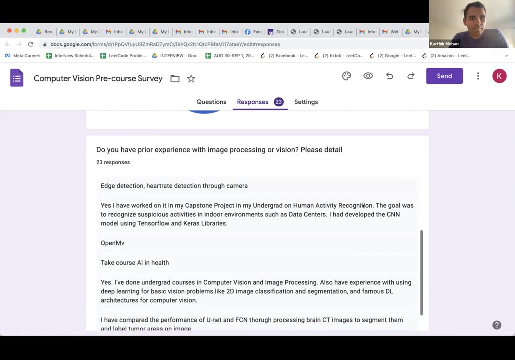 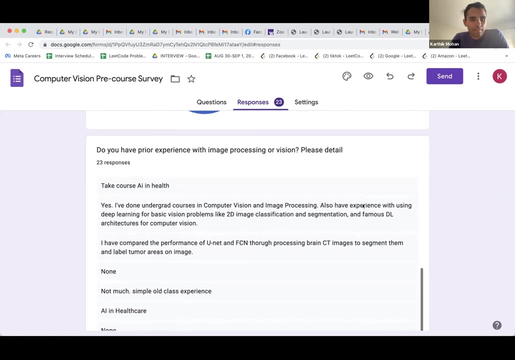 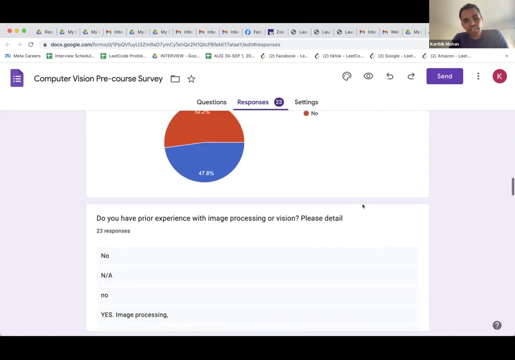 Do you have prior experience with image processing or vision? No, no, yes. MATLAB, edge detection, heart rate detection- Okay, great, Okay. Human activity recognition: Okay. OpenMV: Yeah, and healthcare: Yeah, Okay. It helps to have some background in image processing. 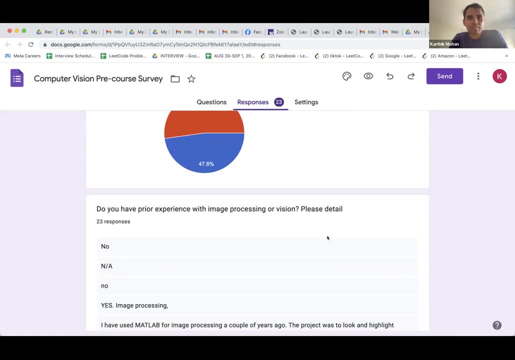 If not the first two assignments of this course, we are going to kind of brush up our background on image processing. So some denoising, some smoothing, some transformations on images, some basic things that should be part of your understanding and toolkit. 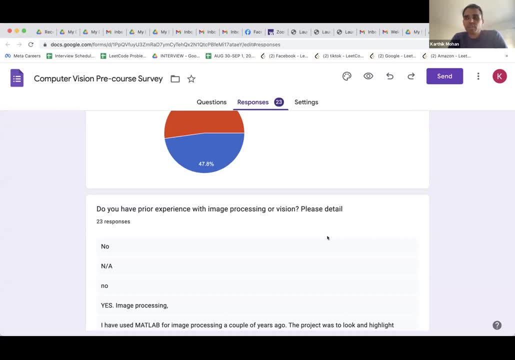 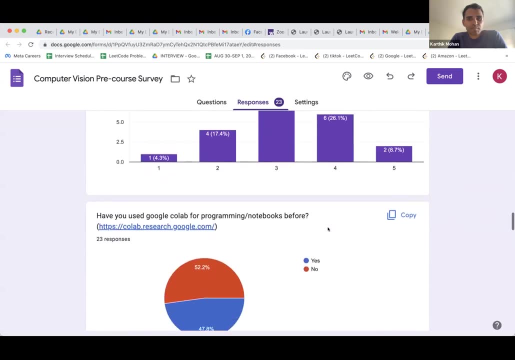 for working with images we'll cover in the first two assignments. So, as you work on that, if you didn't have the background, you'll catch up. If you had the background, you'll just refresh it right. So yeah, this is something I want to mention. 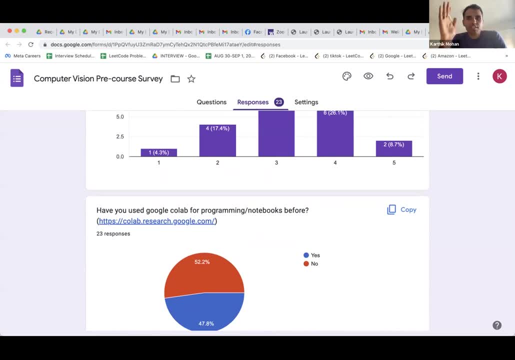 In this class we will be catering to the average. So if you are, you know, lower on the understanding side or you're catching up on many things, you may have to work harder. But if you've only used PyTorch and TensorFlow, 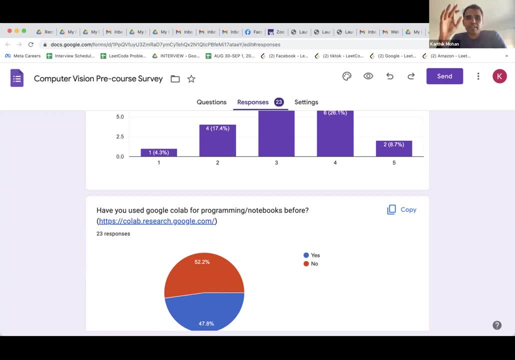 and you've done a lot of computer vision applications, you might find a little bit slow on the progress that we are, you know, making in this course. So we will be taking a balanced approach. For that reason you may find it slower or faster. 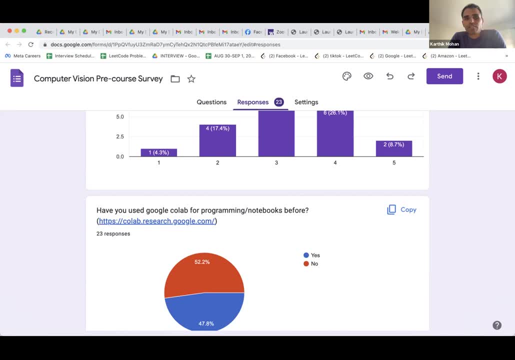 the pace at which we are going right, But if, in any case, you're finding it slower or faster, just reach out to me and we'll have ways to deal with that. So if you're going slower, then I'll give you a little bit more time. 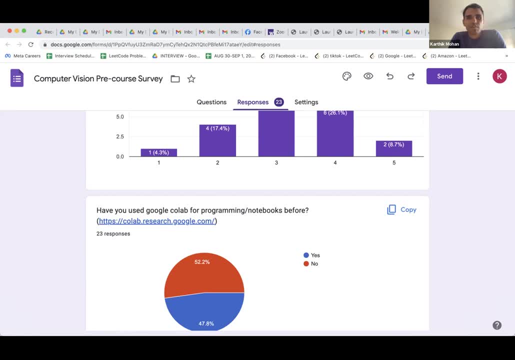 I'll give you additional things to work on your own so you can augment your understanding. If you think it's going too fast, then we should also discuss that so that you feel comfortable going forward with deep learning that will be coming up and all the other assignments that will be coming up. 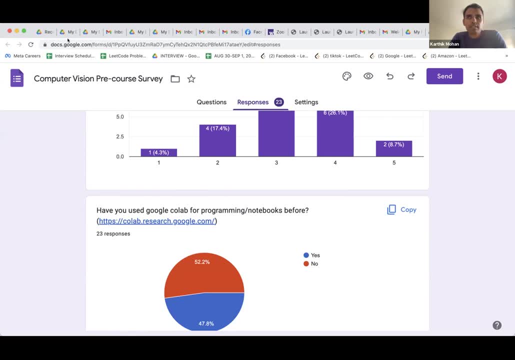 Yeah I mean, but it's a great. I would say this course is an amazing course to get started with machine learning in general, but it'll also involve a lot of work, So you will learn a lot through programming and programming assignments. 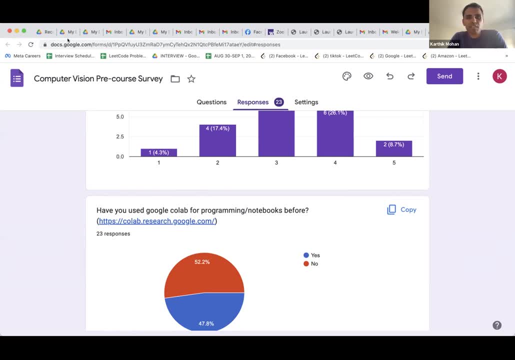 which also means you'll have to spend enough time for it. But if you did that, you will get the most out of this course, right? So but it's a great thing. I mean, computer vision is really exciting field There's, as you saw, 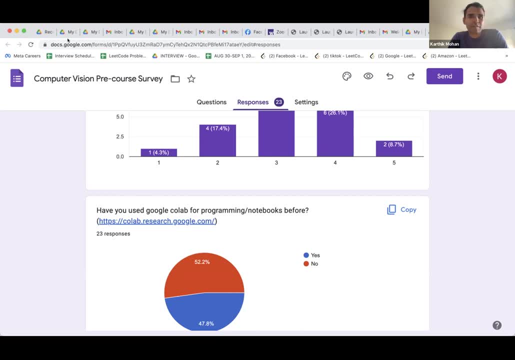 there was, like some recent amazing innovation that just happened this week, So these kinds of things keep happening, So it's a great field to be in. So I think the hard work that you put in to this course will definitely give you benefits going forward. 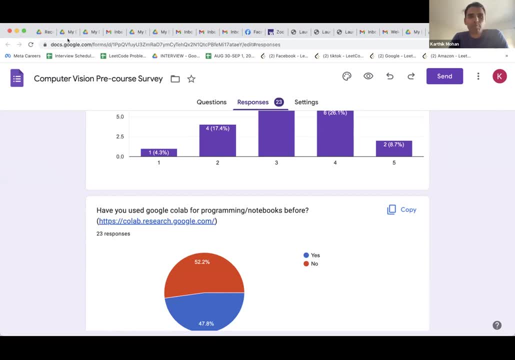 And anything that you think. oh, I still don't understand back propagation. Okay, that's where we have the next course on machine learning. So, because we might just brush through back propagation, we might just brush through neural networks, so we can get to the topics that. 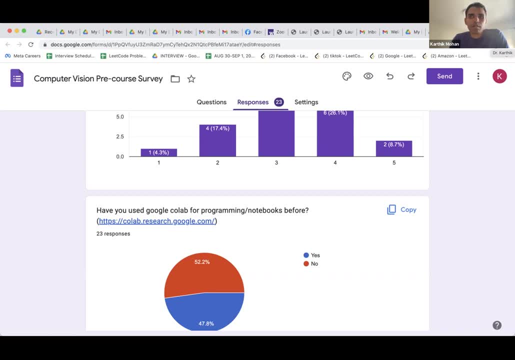 applications that we want to go to. So, wherever you think there is missing gaps or you want to have a deeper understanding, feel free to take the next course or do your own learning right, And there's so many resources available. Yeah, I think that's what I want to share here. 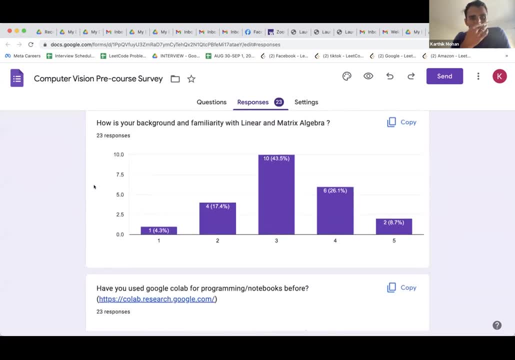 Okay, How is your background and familiarity with linear and matrix algebra? So we're okay with it. Yeah, I think we'll be covering some of this in the first two assignments as well. So some mathematical background that's required for processing images. 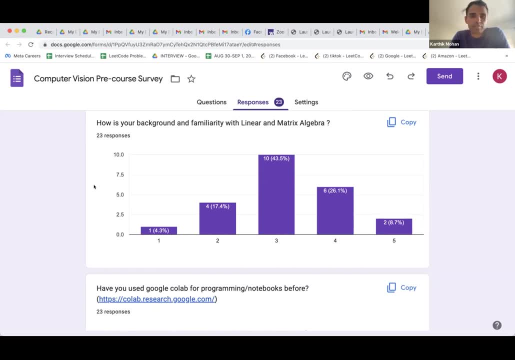 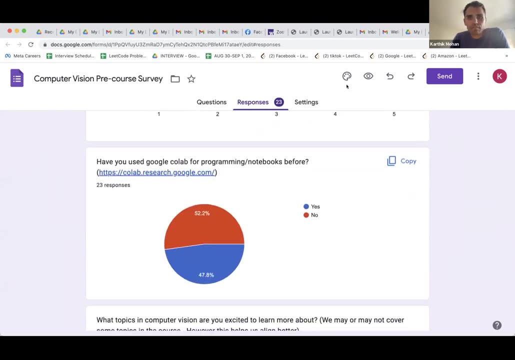 So you'll kind of go through it and also programming backgrounds. You need to be able to program and code these things, And the primary language for coding we'll be using is Python in this course And you're encouraged to use the Google collab. 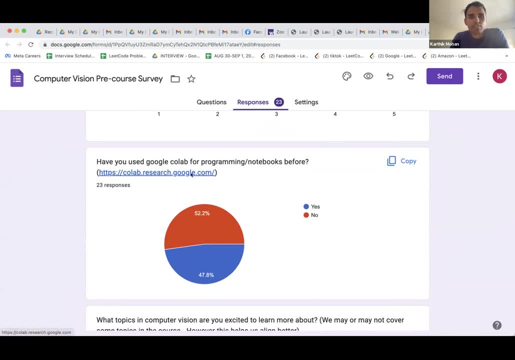 as a way to submit assignments, And we'll also probably share template for programming in Google collab So you can get started with some startup code in Google collab and then fill in the missing pieces and then make your submission right. So most of the assignments are going to be programming. 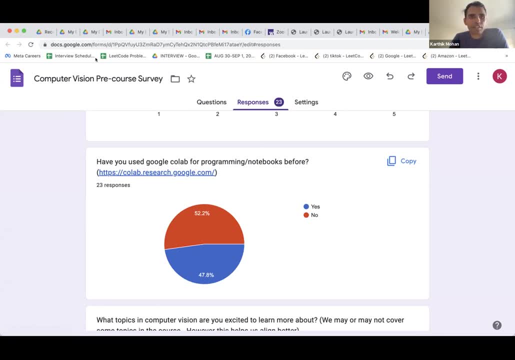 So if you've been using MATLAB or something else, you may have to switch to Python. MATLAB is great for prototyping, but not good for an industry context. So if you've been using MATLAB, it's a good time to learn Python. 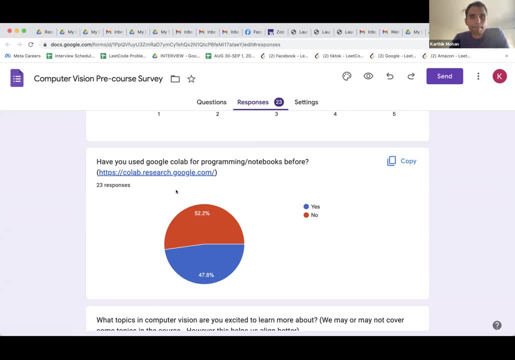 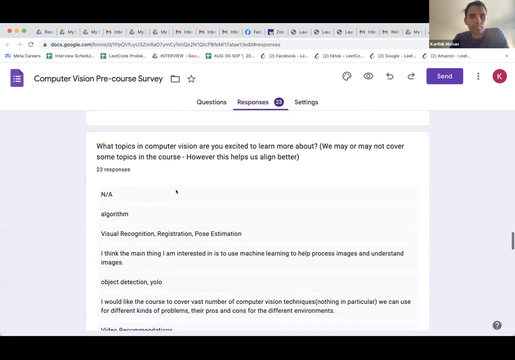 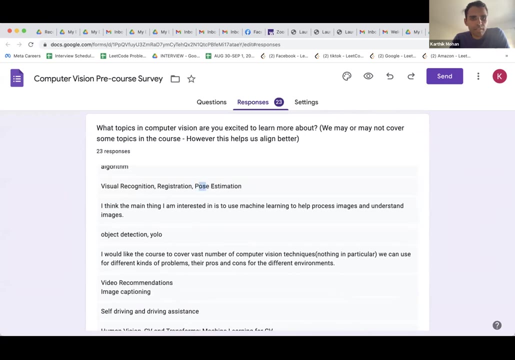 It's a good time to learn Python and switch to Python. Okay, All right. What topics in computer vision? are you excited to learn more about? Algorithms, visual recognition, pose estimation, Yeah, So these are some advanced topics. We'll see. 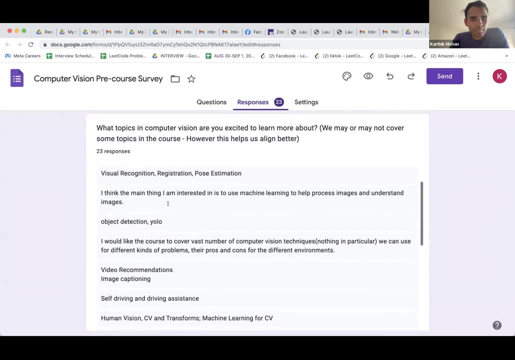 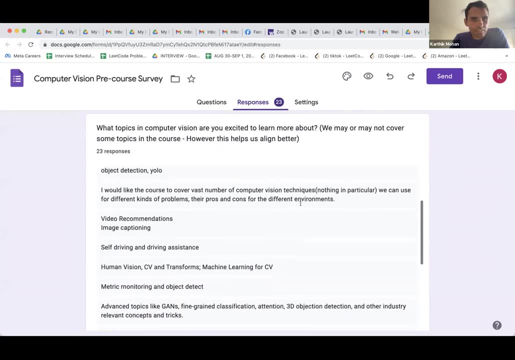 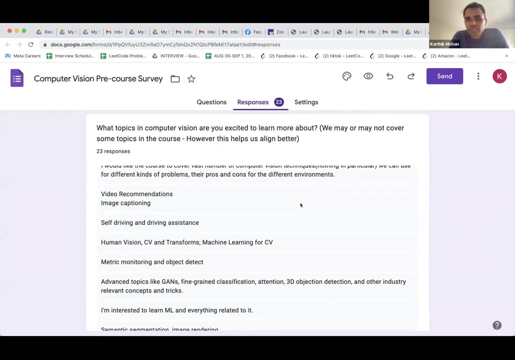 We may or may not get to it. Yeah. help process images: Yeah, for sure We'll be doing that. Object detection: yes. Video recommendations: That's a good one. Yeah, there's a lot of industry applications to video recommendations. 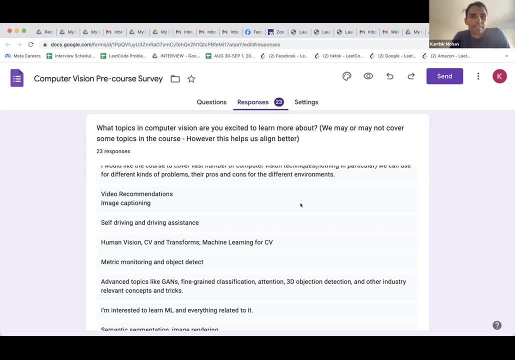 For instance, InstaReel recommendations or TikTok recommendations. So if you were to interview for one of these companies, this is a good topic. YouTube recommendations: I think we'll like we had a separate course on recommended systems in summer. 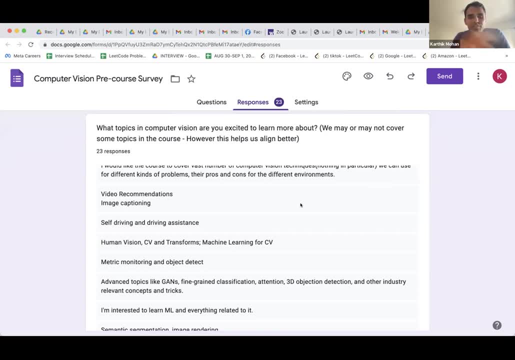 So again, you know, you can spend a whole summer- I mean, you can spend a whole two months- on just recommendations. So maybe we'll- I'll just keep this in mind, Maybe we'll touch on this in one of the lectures as an application. 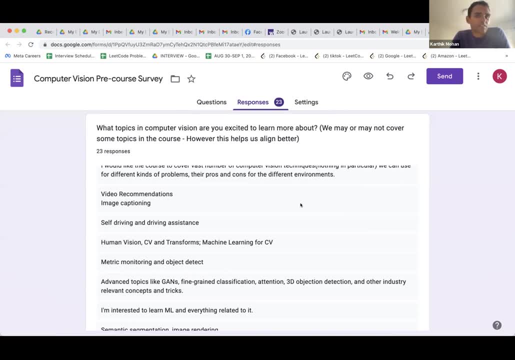 at a high level. So we can always touch things on a high level, like at a system design level or a machine learning design level. We can always go through things, But, as you know, a lot of learning happens in the details as well. 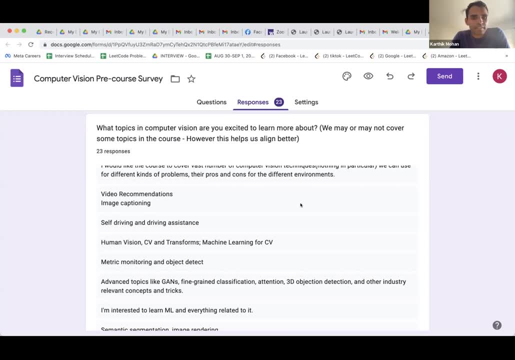 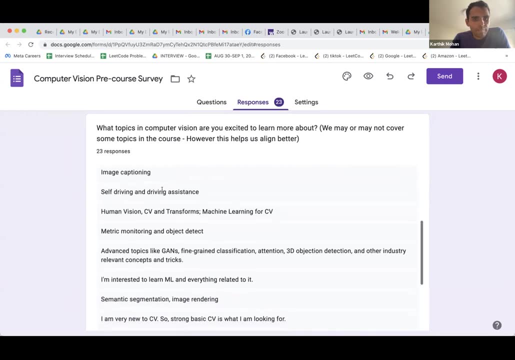 So we may not be able to go into details or recommendations, but I think that's a good call out. We'll probably touch on this in one of the lectures. Image captioning: Yeah, Image to text. We spoke about that. Self-driving and driving assistance. 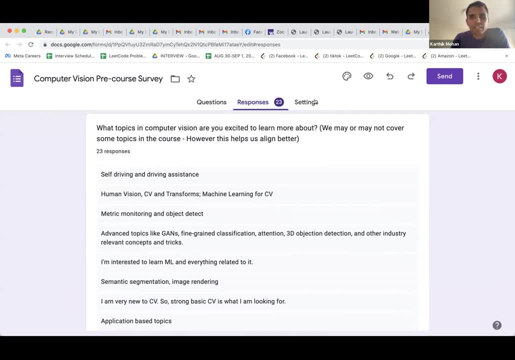 Again, maybe at a design level. we'll probably go through this and then you can imagine how the pieces will fit together. So we'll probably go. we might go at that level. Human vision, CV transforms: Yeah, Metric monitoring and object detection. 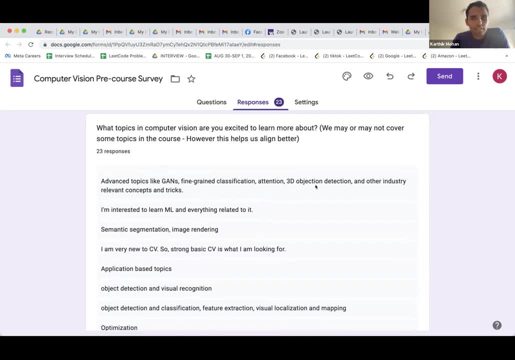 GANs, Yeah Yeah. industry, Yeah. So we will be keeping things relevant to the industry setting because it's a professional master's program. So we will talk about scalability, We will talk about latency, We'll talk about trade-offs. 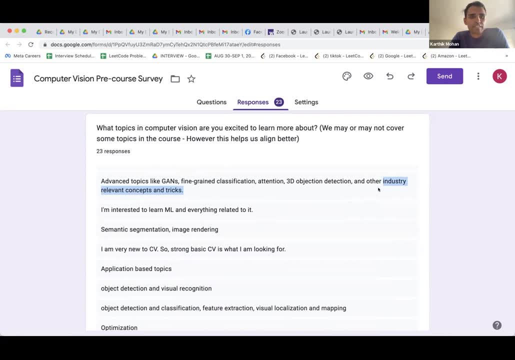 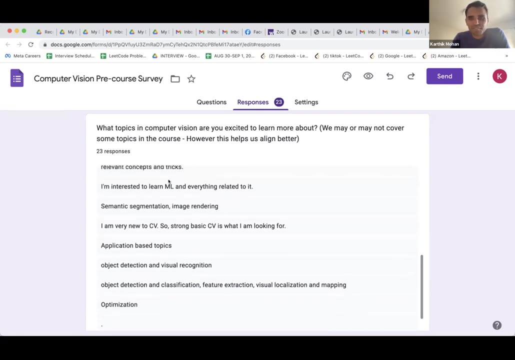 that are very practical in an industry setting right. So we'll definitely do that. But, yeah, will we have time to talk about GANs? I don't know. There's a lot going on in the vision literature, So, and we only have two and a half months. 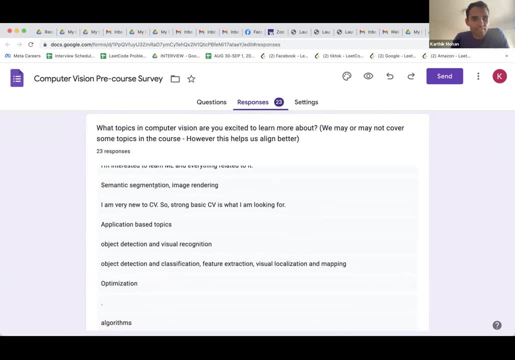 Interest in learning machine learning: Yeah, we'll do a crash course on machine learning in this course. Create object detection. classification: Yeah Yeah. Relation to real life application: Okay, I think we've covered it. Yeah, This is great. 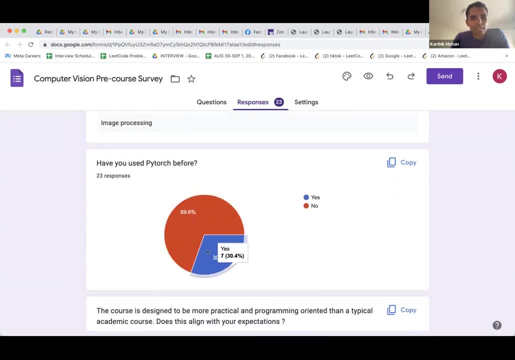 Have you used PyTorch before? No, Yeah, So we'll be using PyTorch for when we get to our neural networks, back propagation, deep learning module, and looking at some of the, let's say, you want to do image to text. 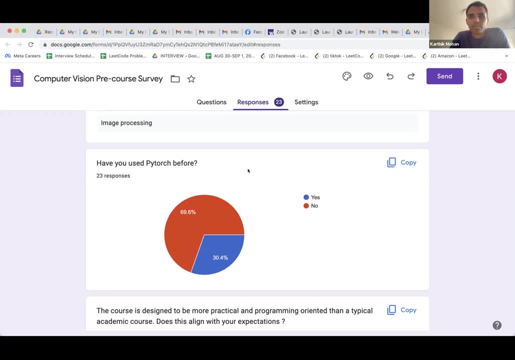 Okay, That's a complete deep learning model. You're going to have the computer vision on one side with all the CNNs getting stacked, And then you're going to have the NLP modules, maybe with LSTMs or something else, And then PyTorch is going to help you put those things together. 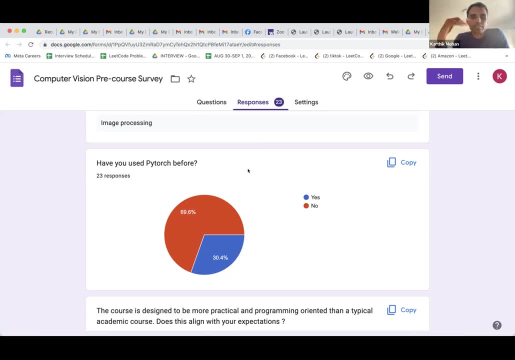 So we'll have a few assignments on PyTorch towards the end of this course. So you get exposed to PyTorch And again it'll be a learning curve, So you will have to. you may find yourself putting in extra time. 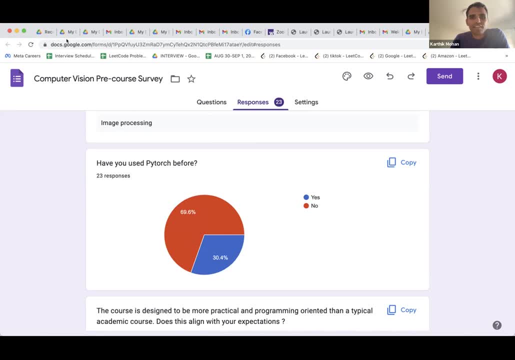 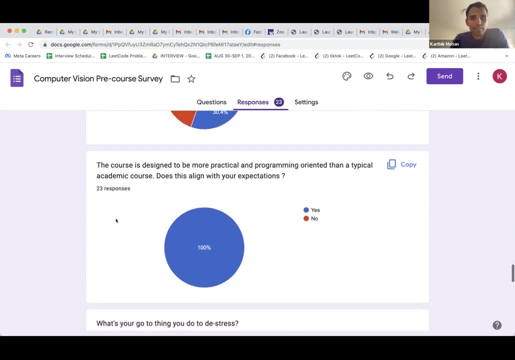 to even get things going, So, but it's totally worth it. Right, Yeah, Okay, This is great, A hundred percent Okay. What's your go-to thing to de-stress? Looking out, running in the park, rock climbing, watching TV series, meditation. 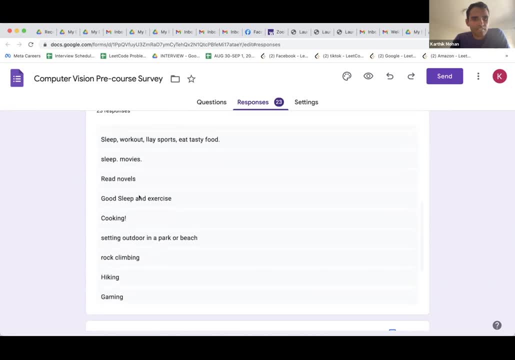 video games, listening to music: Yeah, Sleep, Yeah, Sleep is so important. You know, we don't usually talk about these things much in a class because it's like your personal thing, Right, But I like to talk about it because it impacts your learning. 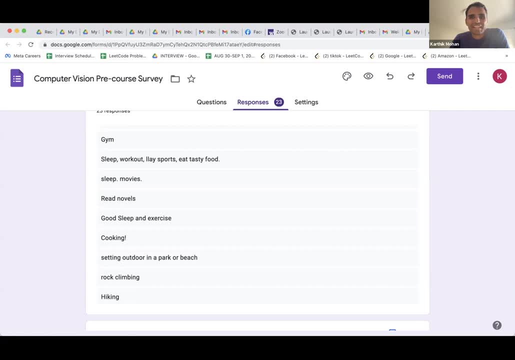 If you didn't sleep? what are you going to learn in the class? If you didn't take care of your stress, what are you going to learn in the class? It's just going to go over your head, or you might be nodding your head. 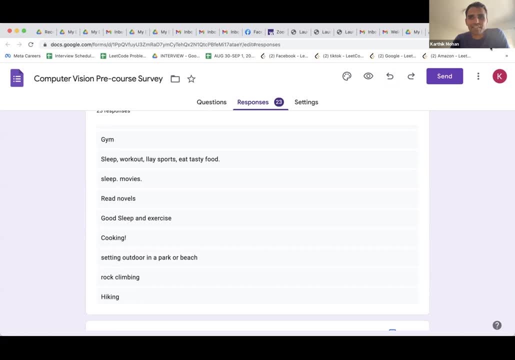 but it's not registering. So these things happen when we are sleep deprived or when we are stressed out, Right? So it's good to at least know how you. yeah, this is great. Seattle's a great place to do a lot of outdoor stuff. 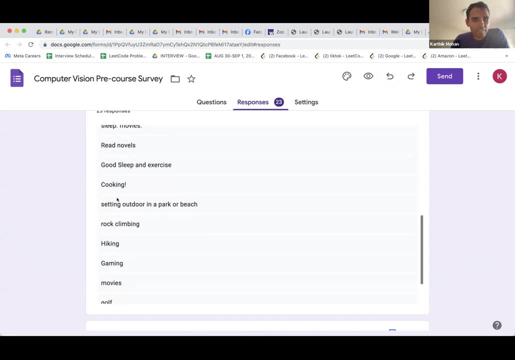 So nice to see some of these hiking, rock climbing, all of that Great, Awesome Cooking: Yeah, Pandemic has taught us how to cook. If you didn't know already how to cook, you were forced to start cooking, Right. 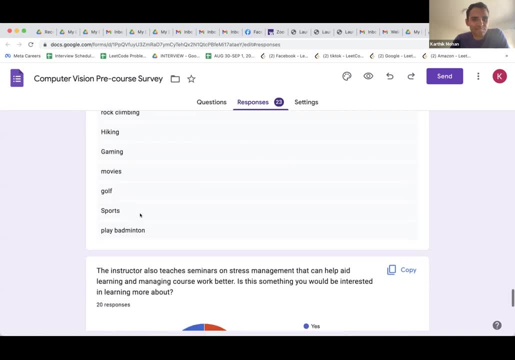 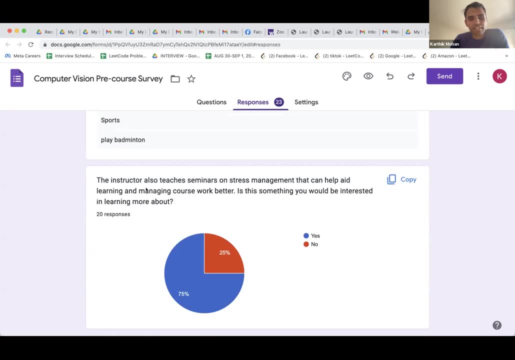 Great, Awesome, Okay, Yeah, I also wanted to mention that I kind of have a second- I could say part-time- hobby that I do over the weekends as I teach seminars on stress management, And I find this to be incredibly helpful for myself. 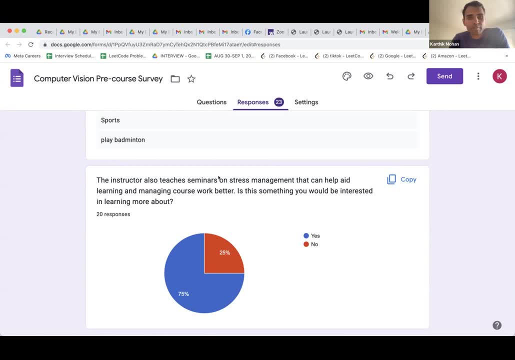 but also many of my students have taken some of these seminars in the past and have benefited themselves, like even to the extent of helping them land a job because they were not so stressed in their interview or interview prep. So there are the. all these things are really real. 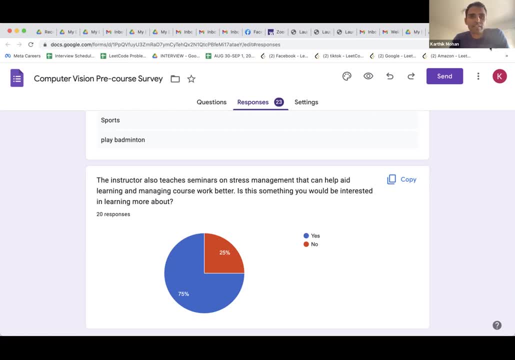 like interview anxiety, you know getting that call, you know making sure you land a job, all the stress of that- all of that is really real. You cannot brush it aside. So if there are things that are really real, like you know, 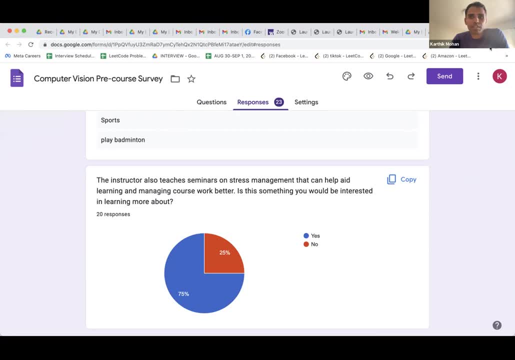 I'm not going to go into too much detail, but I'm going to talk about some of the things that are really really important, Right? So if there are tools that can help you smoothen your experience, why not? So that's what these seminars are about. 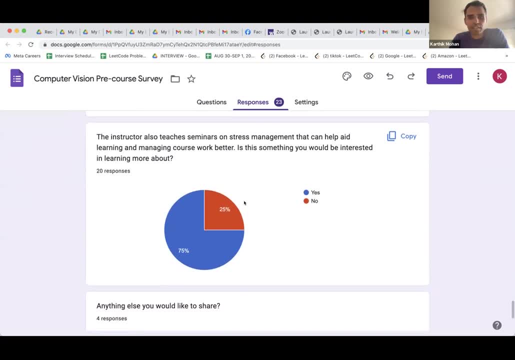 I might share, especially those who have shared. you would be interested in learning about it. I'll probably share some resources or seminars coming up that I'll be hosting outside of class time, Right, But definitely going to help you in class time as well. 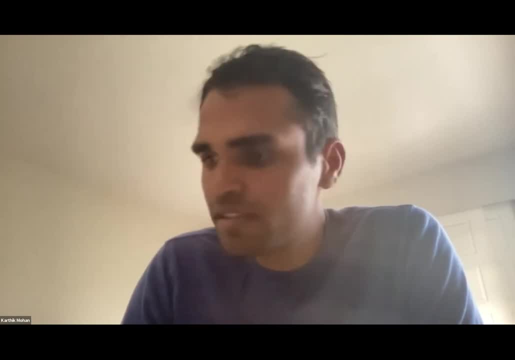 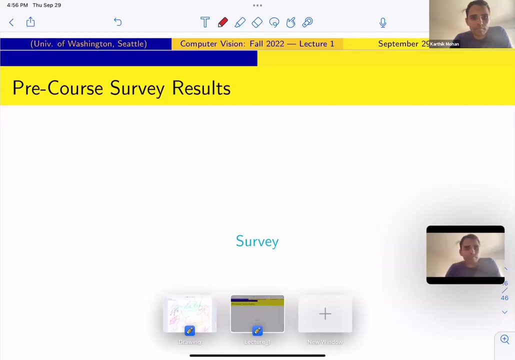 Okay, All right, So the next slide. So this is a webinar. sorry survey we went through just now. Okay, great, It's good to align on expectations. So I think I think this survey is useful, for me for sure. 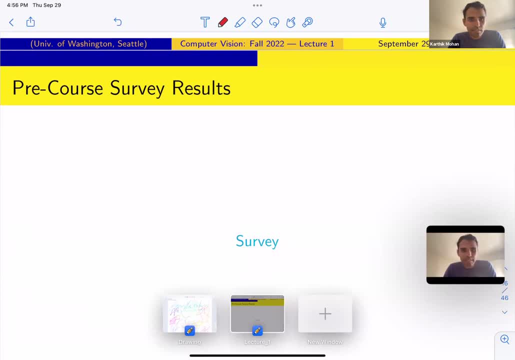 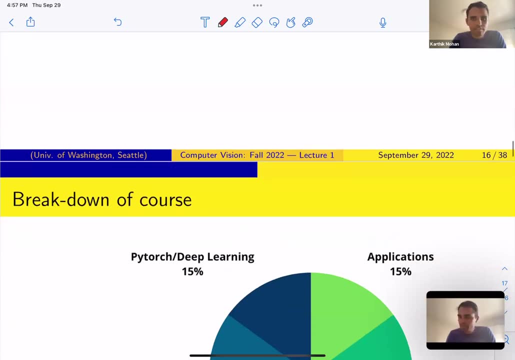 Because now I understand, you know where people are, What's going on. Okay, Yeah, that makes sense. Okay, Great. So let's go to. Let's go to some more logistics and high level understanding of The breakdown of the course and things like that. 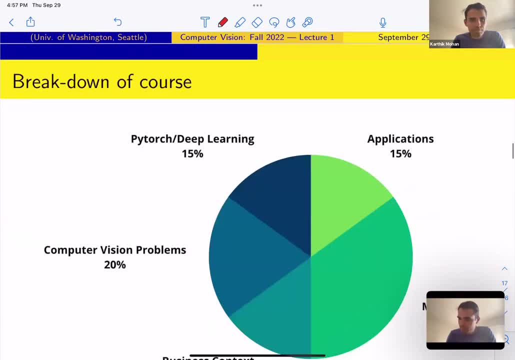 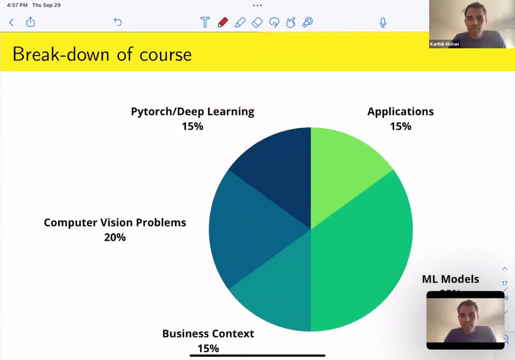 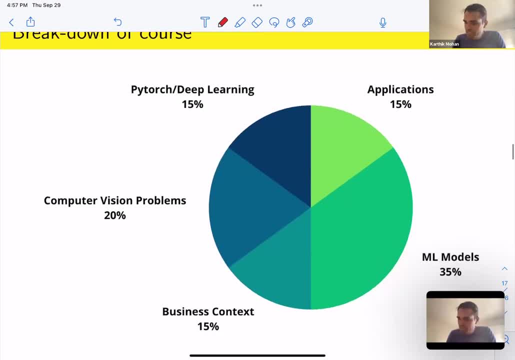 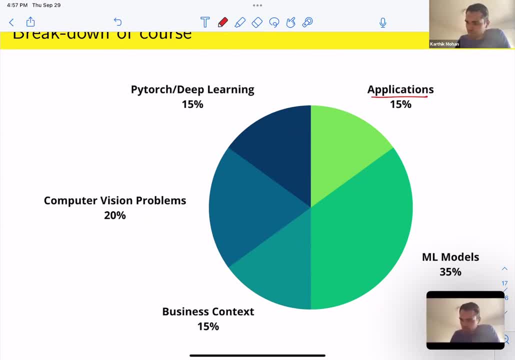 Right, Okay, There's machine learning models. So this is like the fundamental building block For almost anything that's you know happening in industry these days as machine learning Models. You can say you know, deep learning is a subset of machine learning. 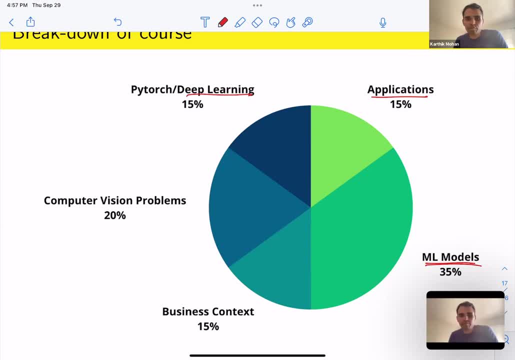 Like more sophisticated methods that can That have a much better performance. So we'll start with machine learning models with machine learning models and then we'll jump to deep learning, maybe in week five or week six of this course. right, so once we've covered enough background on applications and a background on 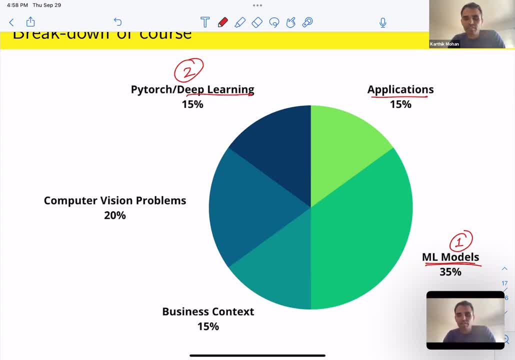 machine learning. you've done enough. uh, got hands-on with some of the programming assignments. you feel more comfortable, then we'll get started with pytorch and deep learning and then again explore more of these applications. um, computer vision problems, yeah, so there's distinct problems in computer vision: object detection, instant segmentation. 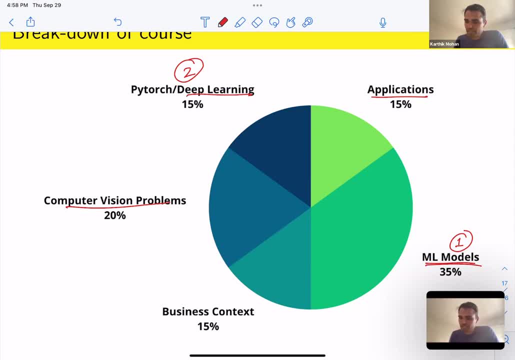 image to text, text to image. so we'll be looking at some of them. uh, in this course there's a lot of classic computer vision um that people usually cover in a computer vision course, so i am i am kind of choosing to skip it in favor of things that will actually be used in industry. 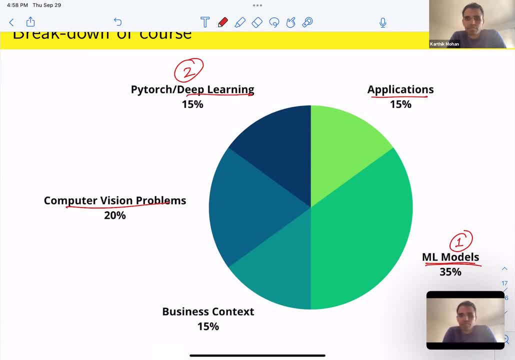 does that sound good for people, so you might. you might want to read that and i will share the link in the description below if you don't mind. to understand color better? we may not be able to. we may not be discussing that so much in this course, but it might be part of a classic academic computer vision course. right, because if you take 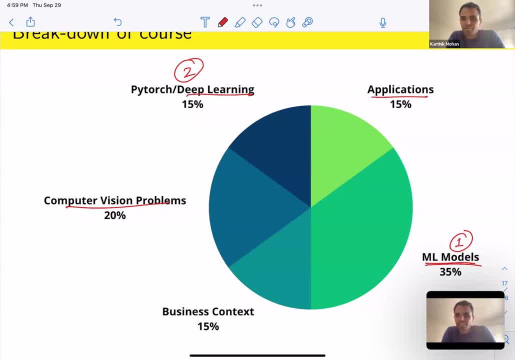 time for that. then you will have less time for all the cool applications that you may want to look at, you know, as part of this course. so we'll skip some topics in favor of other topics that are more interesting and useful. that we believe is more useful for us. yeah. 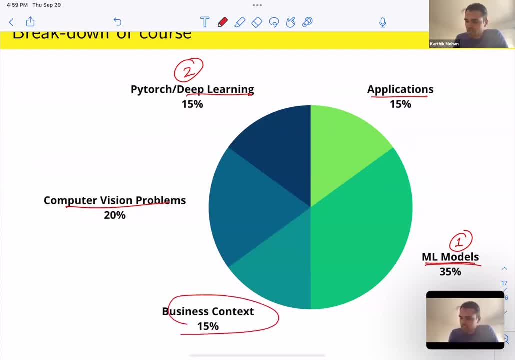 yeah, okay, and then business context: yeah, so this is very important. um, anytime you look at anything. um, like i want to do classification, okay, i went to scikit-learn i, you know, picked my favorite classification library, classification module, and then i applied it to my data set and i got results. yay, i'm done, i got, i understand classification. then you, then you join. 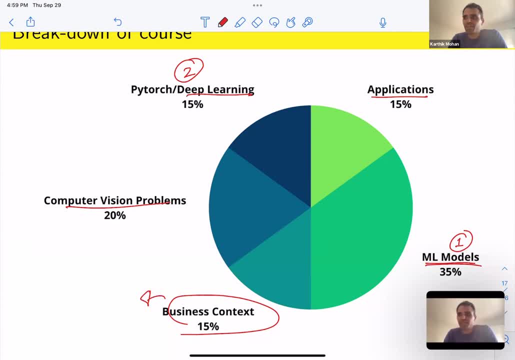 uh, machine learning team. and then you realize, oh my gosh, there is so much more to just classification. there's this whole data pipeline, there's this whole machine learning pipeline, there's this issue of scalability- and scikit-learn is probably going to fail at that point- and you're like: oh my. 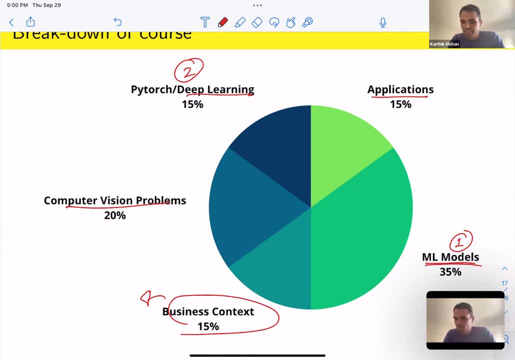 god, i need to do something about this, something about that. so all of that is business context: understanding how things happen in a real business when you implement these things. business context also refers to what, what applications does a business really care about? um, like in computer vision, how does computer 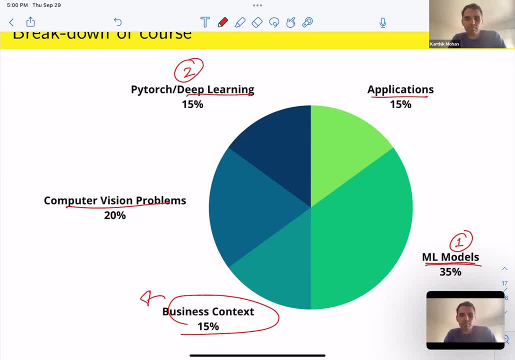 vision apply in amazon, for instance? have you thought about it? people do use computer vision in amazon. where do they use it? and yeah, maybe this is a good thing to ask right now. uh, feel free to share, maybe in objects sorting using, uh, industrial robotics manipulator. i mean yes, yes, 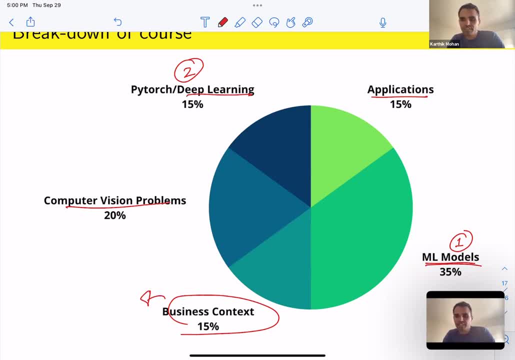 have you guys seen one of those videos that, uh, automated sorting using a robot? yeah, yep, absolutely so. different things are going on a conveyor belt and then you want to put the objects in the right bin so that they get sorted, and then you can want, but for that you need to. 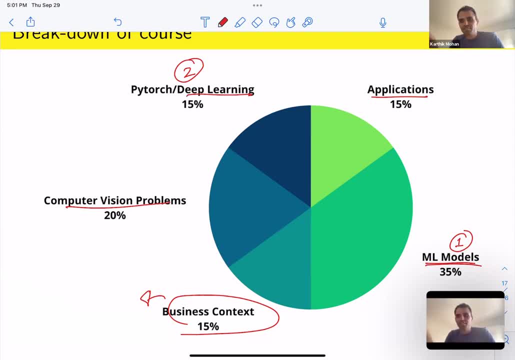 be really quick. so it combines robotics and vision, because the robotics is taking care of the mechanical moving pieces and the vision is telling the robot what to do. okay, this is an object. you need to do this, all right, great. any other example- visual advertisements, yeah, i mean, you know there's many interesting examples, like, for instance, you have an image of 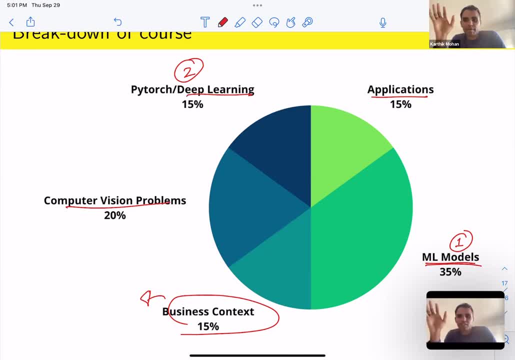 a product and some. for some reason, the image is not matching up with the text description. uh, someone decided, some seller decided, to put up some product on amazon. they're like these words are really cool, they get a lot of attention. let me put it up and then, but it's not matching up with. 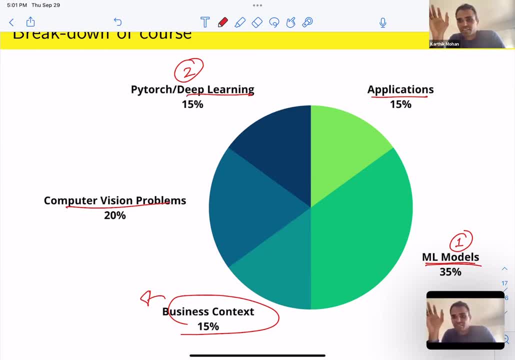 the image or the. the text is right, but the image is something else. it's like: uh, it's grabbing you attention, but it's not really connected to the product, so these could be confusing customers. if that's the case, you want to know if they are confusing or not. so what? what part of computation? 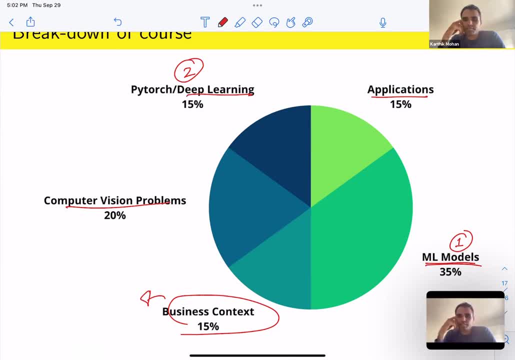 would you apply like? what kind of uh model would you apply there Anyone? Maybe also an example of Prime Air drone that delivers goods and that drone use computer vision to navigate through the infrastructure? Yep, yep, that's definitely there. Yeah, Prime Air is all vision, yep. 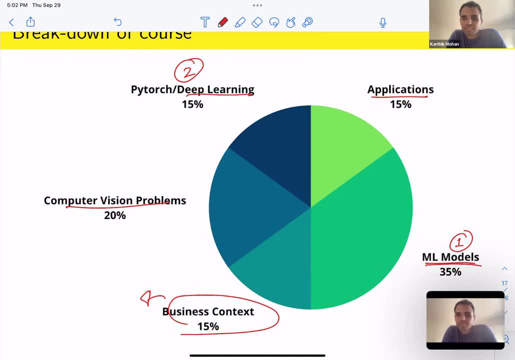 In the context of spurious image or spurious product descriptions. you can do image captioning, right. You caption an image and see if that caption matches up with the description, or the keywords there match up. If they don't match up, then that's a spurious kind of hodgepodge of text and image. 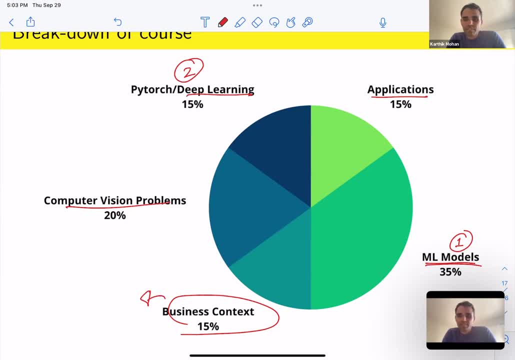 that the seller decided to put up on Amazon. So that's an example. So there's many, many such applications that you can have. Also, I think what's it called, What's it called? where you actually walk into a store and you don't have to pay, and then 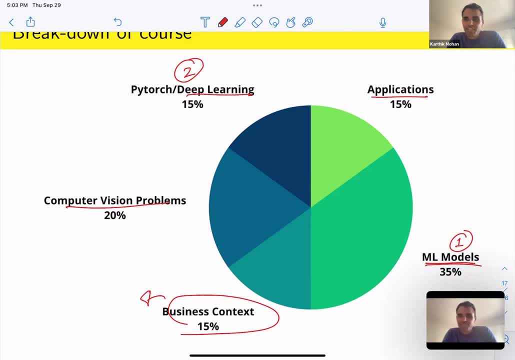 forgot the name. You just pick whatever you want from the store and then you just Amazon Go. yeah, great. So Amazon Go is again an example of vision. right, There's many things going on there, but one of them is vision. 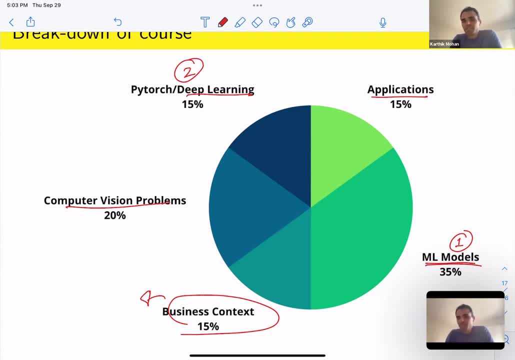 Okay. So it's useful to think in terms of the business context as well. So if you want to land a job in computer vision, just think about what companies out there might be using what kind of models for what kind of applications. So helping you think along these lines. 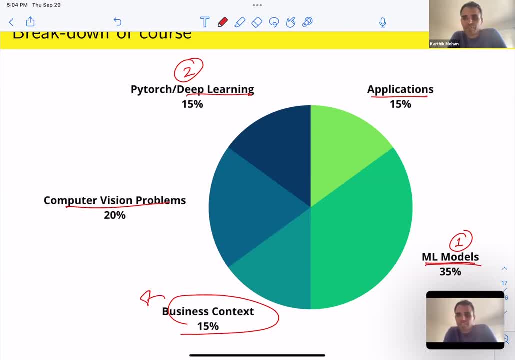 will help you in your interviews as well, at some point when you want to start interviewing And if you think you want to go down the route of computer vision. all of these I mean not just for this course, any course that you're taking in the machine learning. 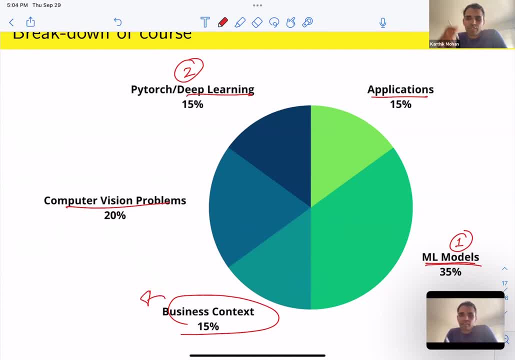 deep learning specialization. take any method and say which company would I use this method for and for what application, So that will keep things real for you. So you can see that, okay, what are you learning here is actually something you're going to apply somewhere. 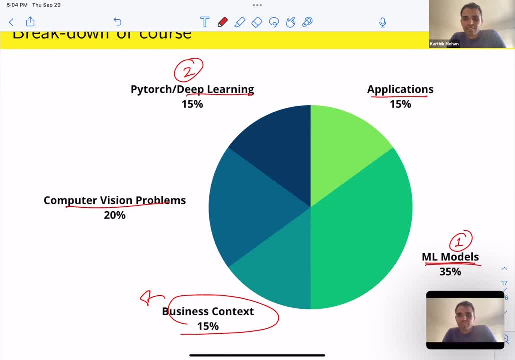 someplace, And that's also a skillset to be able to model a business problem as a machine learning or a computer vision problem. That's also a skillset that takes time And it's going to help you. Sorry, you both were saying something. 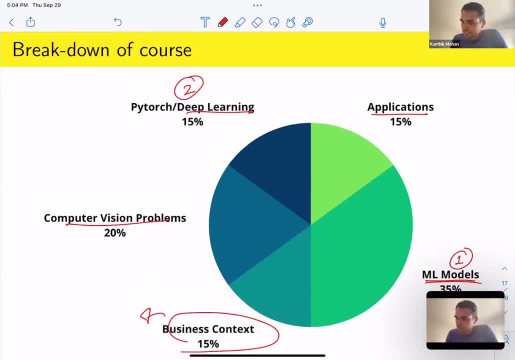 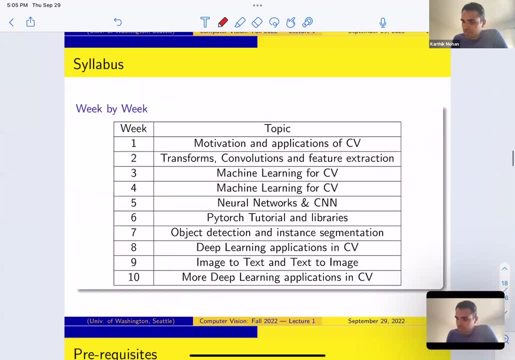 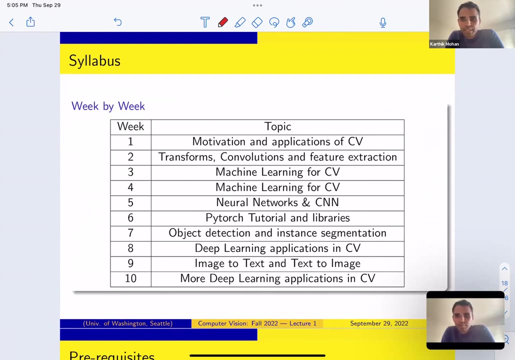 Okay, great, So that's a breakdown of the course. So in terms of week by week syllabus, so we have about, I think, 10 or 11 weeks. So, okay, this is kind of the rough breakdown of what we'll be looking at with each week. 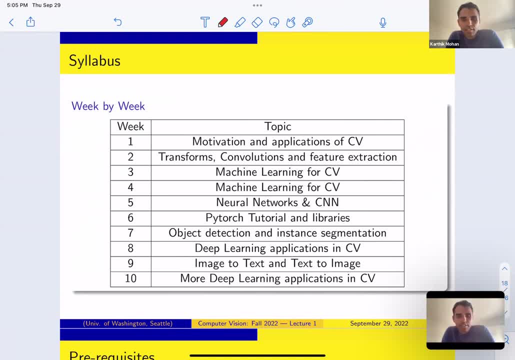 So this week, of course, is short, but motivation, applications of computer vision, and we'll be looking at some image processing. background in week two: transforms, convolutions, feature extraction, And then we'll be going into machine learning for computer vision. 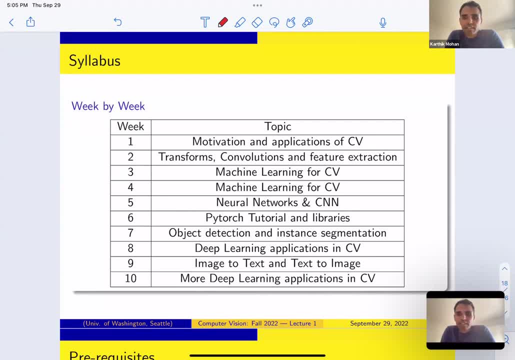 So some of the classic topics in machine learning that are pertinent for computer vision, like image classification, for instance, or feature engineering for image classification- How do you use SIFT features? Things like that we'll cover in machine learning for computer vision. 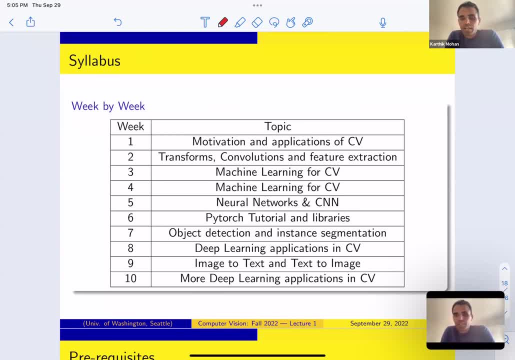 How do you do clustering of images? How do you identify digits in images? How do you classify different kinds of problems, spaces? So that'll be week three and four, Week five, now that we have covered basics of machine learning and some basics of computer vision. 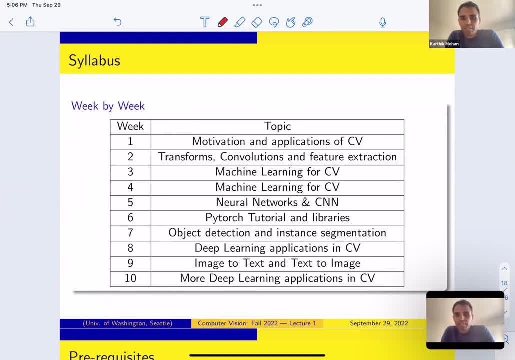 and we will jump into neural networks and convolutional neural networks. So CNN is going to be kind of the bread and butter of some of the advanced computer vision methods that we'll be looking at in this course, But also in general, CNN is like a staple diet. 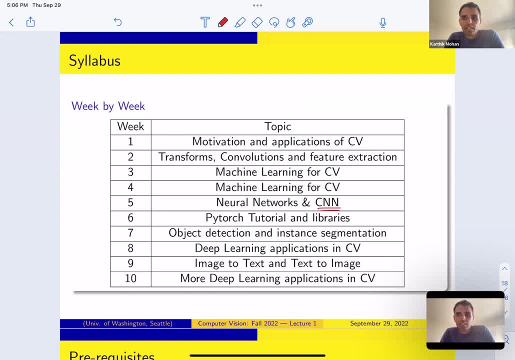 You'll see CNN show up in almost every advanced computer vision model, including image-to-text or text-to-image. There's a CNN happening somewhere, Then we'll be looking at. obviously, you need to know how to implement neural networks, So that's where PyTorch comes in. 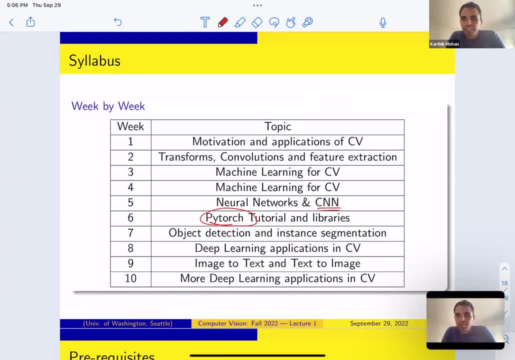 So we'll have a PyTorch tutorial. We'll cover some of it in class, but also, I think our PA Ayush will also cover it in the office hours or the quiz section. So you'll also get more exposure to that there. 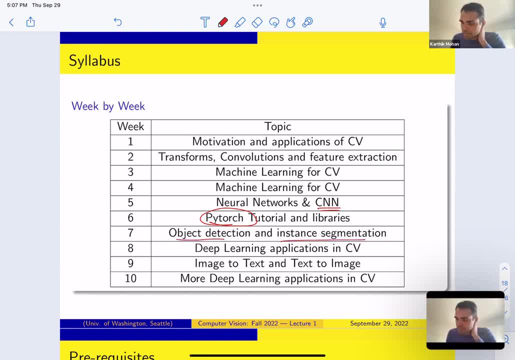 And then we'll move into object detection, instant segmentation or semantic segmentation, And then we'll look into the neural networks, And then we'll look into some more of the deep learning application CV, especially image-to-text and text-to-image, And yeah, if you have more time we'll be as 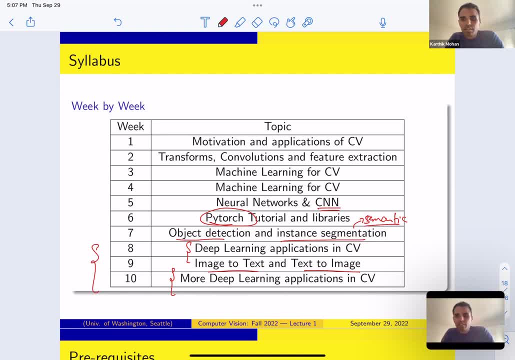 So again, this piece is a little bit flexible and fluid Depends on how we are progressing through the quarter. So we have a little bit of flexibility here to advance to the topics based on where we stand. But if we have time we'll look into more deep learning. 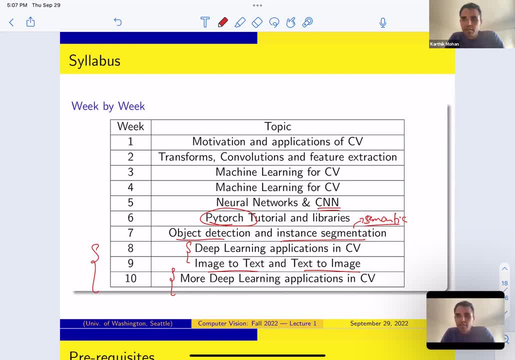 And then we'll look into some of the other applications and computer vision as well. Yeah, Okay. so that's a rough breakdown And obviously, along the way we'll be covering a lot of algorithms and we'll be going into some of the math as well. 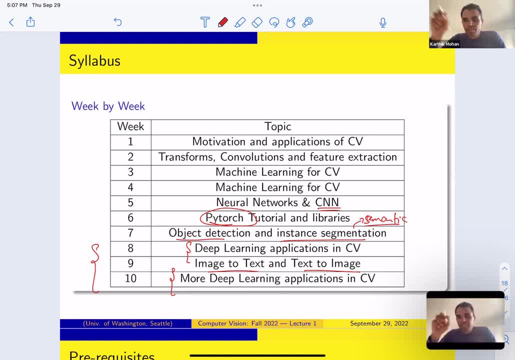 So the assignments will actually give you a lot of the details into any one of these topics. So doing the assignments is the key to learning right. Lecture is probably, I would say, 30%, but you need the 30% so that you can get the 70%. 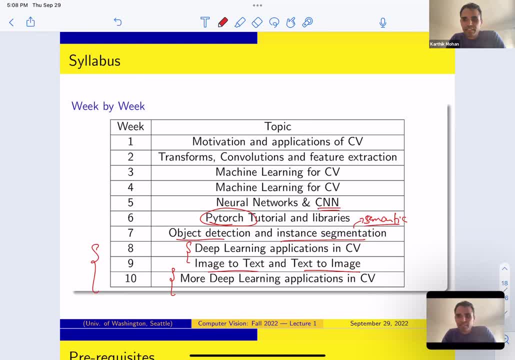 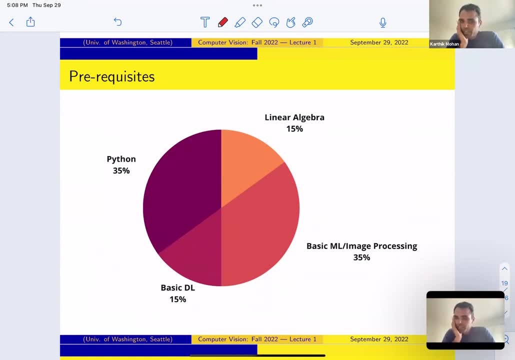 in your assignment. All right, That's the way I think about it. Okay, so some prerequisites for this course, which, if you are missing or you need to refresh, that's okay. I believe most of you should be fine, but if you think it's overwhelming, feel free to reach out. 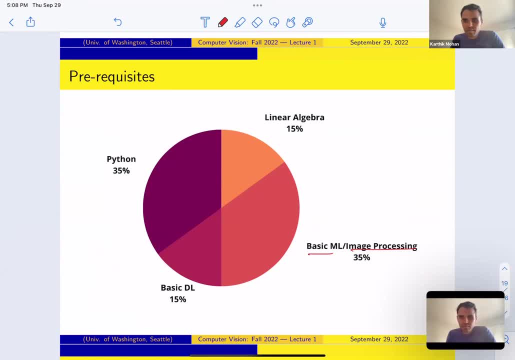 So some basic machine learning and image processing, Some combination of this. Maybe you have background image processing, that's great, they'll be good. Or if you have some basic background machine learning, that's also good. 63 00ramm. 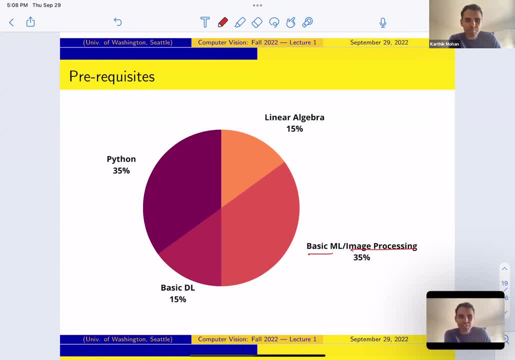 Them exam face ore f? 처ch. but being that then a little bit over, if you don't have background in either of them, you may have to catch up uh quickly in the first two weeks. right same thing with python if you if you haven't um been exposed to python at all. 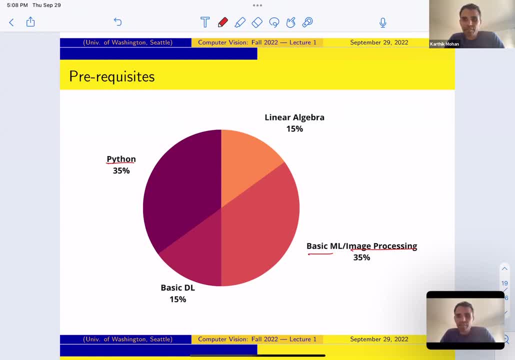 then i would start right away, like start learning python right away, because that's going to be our staple diet in this course. um, some background and deep learning is going to be helpful, but not required. um, so this is helpful. um, linear algebra, uh, yeah, i think in the context of 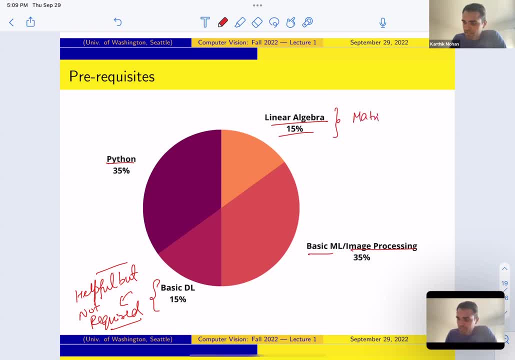 i am. i'm hoping most of us are good with matrices and you know matrix algebra, but if not, again you may have to catch up on that um. so yeah, this is kind of like the breakdown on prerequisites, um, but if any of these areas like stand out or is something that you need to catch up on, i would do that in. 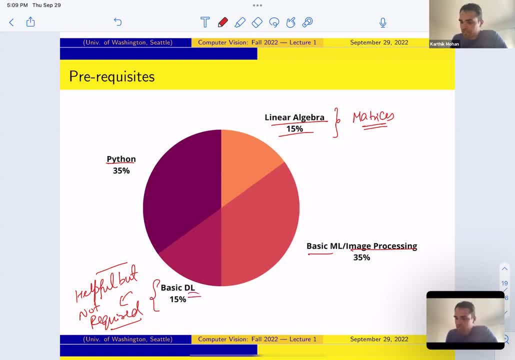 the first three weeks, um, except for deep learning. so deep learning we will cover a little bit later, but the other three, if you think, oh, oh, really, python, okay, i'm not sure- then i would start right away, uh, so that you can actually have a good time, uh, in this course, okay, 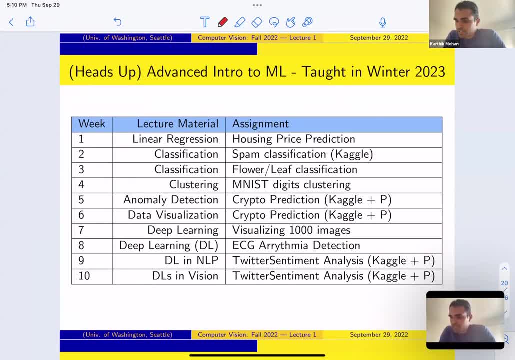 so, uh, just a heads up, um, uh, plug-in for next quarter. so, if you want to start your 85th and passing the new year in in visa ى онный, uh, this is, uh, this is what i taught last or this year or the previous academic year, which was winter 2022. uh, i taught this course and this was a breakdown. we looked at uh kind of a lot of breath in machine learning, so linear regression, classification, clustering and only detection, data visualization, deep learning in NLP, deep learning and vision, deep learning in general, and a lot of Kaggle contests across different applications. so people found it really fun to go through this course for different courses, just to call anything. 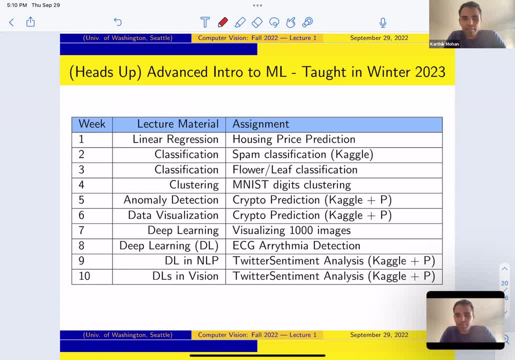 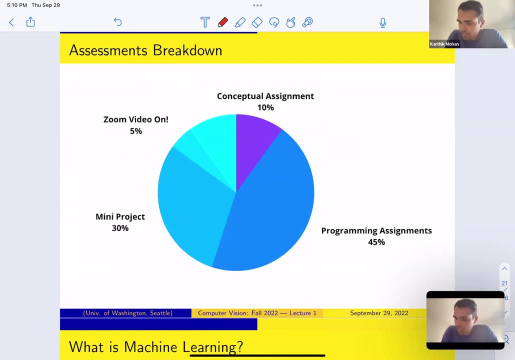 uh, through the assignments and, um, you know, understand machine learning better. so if uh- and this is coming up next quarter, so, um, you, you might, even if you're interested, you might as well take this uh next quarter, okay, okay, let's get to assessments breakdown. um, so i've not done this before, but i want to give five. 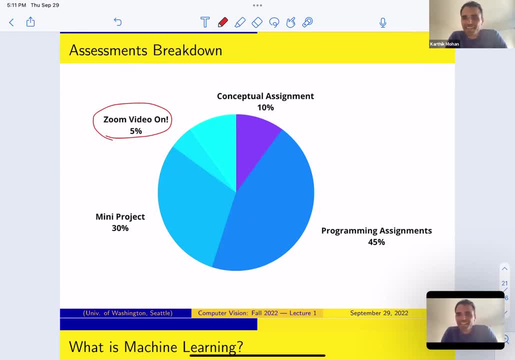 percent to keeping your zoom video on um, because i've requested people to keep their zoom video on in the previous courses and, uh, people weren't taking it so seriously, so i'm just going to put it here. how are we going to monitor it? i don't know, but someone will be monitoring it, maybe ayush. 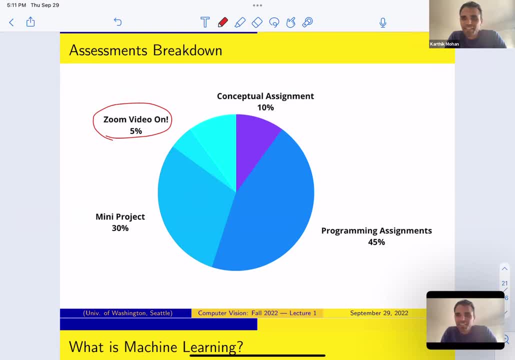 or you know, fatweer will be monitoring it and adding it to your grade. but it's a very easy five percent. just turn your video on and you're good to go right. um, so don't ask me if you have a few lectures that your videos are a few lectures are your. 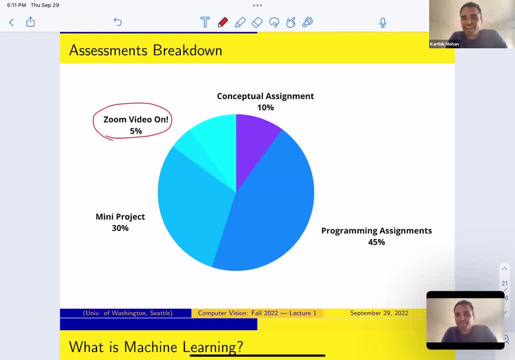 videos on. what's the percentage? i'm not going to answer that question, but uh, you know, just keep your videos on and you'll have a good time. um, we'll also have a conceptual assignment. uh, just to cover some concepts in computer vision. um, may not be as frequent as a programming assignment. 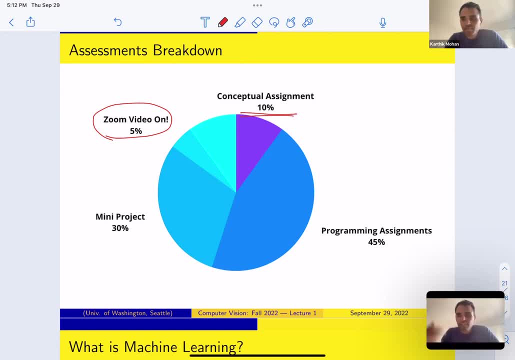 but we'll have one every two or three weeks so that your concepts are also clear. so we'll have some interesting questions in there: um, maybe two, three questions that you can just ponder on and answer. um, so that'll be conceptual assignment 10. bulk of your grade is going to be: um, oh, this is not adding up. 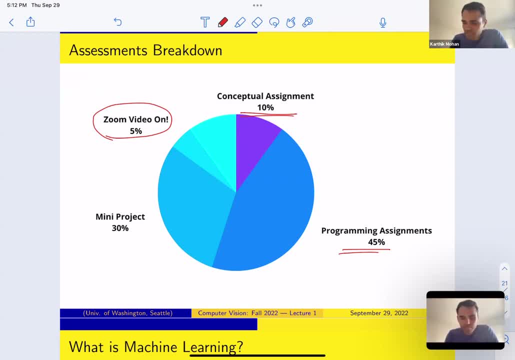 100. so there's something missing. okay, we'll, we'll uh come back on this. it's adding up to 90.. there's something missing here, okay, um, what is missing? oh, i see, i see, i see, yeah, there is in class exercise. that's what's missing. so we'll have some in-class exercise as well. so, uh, in the zoom session or in. 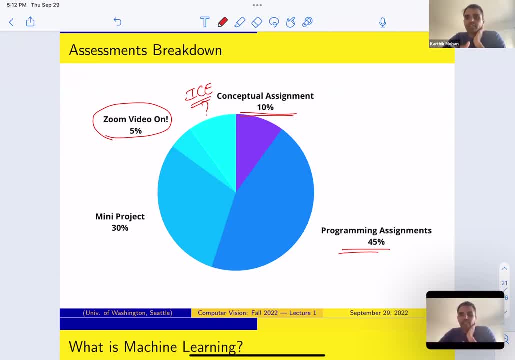 class on tuesday, there'll be some in-class exercise where you can just like: uh, you have a question, you'll have a couple of minutes to answer it, just go through it and answer it and then record it on a poll and then that'll get, uh, about 10 percent of your grade, right? um, this is 10 percent, and then 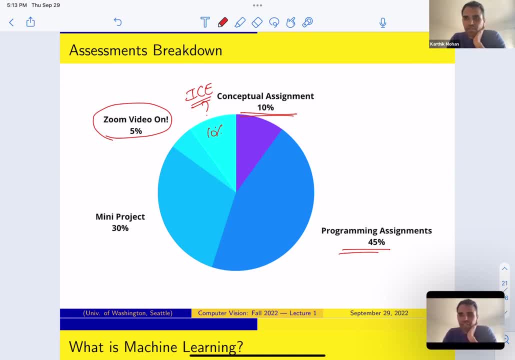 we have programming assignments. this is going to be bulk of your uh, grade 45, percent of your grade 45, and this is where you're going to learn the most. um, just, you know, running through all of that, running through that pytorch assignment, running through that, uh, you know, convolution assignment. 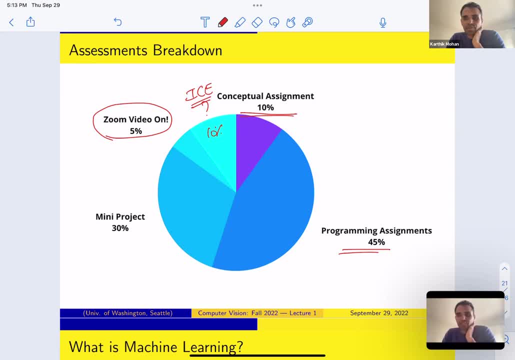 running through your deep learning assignment. that's where you're going to learn the most, so we have the bulk of the grade there and these two are connected. so we're going to have some mini projects, uh, and we're going to have some assignments, so mini project is basically 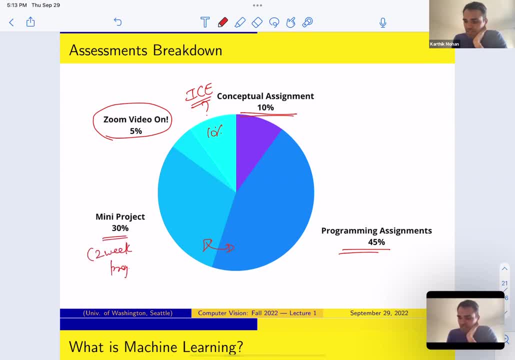 more of like a two-week uh project. so uh, programming assignment is one week, so that's the only difference you can say. but also with a mini project there is more level of complexity and more level of detail that you will go through in the mini project, right? maybe, for instance, um image to text might be a mini project, so we'll. 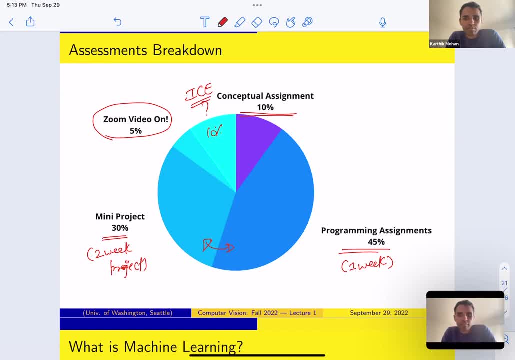 put a kaggle contest on image to text, and then you'll work on your computer vision model, you'll work on your nlp model, you'll piece it together that all of those moving pieces are going to take some time, uh, and then obviously we'll have a kaggle contest. 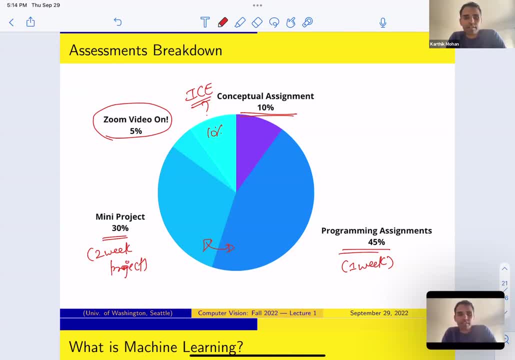 you want to uh see how you're performing um, and it's fun. kaggle contests are something we've done in the past. how many of us have done a kaggle contest before um in some previous course or show fans? no one, two, three. okay, yeah, if not, you'll get exposure to a kaggle contest in this course. 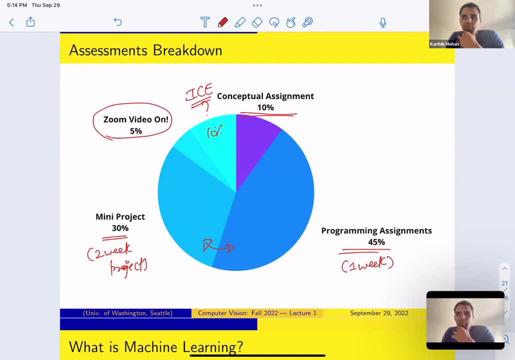 it's really fun, um. it's more than an assignment because you have your team score, but you also see other people and how they're doing and it's a friendly competition, uh, to do better on some metric um. but it's also a motivation to understand material better, so people really get hooked. 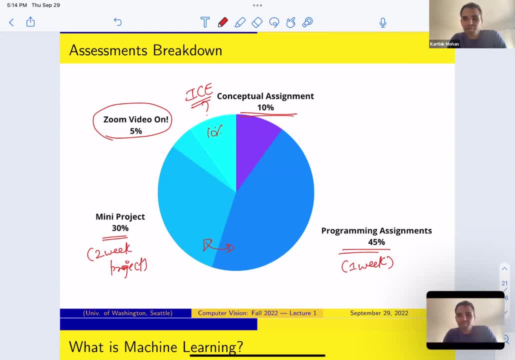 on to the kaggle contest because they want to get to the top of the leaderboard, but it's a more of like a motivation to learn better, so i would focus on the learning and then you'll obviously do well. so, yeah, so we'll have many projects as well. maybe a couple of mini projects. 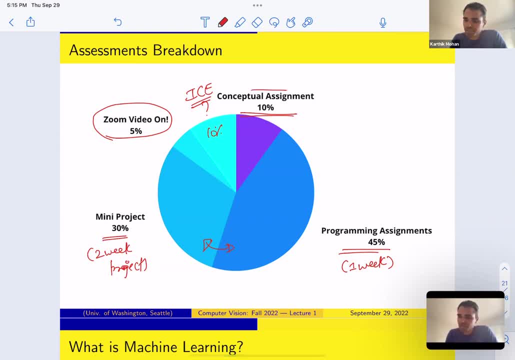 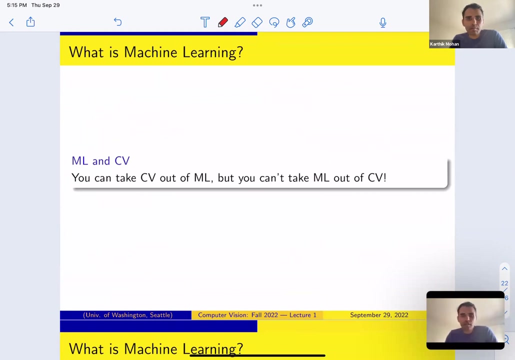 programming assignments and then we'll have a couple of conceptuals and in-class exercise will happen. every lecture, right, okay, any any questions on this? okay, all good, all right, so so that's kind of like: uh, logistics and setup. maybe we'll take a five minute break, um, you know, i think i've found 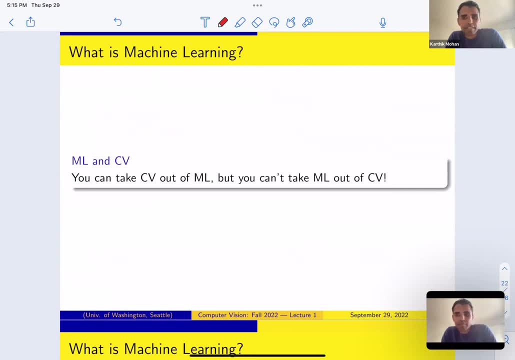 this in the past as well- that i sometimes ask do you need break? and people say no, and then after half hour they're like really tired or distracted. i'm like what's happening? so then i realized, okay, we didn't take a break, so let's take a five minute break. 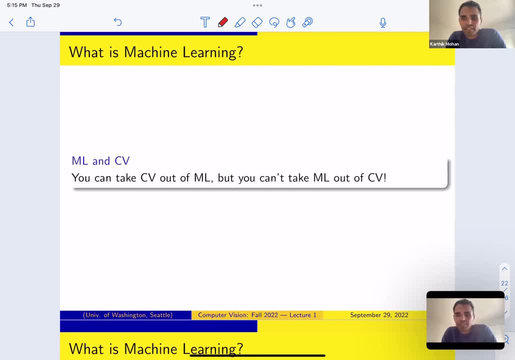 and then we'll come back and then we'll maybe go for another 20 minutes today. yeah, all right, uh, let's get started. so, um, machine learning is fundamental to computer vision, right? so we'll just, uh, i think today we'll just kind of touch upon these connections and go a little bit on a conceptual understanding. 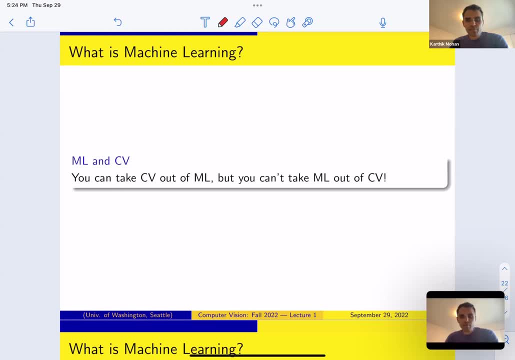 of machine learning. um, something i find people have found useful in the past courses i've taught as well, uh, is to kind of understand machine learning on a more high level. um, before we dive into the details of it. so, ml and cv, you can take computer vision out of machine learning, but you cannot take machine learning. 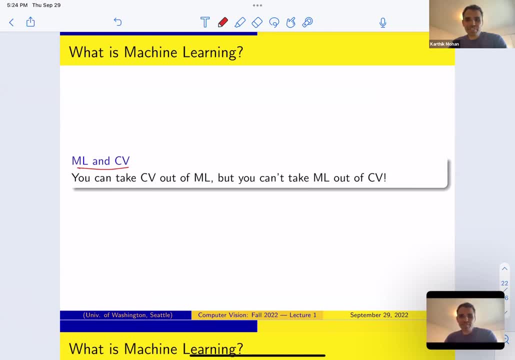 out of computer vision. so what does that tell you? it tells you that machine learning is foundational for computer vision, but it's much more broader. there's many more things happening. i mean more applications, machine learning. but one of the fundamental applications of machine learning is in computer vision, right? 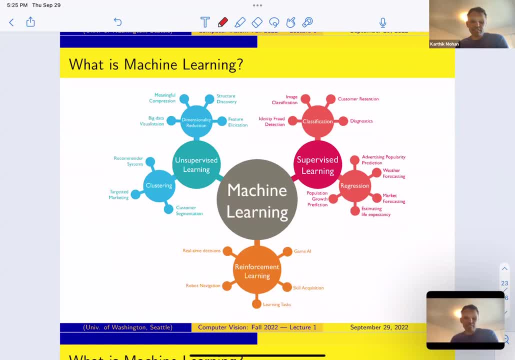 so what is machine learning? uh, it's a lot of things. it's, uh, unsupervised learning. it's supervised learning, it's classification, it's recreation, it's dimensioning reduction, it's clustering. you know, it's so many things. so that's why we have a whole course in winter 2023 on 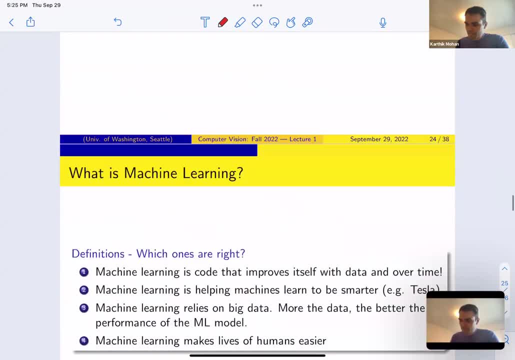 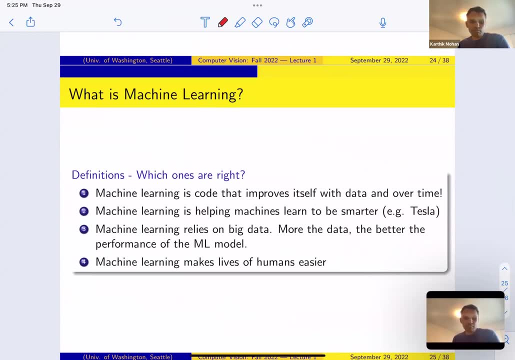 exactly this. but if you, if you, if i, were to give you some definitions of machine learning and ask you which of these are right, uh, what would you answer? just take a look at this. maybe third one, sorry, maybe third one, third one, okay, yeah, maybe all of them. maybe all of them okay. 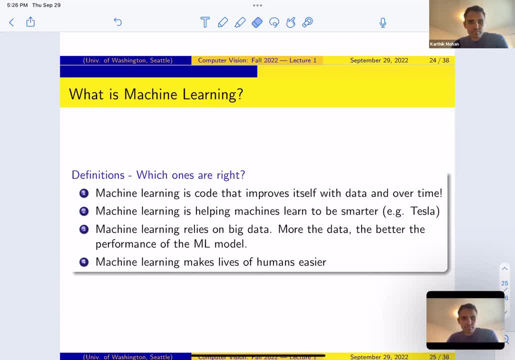 okay, any more answers: a second, one, third and fourth, one third and fourth, one second, one uh-huh okay, great, yeah, so yeah, there are multiple answers to this. um, machine learning is code that improves itself with data over and over time. yeah, in general it's true, but there can be exceptions, so all these statements come with. 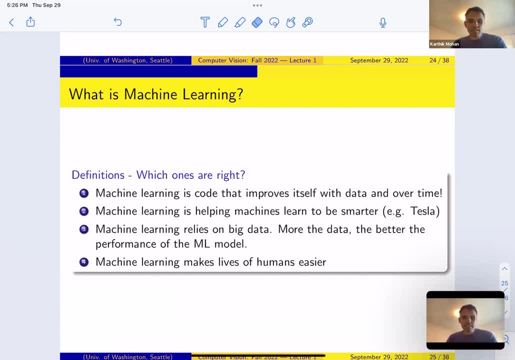 some exceptions. uh, it's not true that more the data, the better the machine learning model. um, more the data, better the machine and model to some extent, uh, to the extent where it's useful, but after a while it may not be useful, so you may not improve over time. again, depends, uh, so a lot of. 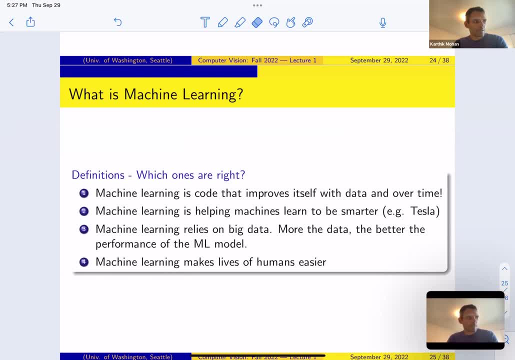 okay, that's so. but the first, uh, first- statement is true: machine learning is a software that is smart. you can say in that way, a lot of software is like designed to do something specific and then it executes it and that's it. but machine learning can improve itself with more data. so that's true in general. 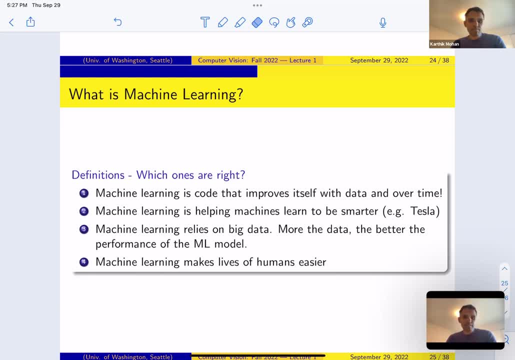 but there are exceptions. machine learning is helping machines learn to be smarter. yeah, that's true. uh, machine learning relies on big data. more the data, the better the performance. again, this is connected to one. you cannot. yeah, it's a little bit of an ambiguous statement. it is true in some cases. it is not true in some cases. 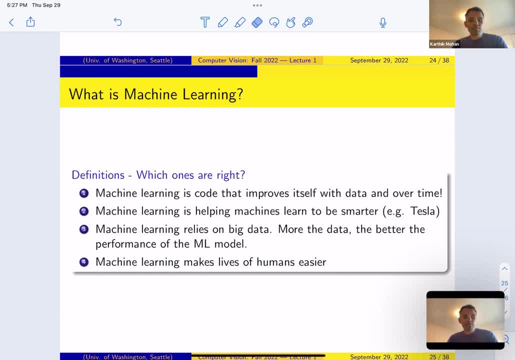 um, more the reader, the better the performance, yeah, so we have to be a little bit careful with this. if you use this principle and then you, you're working at a company and you say: more the data. i don't have enough data, i need more data, more data, more the person your manager is. 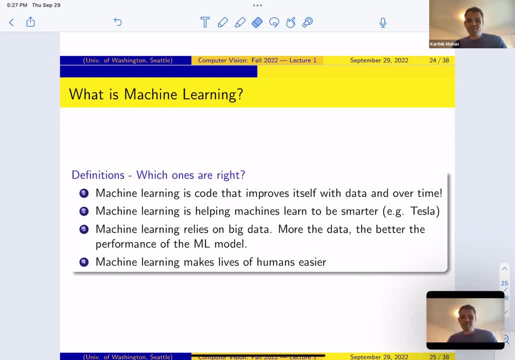 going to be like: uh, i think you're not doing a good job. i've already given you enough data. tell me why you need more data, more data. they're going to ask you back: why do you need more data? can you please tell me? and then i: 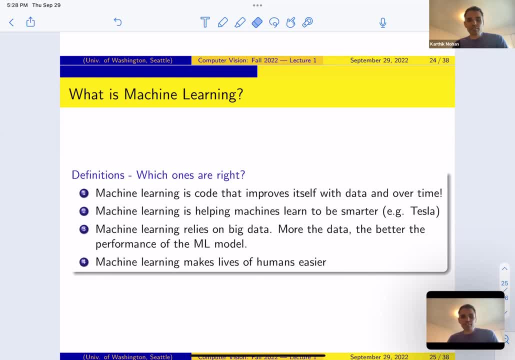 will give you more data or get more data yourself. so you need to be able to justify why is more data better for your machine learning problem. so having that understanding is important, right, um? and let's see, um, if you were to graph it. um, so this is learning, and then this is maybe the data access. 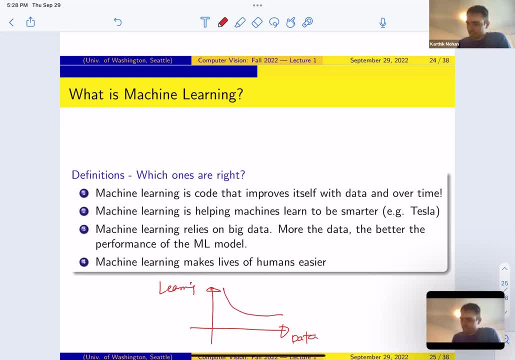 there might be some flattening. that happens. so yeah in. if you're in this regime, more data is better, right, but if you're in this regime, um, you may not learn from more data. so what that tells you is: you need sufficient data. whether you need more data or not, you need sufficient data to be able to build a good 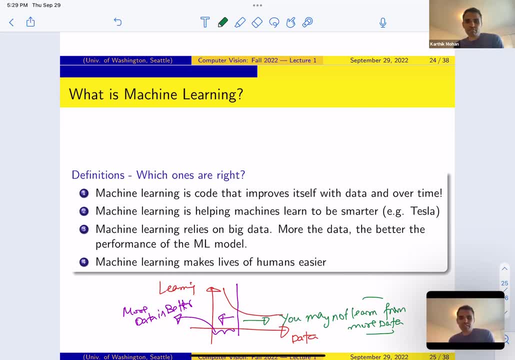 machine learning model and what is sufficient varies from problem to problem. uh, for certain problems, um, simpler ones, like spam classification or um, you know, you have image classification or simple uh classifications of this data. you might do a problem with this data from data scrub society. okay, if you looked at this classification, you have an estimated step size without databoxing in one picture. 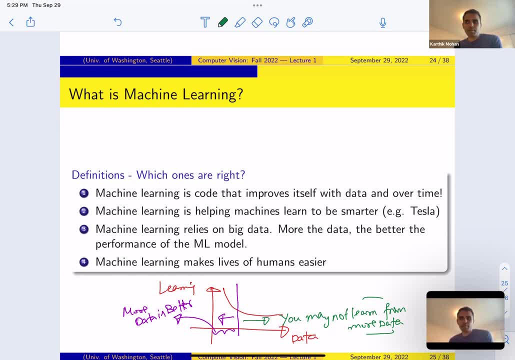 classification problems, like you need sufficient data and that's good enough. but for uh things like you want to do uh text to image, or you know, image to text, or one of these complicated uh you know computer vision problems, there's usually not enough data. so that's where you would say more data is better, because you're not hit that sufficient mark you. 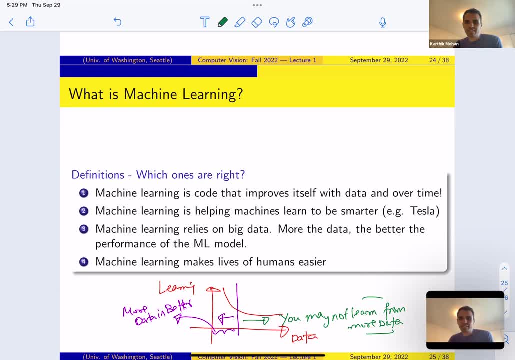 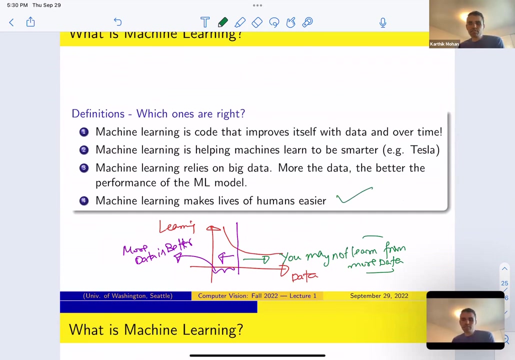 don't have enough examples, so more examples are usually better in that scenario. so we cannot really put a blanket statement, but understanding the context of which problem space you're dealing with can help you make these statements more accurate. right, great, machine learning makes lives of human easier. yeah, yeah, so most of what we do in machine learning is not meant to complicate. 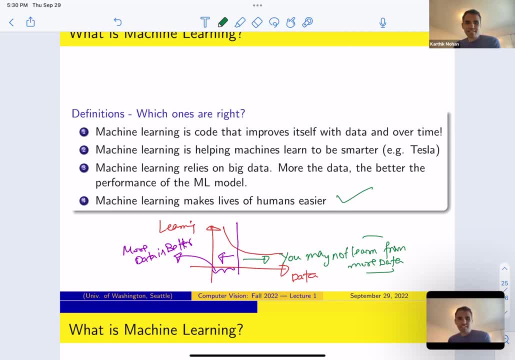 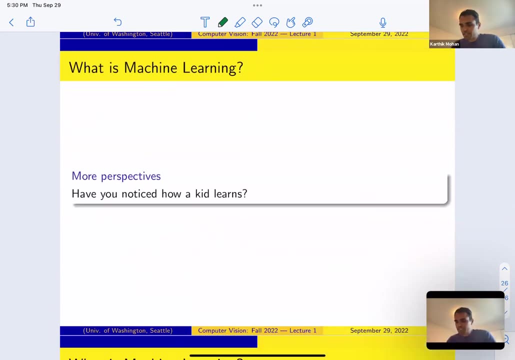 lives if, if it is complicating lives, then, um yeah, find a better application for machine learning. but if you know your problem space, you're dealing with more complicated problems, then you should. It can make lives easier, right? So that is for sure. Okay, what is machine learning? 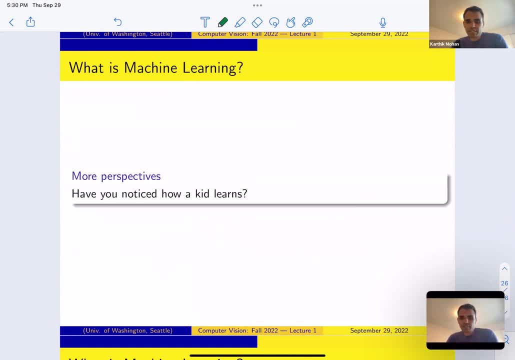 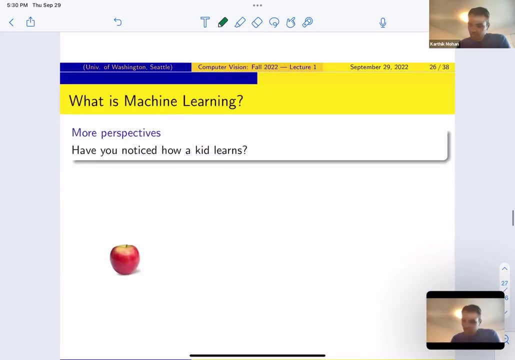 So I wanna give you a high level perspective on this, and I found this to be very instructive in previous classes as well. So have you noticed how a kid learns? So you show a kid, let's say a three-year-old kid. 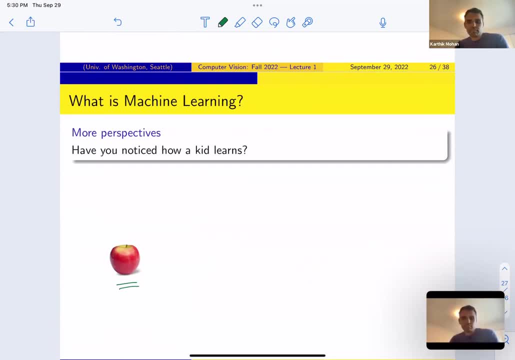 and you say: can you tell me what this is? And the kid is like I don't know. And you say: this is an apple, okay. So the kid is like: okay, this is an apple, I got it. 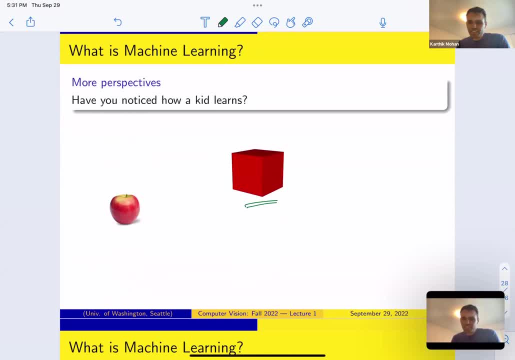 And then you say, what is this? What do you think the kid is gonna say? I don't know. It's gonna say, oh, that's an apple, because it's red Right, if that's what the kid got from the apple. 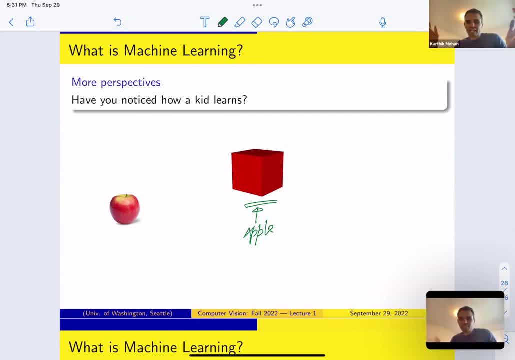 is that it's apples are red, So apples are red, so this is red, so this is an apple. Right, Right, Right, Right, Right Right. Very basic logic. Then you say: no, that's not an apple. 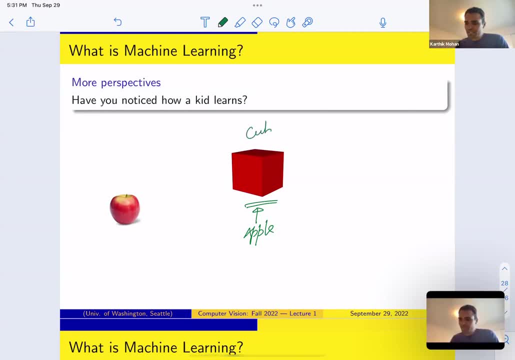 That's red, but it's a cube. okay, Because it looks it's not round. Apples are round, okay. So then the kid is like: oh, if something is round and it's red, that's an apple. 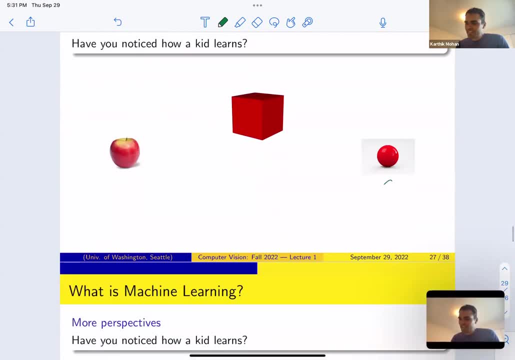 Yeah, that's fair right. Then you say: what is this? You're like, ah, that's easy, That's an apple. Say, oh wait, but why do you say it's an apple? Well, it's round. 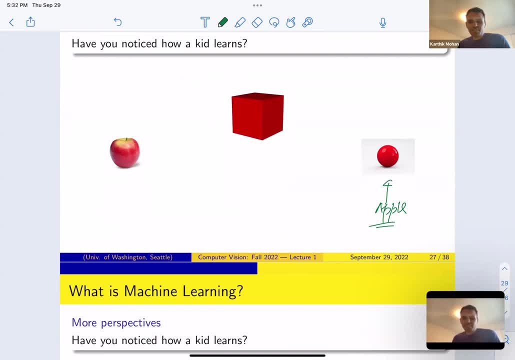 And it's red. That's what you said. So you say no, no, no, no. it's round. Yeah, but it's not exactly like perfectly round. It has to have a stem and it has to have this kind of a shape. 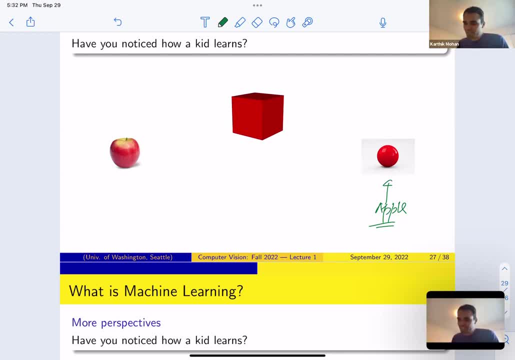 Then it's an apple. You say, oh, okay, So let's go back here and then maybe understand that there is some kind of a shape going on there And that's an apple. Okay, Then you say: what is this? 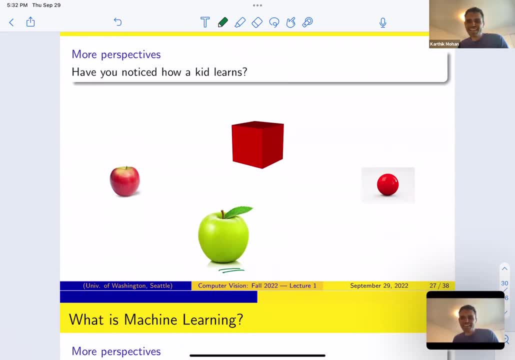 And the kid is like: no, that's not an apple. Why? Why would the kid say it's not an apple Because it's not red. Because it's not red? You told me apples are red and they have a certain shape. 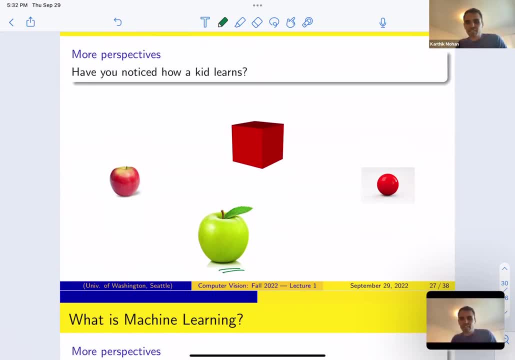 and it's kind of round. Now you're showing me something that's green. Obviously it's not an apple. Then you say: well, you know, apples can be green too. Then it's like: oh, kid is like oh. 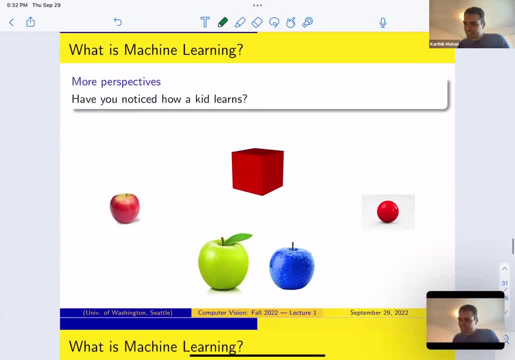 I think I learned something new today. And then you show this, Say, is this an apple? The kid is like, oh, I think I learned something new today. And then you show this, Say, is this an apple? The kid is like: yeah, that's a blue apple. 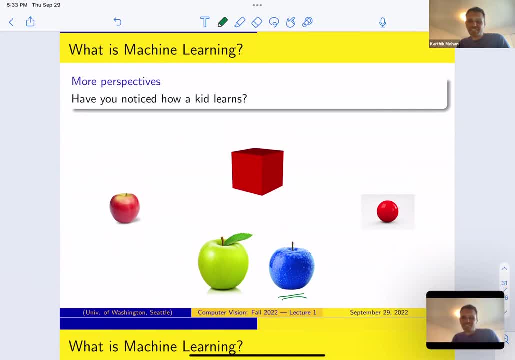 You say: no, there is no blue apple. That's imaginary. There's no such thing as a blue apple. Now. now the kid is confused. So this is how machine learning sometimes is: The more features you expose, the better your understanding of what something is. 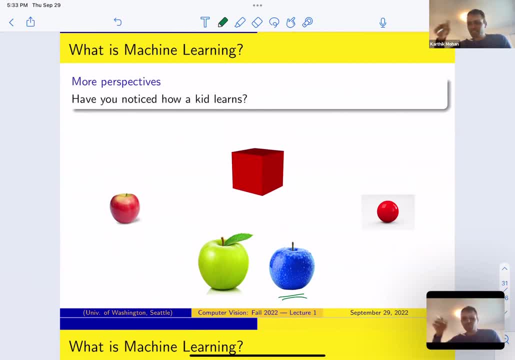 or you could also say: your understanding shifts. That's: this is an example of more data is better, Because if you just give me one example and say this is an apple, I might just pick up on it and say this is an apple. 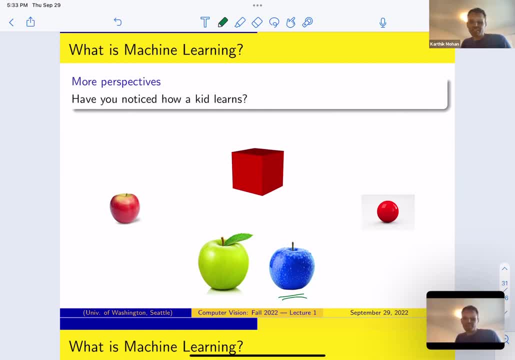 I might just pick up on the color and say, oh, red color objects are apple, Because you just gave me one example. But then you gave me two, then I picked up something else. You gave me three, I picked up something else. 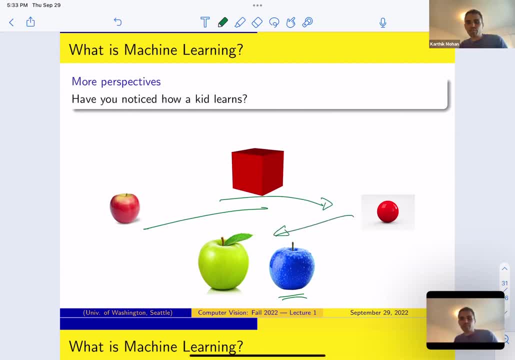 Then you gave me four. I picked up something better. So maybe after four or five examples I am now after five or six examples. the kid is hopefully good with apples, right? So this is how the human brain learns: with examples, but good examples. 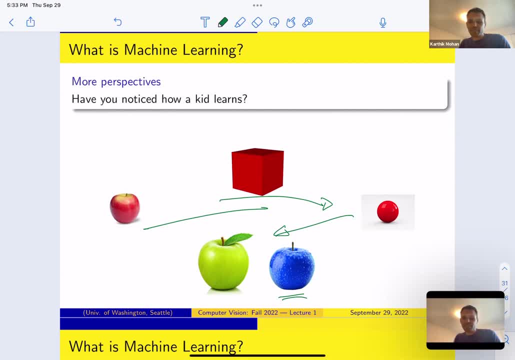 You should give enough good examples that you can actually learn. So good examples are able to explore different features. So if you look at the features here, we have color, we have shape. anything else? Yeah, color is easy, but shape is complicated. 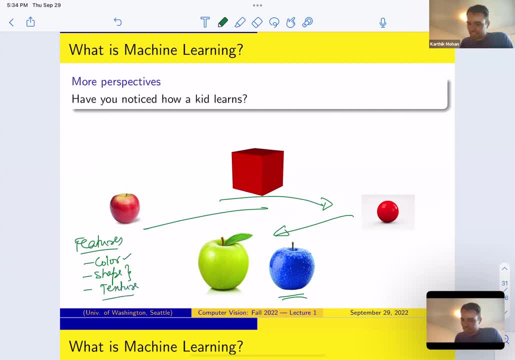 Texture. yeah, John right, Texture is also complicated. but even shape is complicated, Because you have to like: what's the shape of this? If someone says it's round, well, this is round too, Then you're like: oh no, no, no. 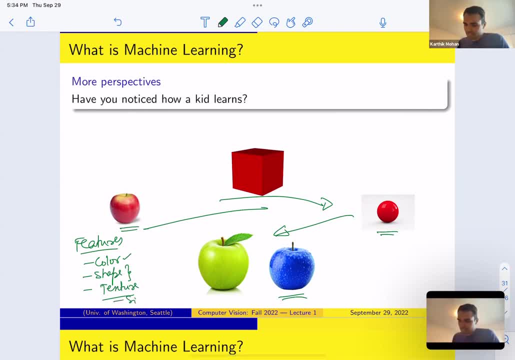 So size, yeah, size also. What if you have a smaller sized apple? right, They say it's not an apple. So again, it's luster. yeah, So so many. now we're able to say something more. 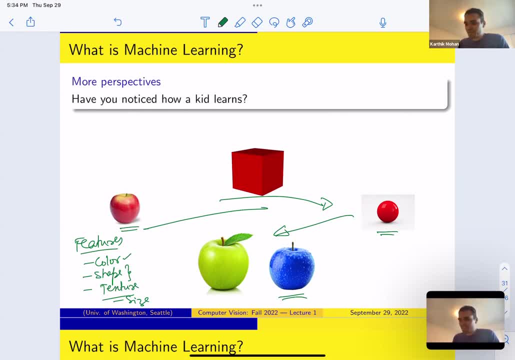 Describe things a little bit more, a little bit better, But you can describe all of this and still not be able to pinpoint an apple if you've not seen it before. right, It's like describing an elephant. It's like, oh, it's long. 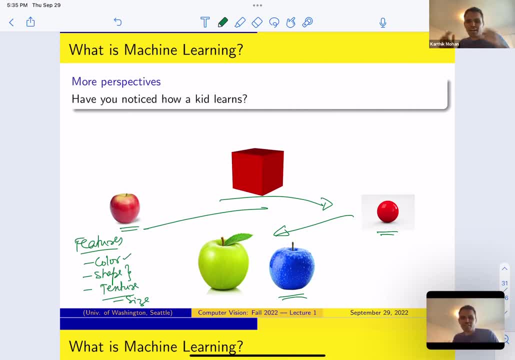 It's wide. Oh, is it a house? No, it's not a house, It's an elephant. It's black. You're like, oh, what is it? So it's sometimes it's hard to just describe the features and understand exactly what the object is. 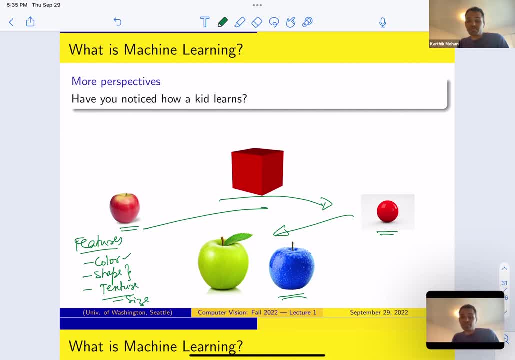 So that's what a machine is trying to do, is you're just giving these features and telling it: hey, figure out that this is an apple or not. So this is a very, very simple example, but very powerful in understanding how exactly we 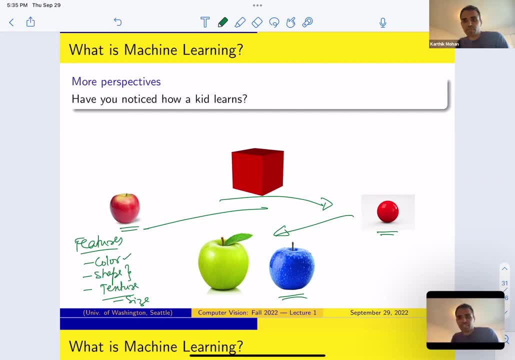 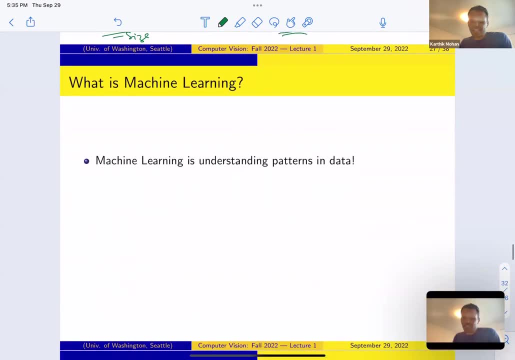 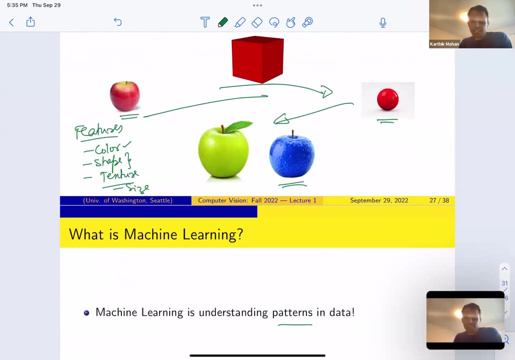 learn as humans and therefore how a machine could learn better with more data. right. So machine learning is understanding patterns and data, right. So, like we said, here there is some texture, There's some- I think someone said shine, or what is that? 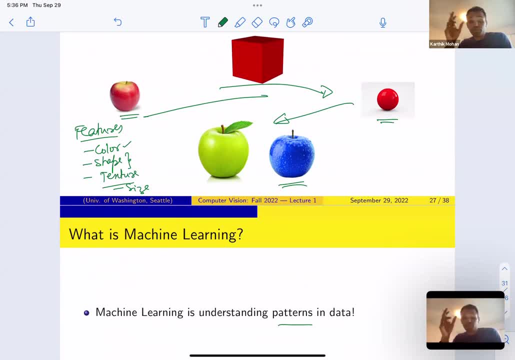 Luster: yeah, There's a luster to the apple, So you look for the luster. These days people put some wax on the apple so it shines a little bit more. So luster, it looks more attractive. But yeah, so you're looking for certain patterns in the data. 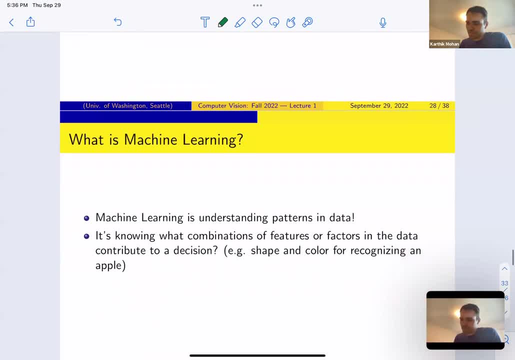 to understand what the object is or what you're trying to do right, And understanding patterns is Learning right. What is learning? Learning is basically understanding patterns. Anything. take any problem: computer vision, Image segmentation. OK, there is a pattern. 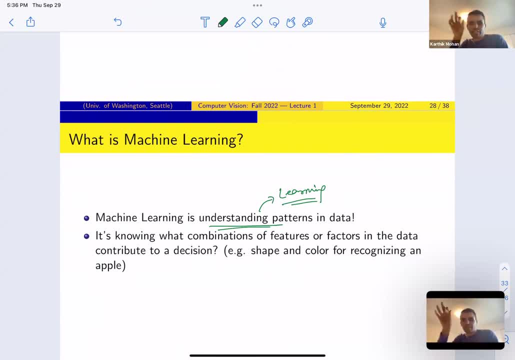 There is a pattern of a sheep that looks like this And I'm trying to fit it in the image And then, if I fit it, then I say it's a sheep. So you're again. it might be a complex pattern. 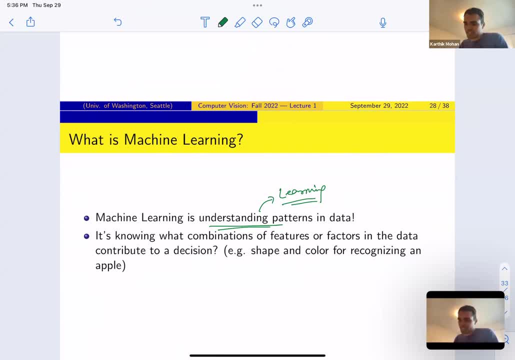 but it's still a pattern. So understanding patterns and data is machine learning right, And it's also knowing what combinations of features or factors in the data contribute to this decision. So sometimes you have a lot of data but you don't know which pieces of the data. 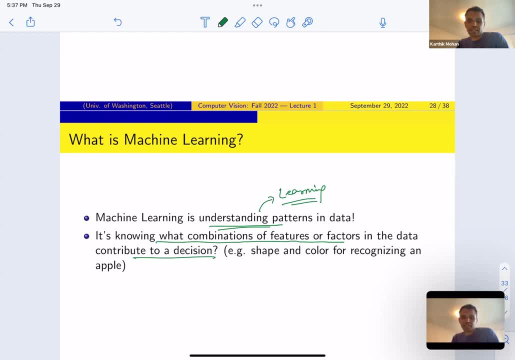 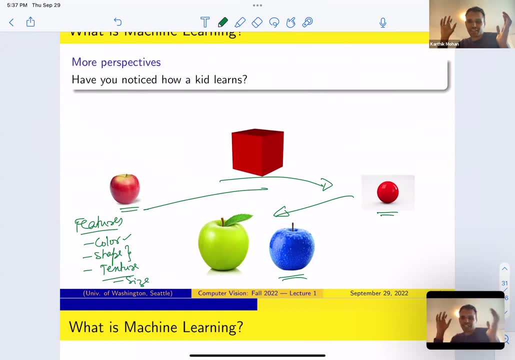 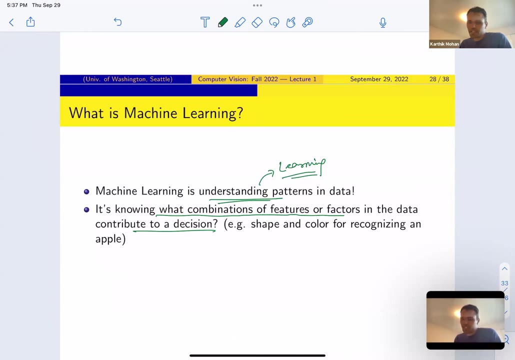 are actually contributing to your decision making, right? For example, an apple. Apple actually has a lot of data. Did you realize that Just a simple apple has so much data, so many features? right, So understanding which features actually contribute to a decision making. 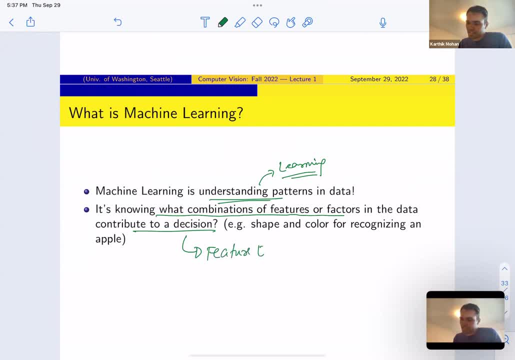 This is what we call feature engineering is building right Building features, Building features, Building features in a way that's actually useful to make predictions And in companies people actually have a whole data engineering pipeline on this- to build feature stores. 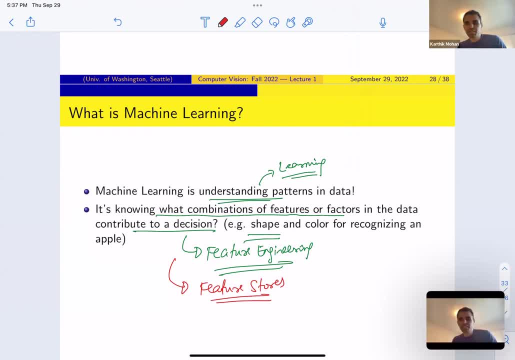 So people say: oh, I came up with a new feature for images And I'm going to upload it to my feature store or to the feature store. Any team that wants to use this feature feel free to download it and use it in your model. 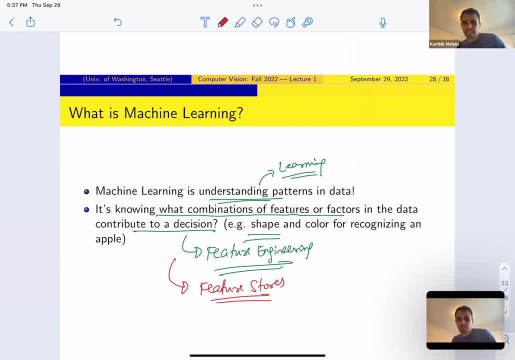 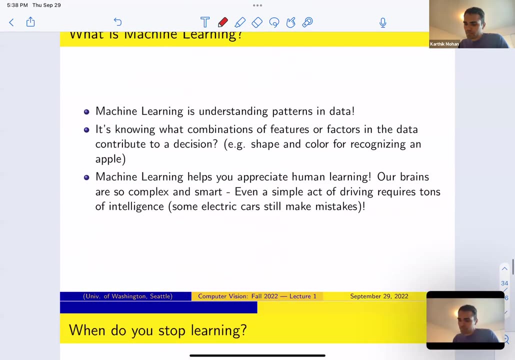 So feature stores are, like now, pretty ubiquitous in many companies as a way of democratizing features that people have worked hard to identify but might be useful for other tasks and other teams. right, So machine learning helps you. Yeah, this is more of a philosophical thing. 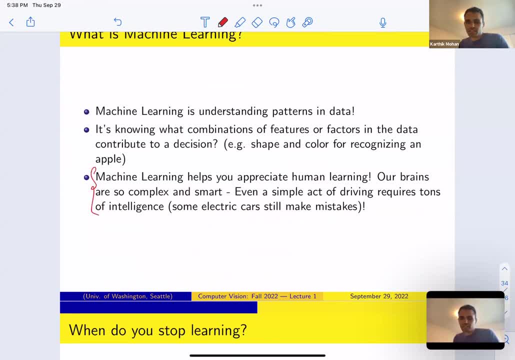 It helps you appreciate human learning. We take our own learning for granted, Like you take a kid for granted. You're like: ah, you couldn't even recognize an apple, But you can do it. So you didn't realize how complicated of a task. 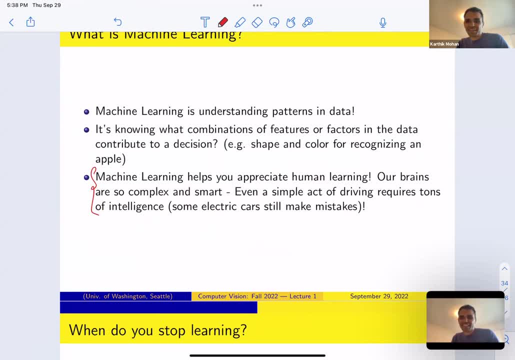 identifying an apple is right. You're like: oh, that's a kid's thing, You can't even identify an apple. But our brains are so sophisticated and smart that we think identifying an apple is not a big deal. But a machine can have a difficult time. 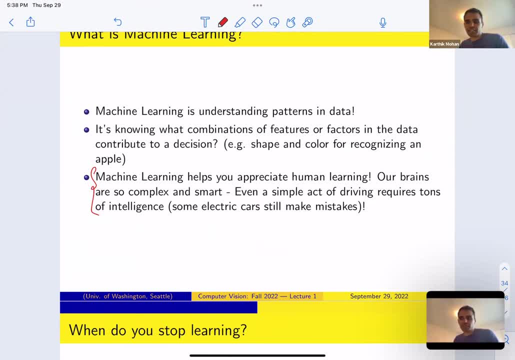 Even now, you apply some of the deep learning methods and it could say: an apple is something else If it has a different tint or a different lighting. you change the lighting, you change the size, whatever you know, And it would say: now it's an orange. 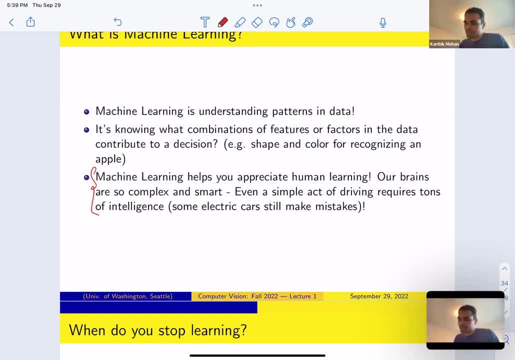 But it was working fine before. So yeah, And let's say driving, you take driving for granted. You're like, oh yeah, you just get a driver's license, you can drive. But a simple act of driving requires tons of intelligence. 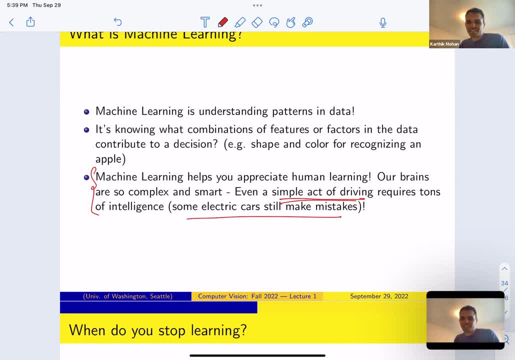 And, yeah, like we know, some electric cars still make mistakes despite a lot of data. So there is some gap between human learning and machine learning that is still not filled Right, Like we, especially with daily tasks. with daily tasks. 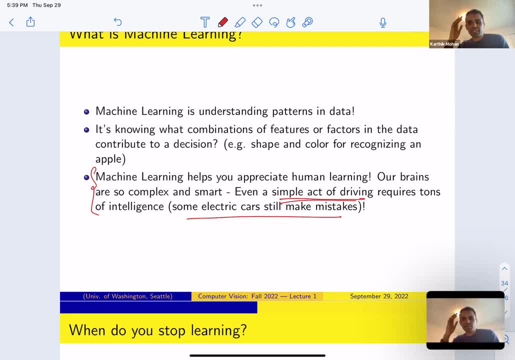 we are really good. We don't make mistakes. But even with millions of data points, machines can still make mistakes. So that's a fascinating thing. We don't need millions of data points and we are able to learn and adapt, But machines might get millions of data points. 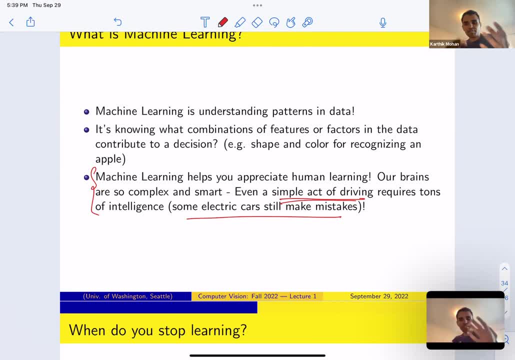 and still make mistakes. So somewhere in the architecture or somewhere in the way a machine is learning, things are not enough Right? So that really helps you appreciate your own brain. Your brain is so like if you think you're not smart. 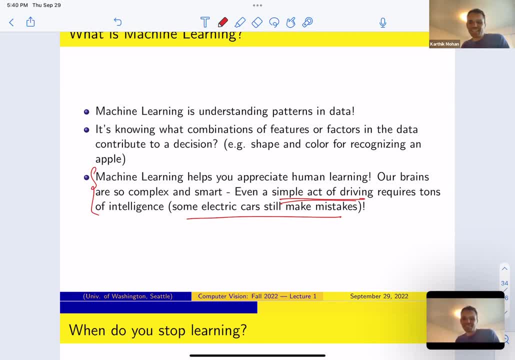 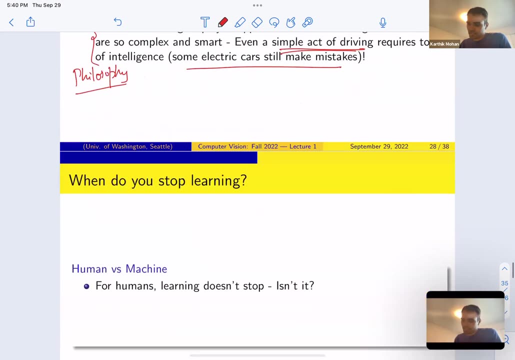 think again: You are really smart to be able to just do daily activities, Just to hear me speak and understand what I'm saying. you're really smart, OK. so that's a little bit of philosophy of machine learning, Right? OK, when you stop learning for humans? 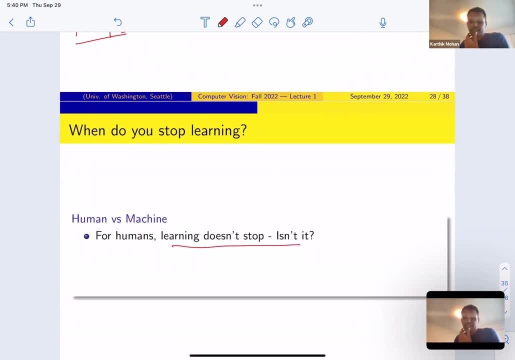 learning doesn't stop Right, Yeah, Yeah, Yeah, Yeah. This is again more in the philosophical dimension. Like we have very complex learning spaces You learn in, like you're here to learn about computer vision. So that's technical. 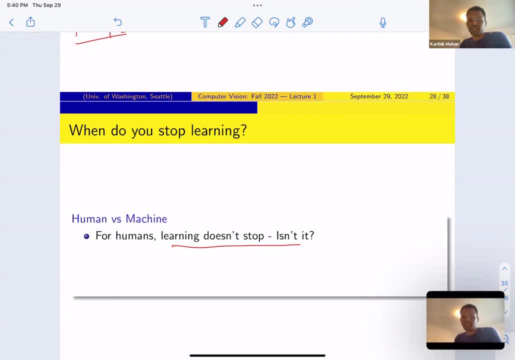 Then you say, oh well, I go back to my life and then I have relationship learning to do, I have to learn how to grow in relationships. So that's a whole another dimension. So for us, learning is multidimensional. 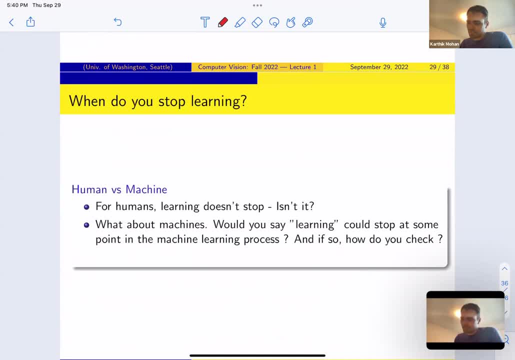 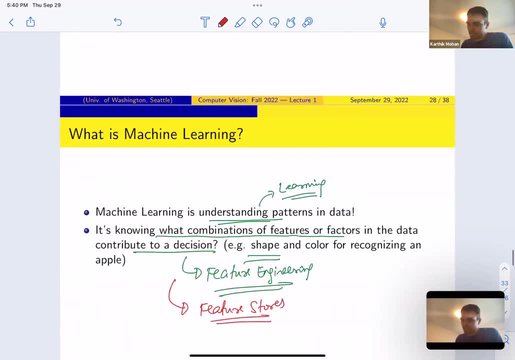 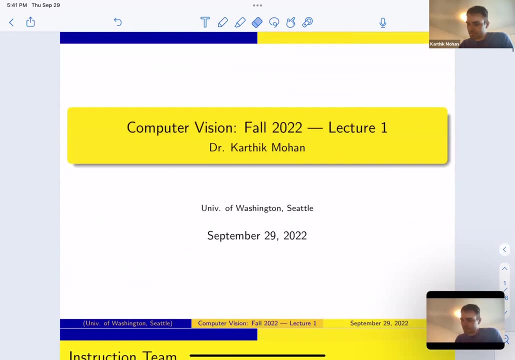 and it doesn't stop. For machines, you would say: learning stops at some point And you can also check if learning has stopped. So this is the graph that we had earlier. Where is that Here? Yeah, there's an example of that. 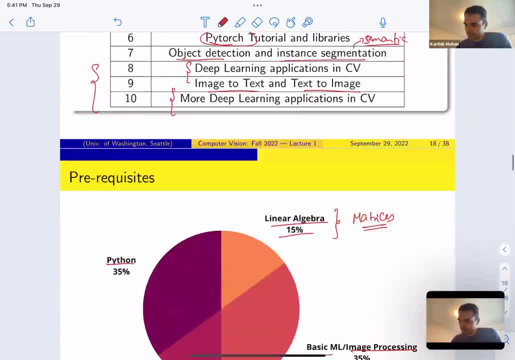 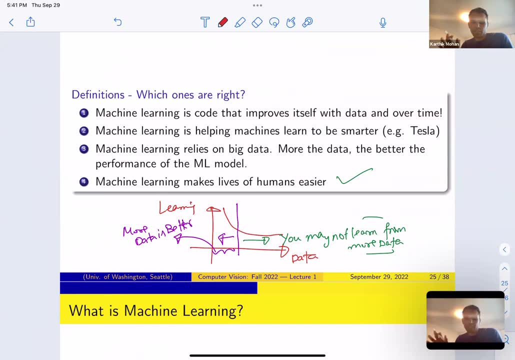 Oops, Yeah, this is an example of how learning could stop. You're feeding it more and more data, but you're not improving the learning. And how do you measure learning? Well, in machine learning we have some metrics like loss function. 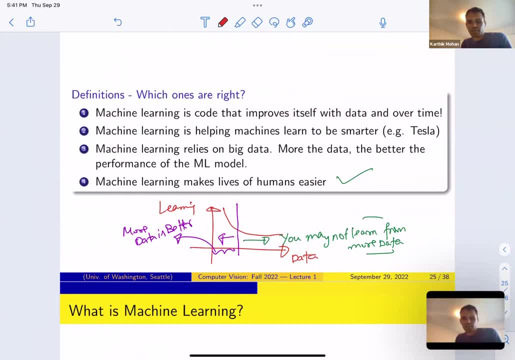 What's that? What's the loss value, What's the precision recall Or what are metrics that you care about in machine learning? It's not improving. You're feeding more data. You're doing these iterations passes through data and it's not helping. 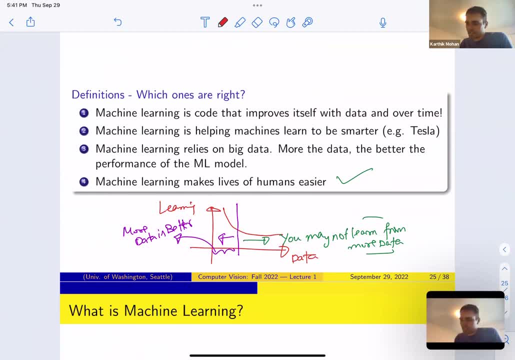 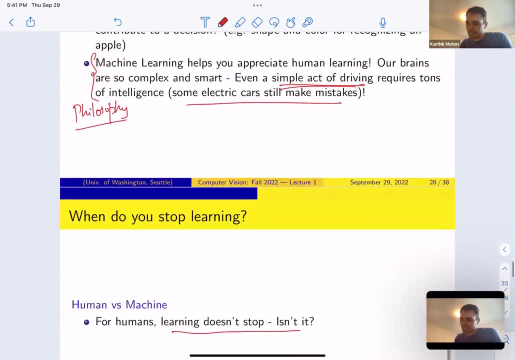 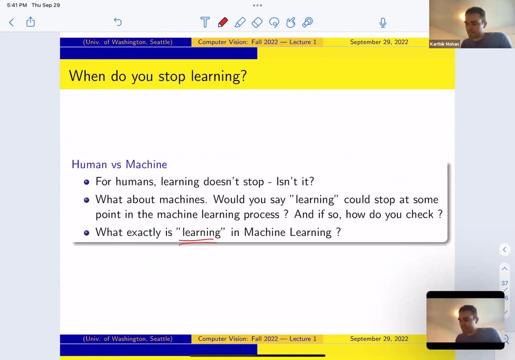 So you say I stopped, I'm not improving. So there are ways to measure if you're improving or you're not learning as much for machines. And yeah, we also covered what exactly is learning in machine learning. It's learning the patterns in the data. 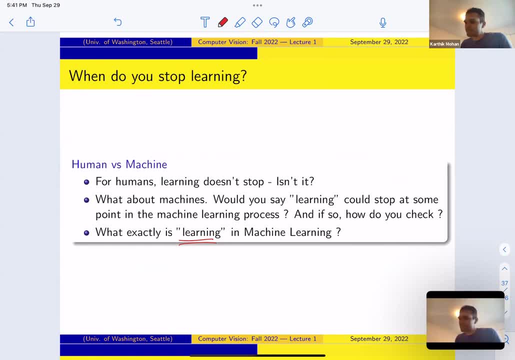 It's learning to make predictions. It's learning to also. sometimes learning can mean understanding things better. So in natural language processing, for example, we talk about semantic understanding. So semantic understanding is saying: I understand what you're saying so that I can respond to you. 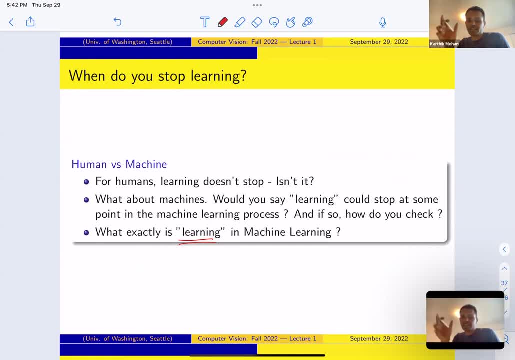 So that's very different from just putting a class to something, Like you said: Can I have a glass of water? You say, oh, you're asking for water and you want a glass of water, OK. Then I say, OK, here's a glass of water. 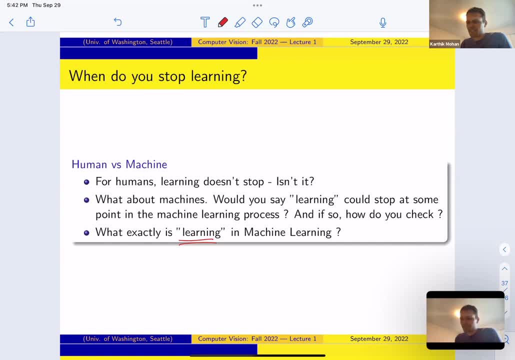 So if I didn't do that, if it was more simple, I would say: oh, you said water. OK, I understand water, But that's it. You don't understand that you want a glass of water, which is very different from just saying water. 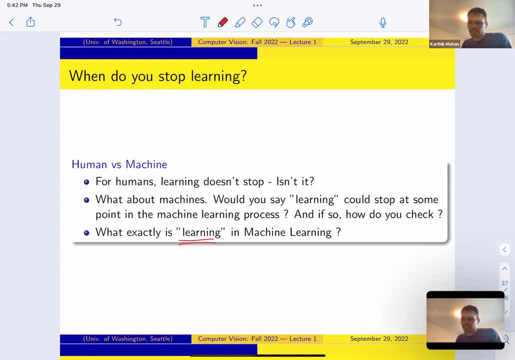 So learning can mean different things in different contexts, And essentially it is enough understanding that you can make predictions. It's enough understanding that you can make smart decisions. So that is what learning in a machine learning context means, And mathematically it's more like you. 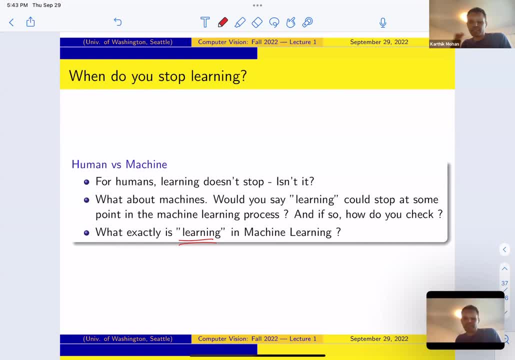 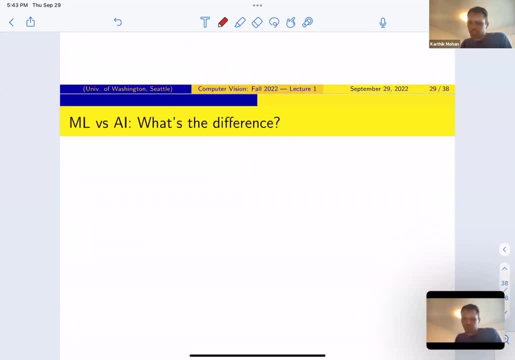 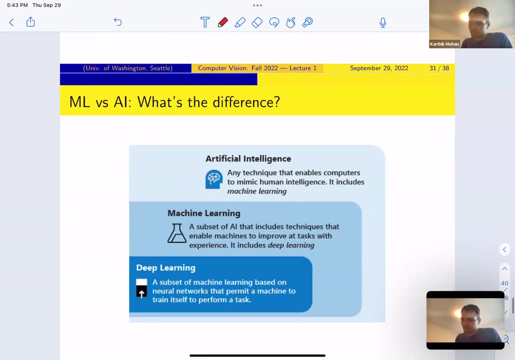 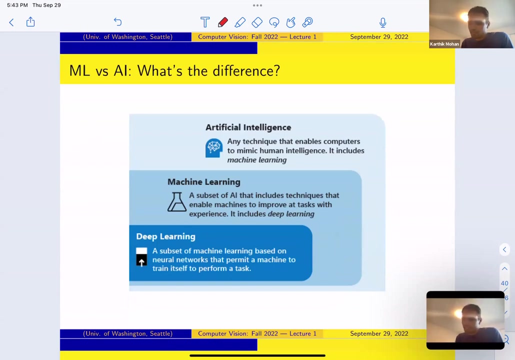 learn some parameters or weight vectors that can help you make these predictions as accurately as possible. Another philosophical thing: what's the difference between machine learning and AI? So this is kind of referenced one take on this. You can take a look. AI is more high level. 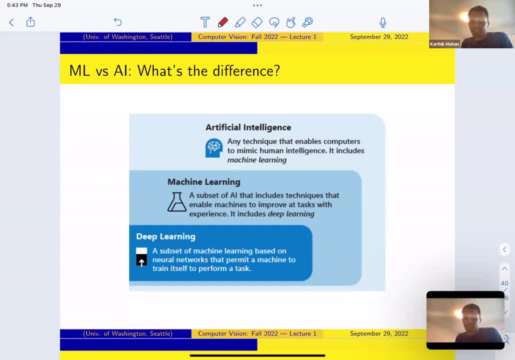 It's like all that fancy stuff. People say, oh, AI is the Transformers, AI is all the things that you see in the movies, Or AI is robots. So AI is kind of the front end of what machine learning can do. It's the things that excites you. 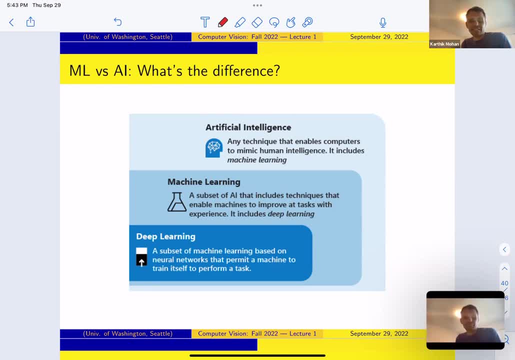 It's like: oh, how did you generate that video from just a sentence? Or how do you generate that image from that text? So that seems like AI. So it is things that enable computers to mimic human intelligence. So that's one way of defining AI. 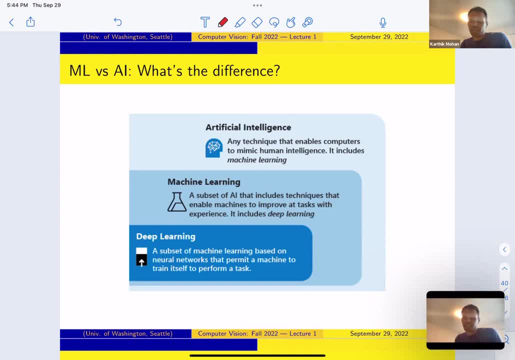 So the classical definition of AI is: can you? There's that Turing test, right. When you have a conversation, you're not able to differentiate if it was an AI speaking or a human speaking. So if you pass that test, you pass a Turing test. 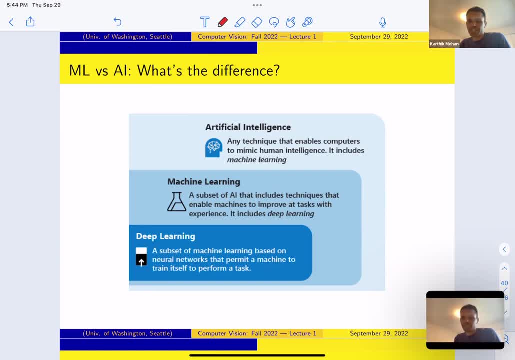 So that was a classic definition that Alan Turing shared on AI. So trying to mimic And human intelligence is like we saw. we are very intelligent And we want to mimic it and automate it so that anything that can help do that, or applications. 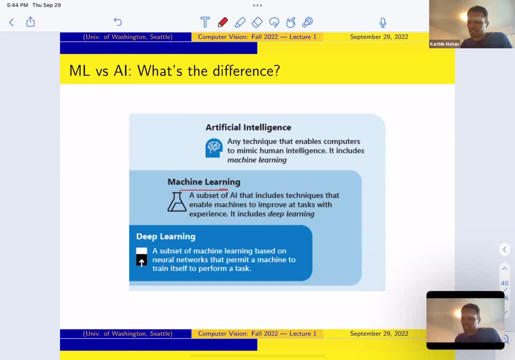 where you do that is AI. But how do you actually do it? You need to do machine learning. Without machine learning, you don't have the tools, You don't have the methods to actually do AI, Then it's more of a buzzword. 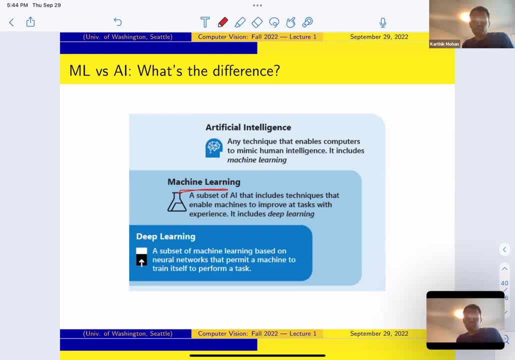 Do you do AI? Yeah, I do AI. I like AI. I like talking about AI. Talking about AI is different from actually working in AI and implementing AI, So that implementation happens through machine learning, And deep learning is a subset of machine learning. 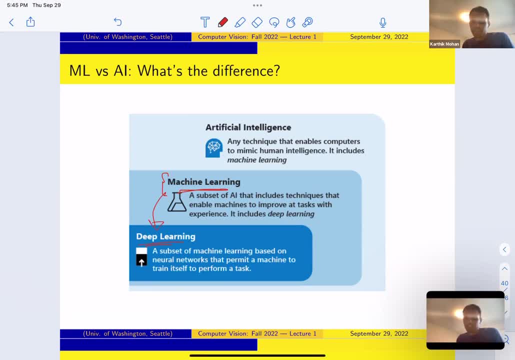 that can do some really high end tasks and have really high performance if you have enough data, And specifically in applications like computer vision and NLP, deep learning is like a staple diet, So these are like it's very well established that you have to do deep learning. 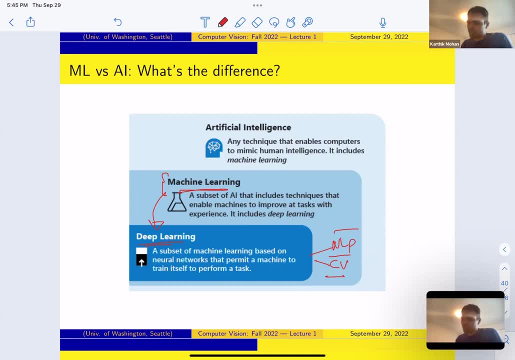 You have to do deep learning for getting good performance in a natural language, also speech, so speech processing, computer vision and NLP. But then there are other things like anomaly detection and clustering where standard machine learning techniques are good enough. So this is kind of a breakdown of that. 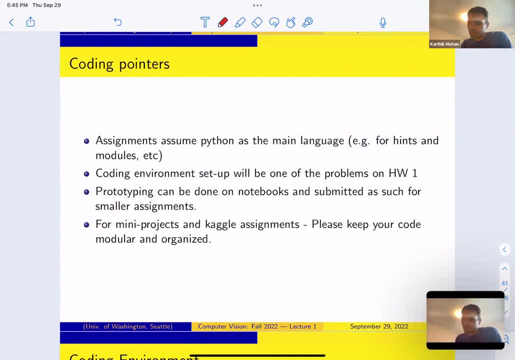 So a few things before we wrap up for today. So your assignment one will be due to the end of the semester. It's due sometime end of next week, But we'll also assign it sometime end of this week, So you have some time to work on it. 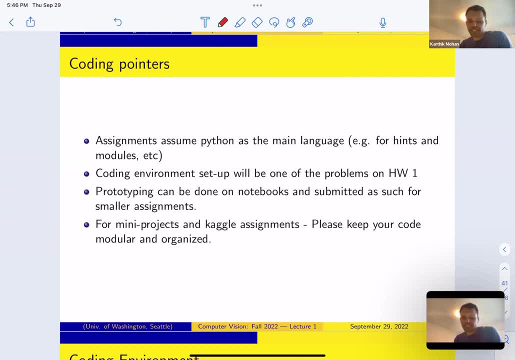 And it's going to be based on basic image processing techniques. We'll cover those in the next lecture, next two lectures. So Python is a main language we'll use And you can prototype in notebooks And you can submit the notebook as such. 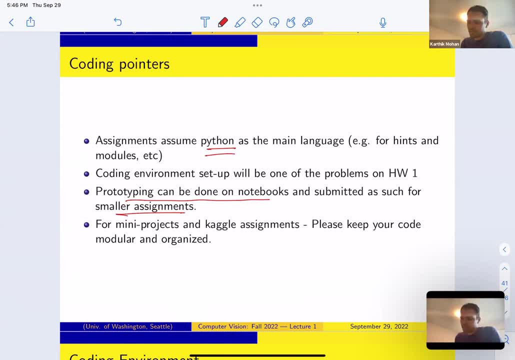 for smaller assignments, For mini projects and Kaggle assignments, we will ask you to keep your code more modular and organized like: use some classes or things like that so as to organize your code like you would actually write code in an interview or in an industry setting. 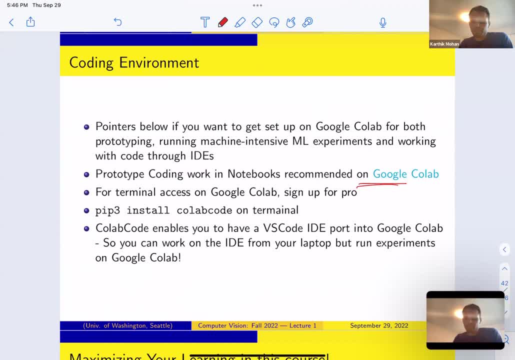 And you can use Google Colab. Highly recommend it because it has a lot of good features, especially when we get to deep learning as well. You can leverage some of the GPU instances that they provide to do deep learning using PyTorch with GPU. 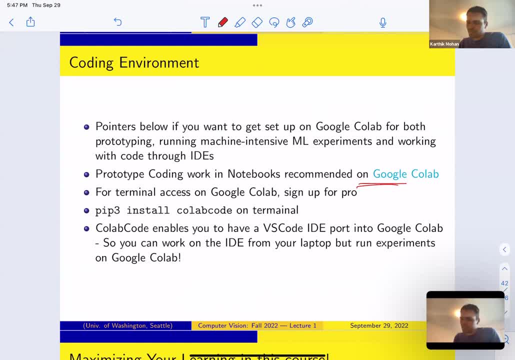 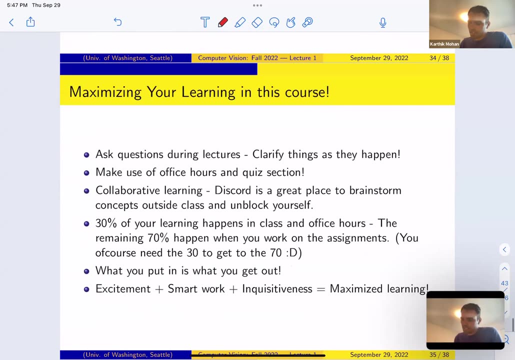 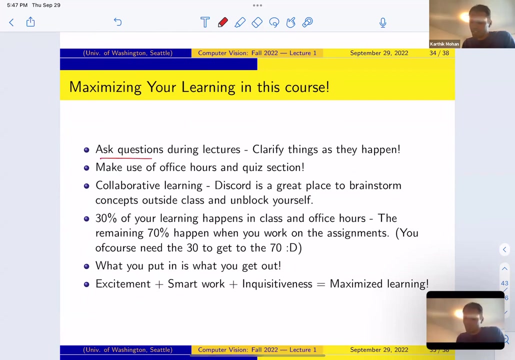 instances. So feel free to set up your Google Colab for your first assignment as well, so that you can start working on it going forward. Yeah, a couple of things on just maximizing your learning in this course. Feel free to ask questions and clarify things as they happen. 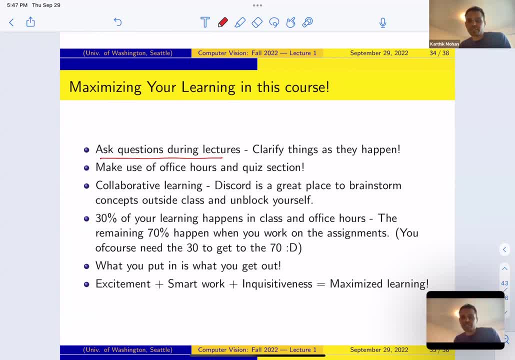 Like you might think: oh, I have this question but I don't know if it's relevant or if it's intelligent or anything like that. Just, I'm very sure someone else might have the same question, So just ask it anyway and we can clarify it. 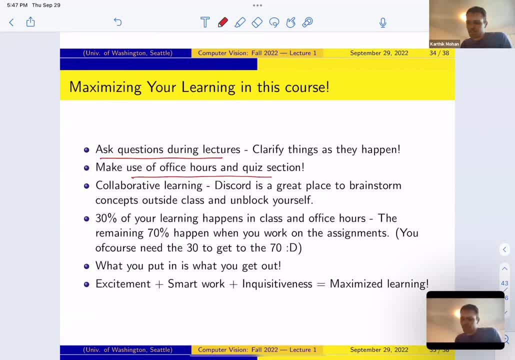 and we can keep moving on. Make use of the office hours and quiz section that we have. So we'll discuss this. We have a couple of office hours and quiz section for this course And use the office hours. Use Discord. So if you're not already on Discord, get yourself set up. 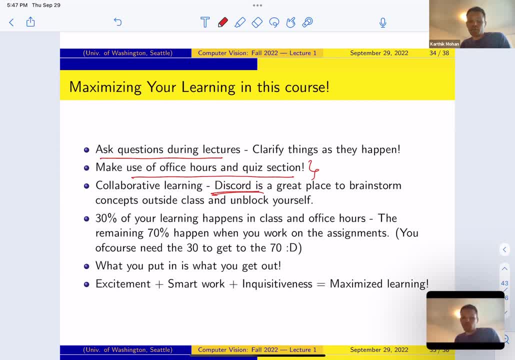 It's a great place to brainstorm concepts outside class and unblock yourself. share ideas, share resources, share materials, share thoughts so you can collaborate and brainstorm, And even for the assignments, you want to discuss some parts of the assignment, like not handing out the solution. 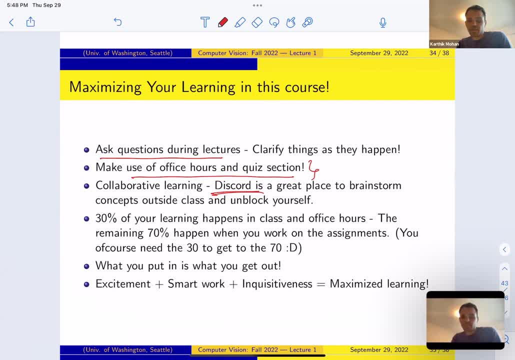 like: hey, here's a solution, but more of like: let's think about what methods might apply here And you want to share some thoughts or get someone to pick someone's brain? Just share that on collab right, Make it collaborative. 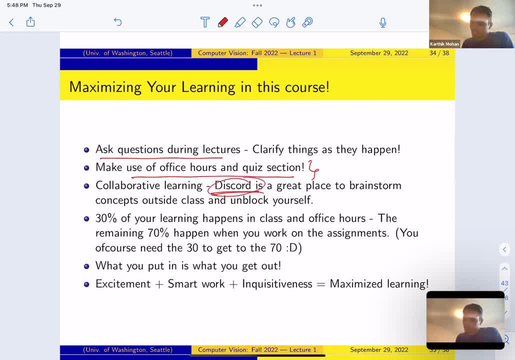 Not collab, sorry Discord. Like I said earlier, 30% of your learning happens in this class and office hours. 70% happens when you work on assignments. So we will be placing a lot of emphasis on assignments And this goes without saying what you put in. 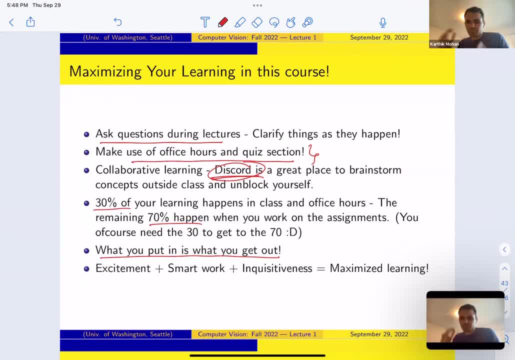 is what you get out. So if you want to maximize your time, maximize your learning, I would say: bring in your excitement, ask questions in class, do your assignments and work a little bit smart. Like it's not hard work, I would say it's more of smart work and optimizing your time. 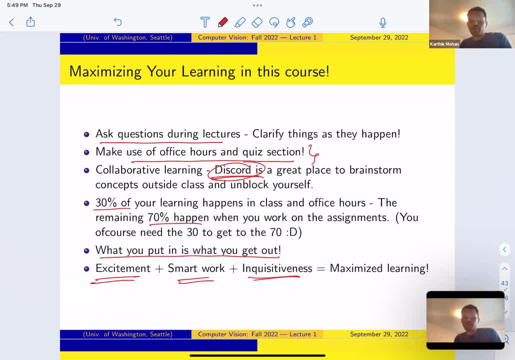 so that, like, OK, I can struggle on some problem on my own for four hours, or I can just post on Discord. So that's a smart thing to do, So not waiting to figure everything out yourself, because sometimes it's easier to collaborate. 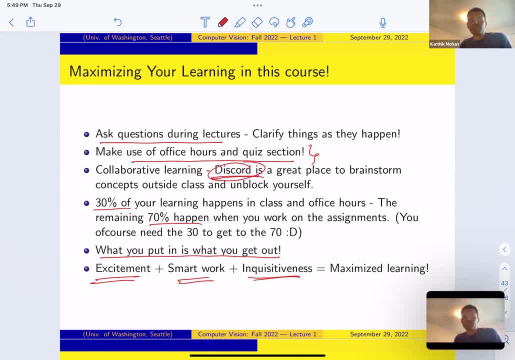 Or You know, just if you're working on a Kaggle contest, breaking things down and working on the critical pieces before you work on the other pieces. So that's again a smart way of doing things. So if you can organize your work schedule, 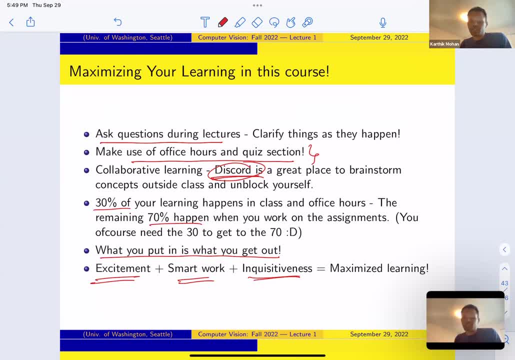 you can get a lot of things done in a little bit of time, a little less time. So then you'll get a lot out of this course. We found in previous courses that we have taught people have found the things that we've discussed in class actually being asked in interviews. 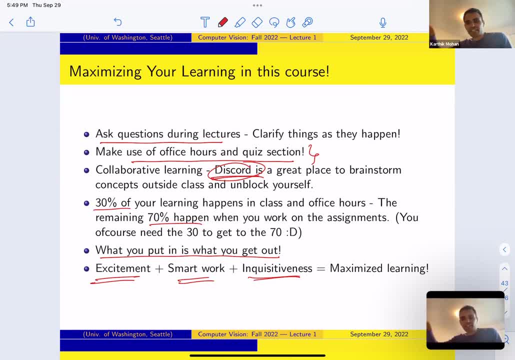 And they were like: oh, we discussed that in class and we actually got that as an interview question And thank you, and I got a job. So that's why I'm saying: just stay active and you'll get a lot out of this class. 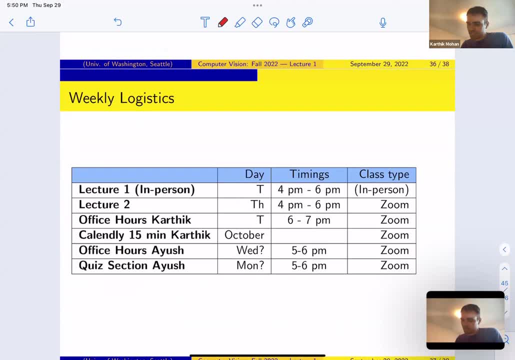 Office hours. I think we did a survey on this. I'm just posting some of the main times that work And maybe, Ayush, you can also clarify what works for you for office hours or quiz section. So lecture one. sorry, this is off. 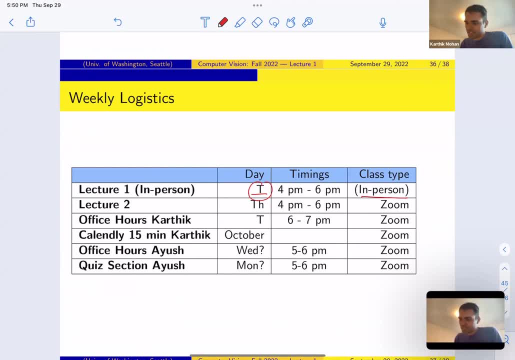 The first lecture every week is on Tuesday. It's in person and it's 4 to 6.. The second lecture- like today is like a second lecture- is on Thursday, 4 to 6.. It'll be on Zoom. 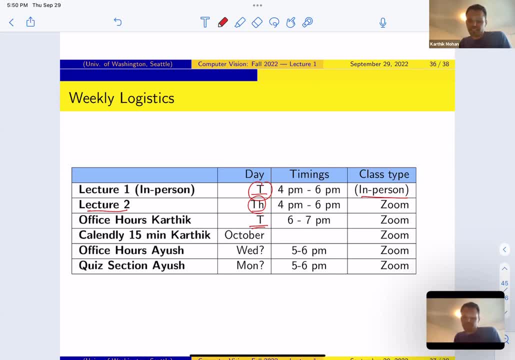 So my office hours, based on the survey, Tuesday seems to work best for most people, So we'll have it 6 to 7 PM, Right after class, And so it'll be in person. right, So I'll be in person so we can discuss it at the building. 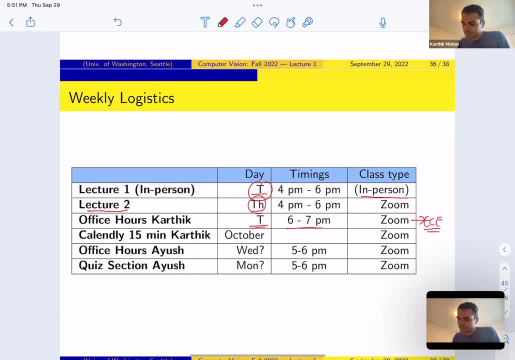 So we'll be mostly in one of the ECE buildings, ECE rooms. I tentatively put Wednesday and Monday for office hours of Ayush. I think we'll also have grading hours. We'll let Fatweer talk about this sometime today or maybe. 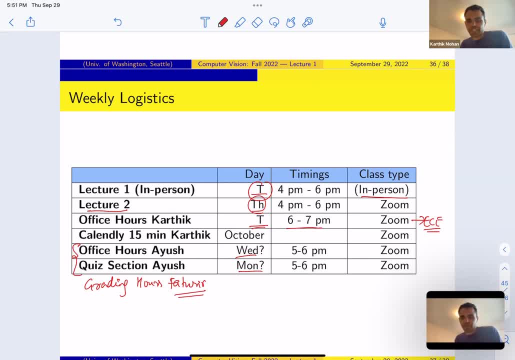 the next lecture Just to discuss any questions you might have on grading. So you can go to the grading hours. This might happen once every two weeks So you can get your grading questions resolved. So, Ayush, if you're around, can you jump in on these two dates? 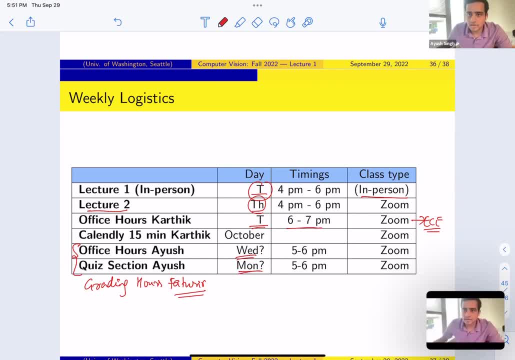 Ayush, sure, actually I'll just have a look at my own schedule and then let everyone know through Discord. the final office hour and quiz section timings: Okay, sounds good. So this is kind of the rough thing. So you have all of these resources: lectures, office hours.